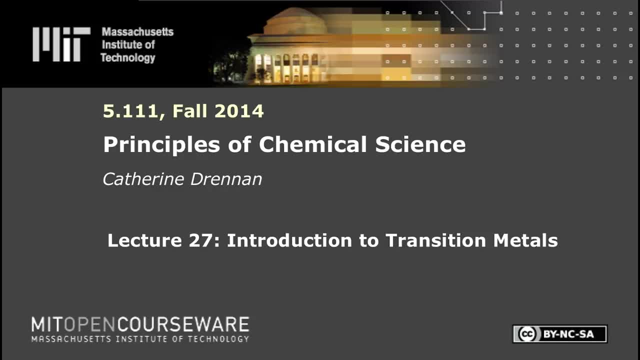 The following content is provided under a Creative Commons license. Your support will help MIT OpenCourseWare continue to offer high-quality educational resources for free. To make a donation or to view additional materials from hundreds of MIT courses, visit MIT OpenCourseWare at ocwmitedu. 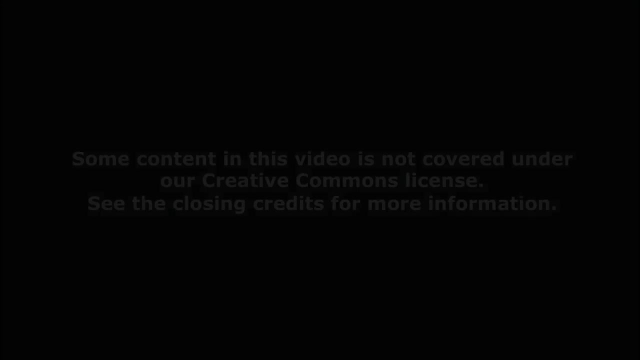 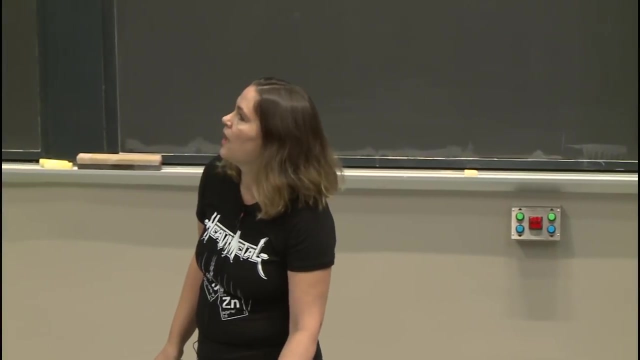 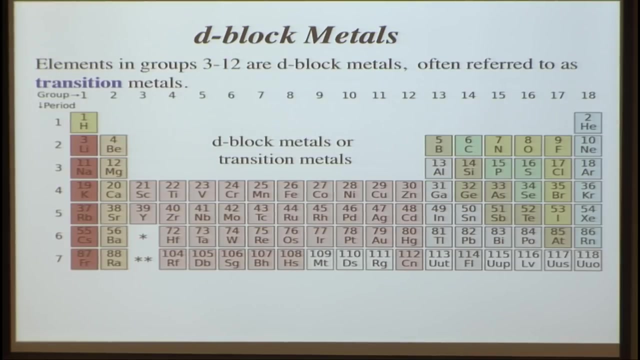 All right. so moving to today's handout, this is one of my favorite parts of the course. Honestly, when I first started teaching 5.11.1, I said transition metals are rarely covered in intro chemistry courses. Is it really necessary to cover it here? 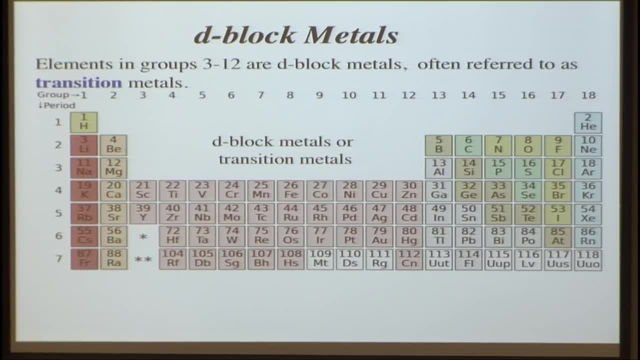 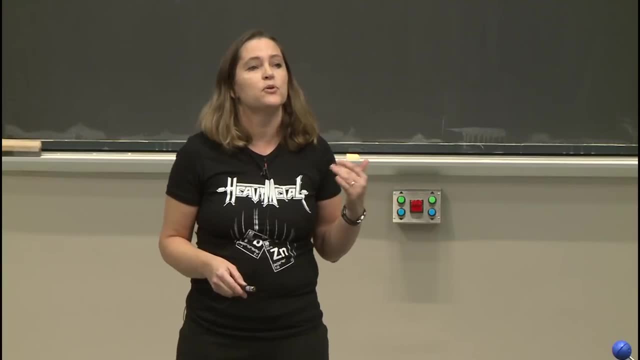 And I was told it absolutely was. It's one of the reasons that a 5 on the AP exam is not good enough, that you have to take the advanced standing exam, because the people who teach inorganic chemistry found that people who placed out of 5.11.1. 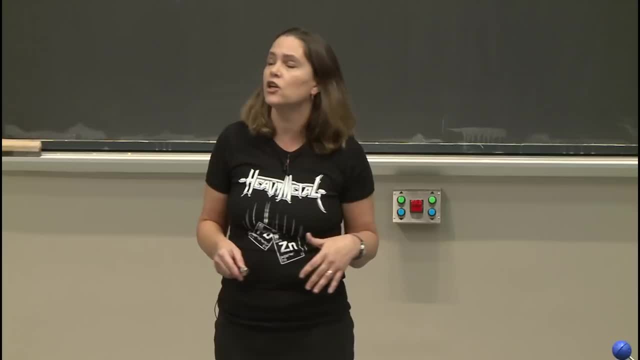 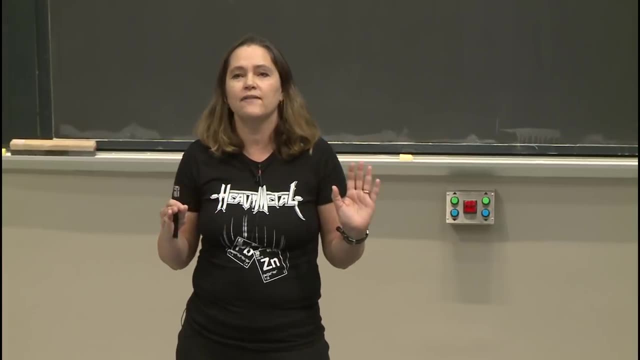 didn't do as well in their course as people who took 5.11.1 here. So this is one of the reasons. And then I started teaching it and I realized this is one of the, even though people haven't seen it before. 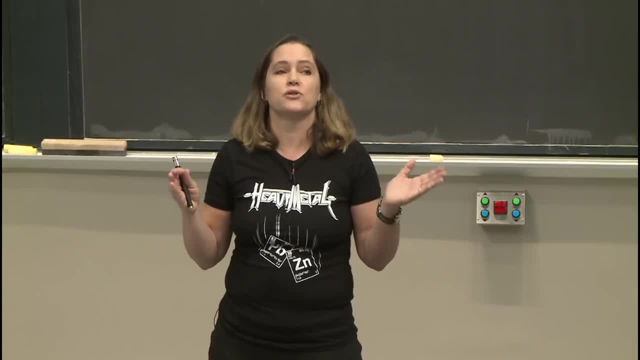 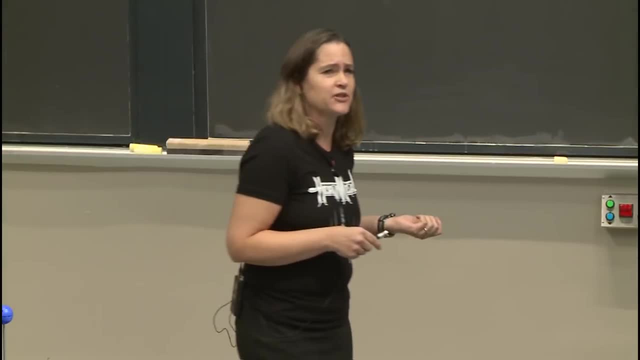 and sometimes people get a little scared. it's actually one of the most fun units, So I absolutely love it And hopefully you will love it by the end. People are like we never covered it. Why are you covering it? We're in chapter 16.. 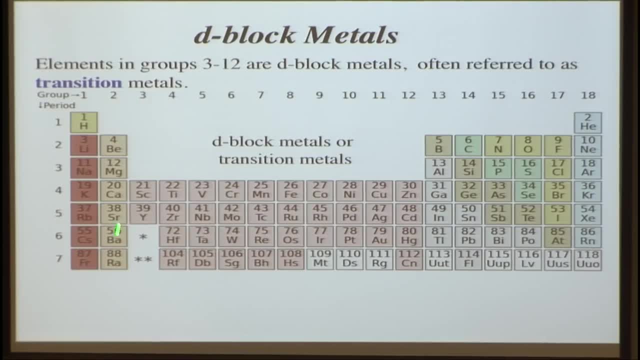 It's fun. So transition metals, d-block metals, because they have those d orbitals. Yes, we're going back to talking about orbitals again And they're called transition metals because you transition from this part of the periodic table with your. what kind of orbitals? 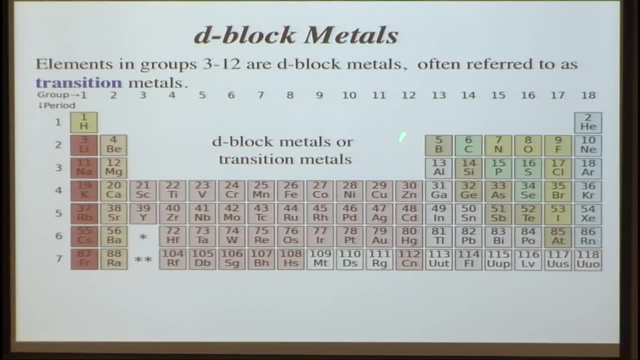 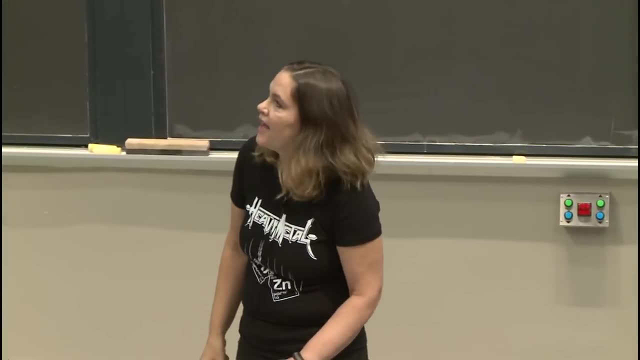 S to this part of your periodic table with your. what kind of orbitals P? So they are the transition metals And they're often really reactive and very cool And many of them- since we're on a biological theme- many of them are super important in biology. 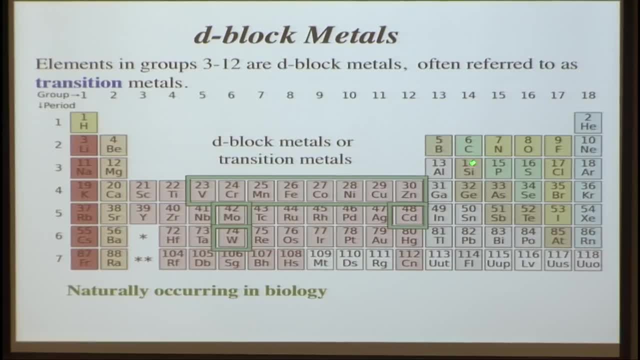 And I have some of these written down in your notes, but here they are. Up. here. in the transition metals you have a lot of metals that we could not live without. Iron carries oxygen to our blood, very important Hemoglobin. We talked about cobalt. 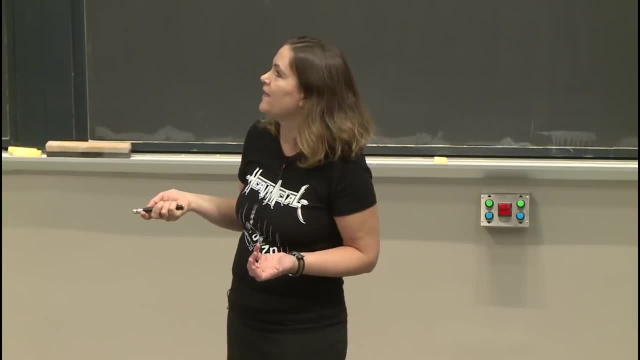 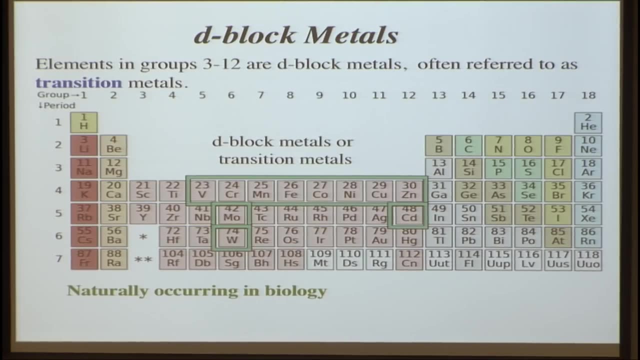 Just now. that is the metal in vitamin B12.. So we know why that's important. We have zinc everywhere. Nickel is important for bacteria- Not so much for us, but bacteria is important for us. So therefore, nickel is important to us. 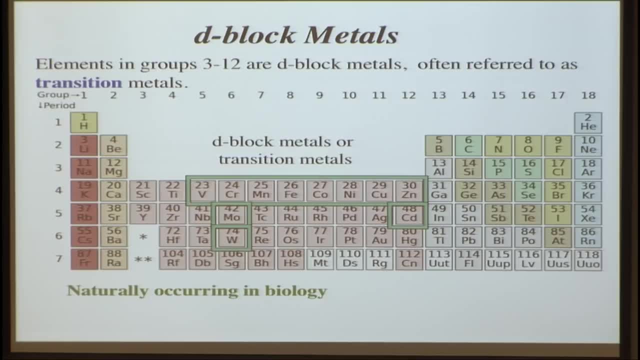 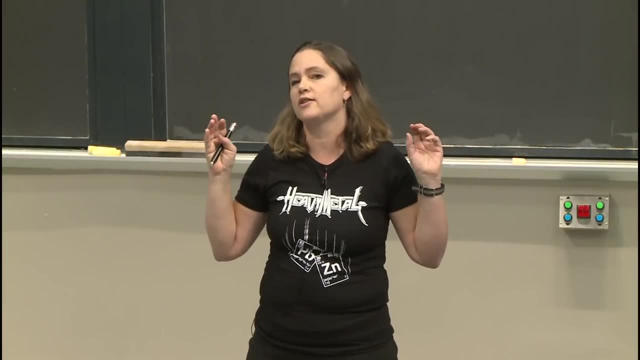 So all of these are really important. Also, this part of the periodic table is part of the table that people love, that want to make pharmaceuticals or want to make new kinds of electrodes or batteries or all sorts of things. There's a bunch that are important. 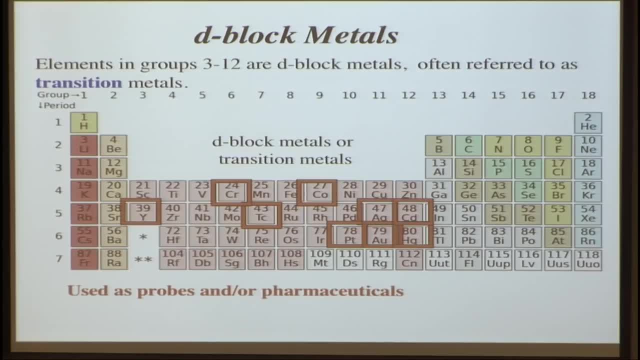 There's a bunch that are used as probes. We talked about imaging agents, detecting cancer and all sorts of different things like that. Many of these transition metals are used in those probes and also in pharmaceuticals, And so this is sort of a very rich part. 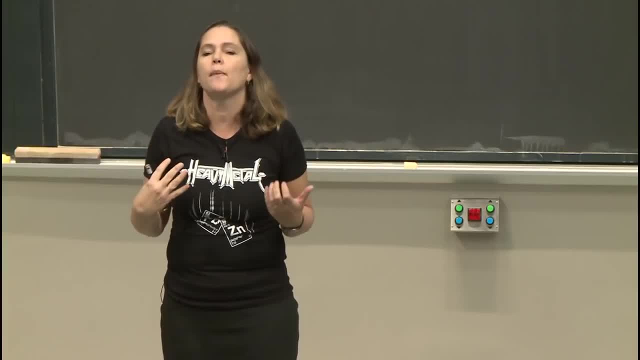 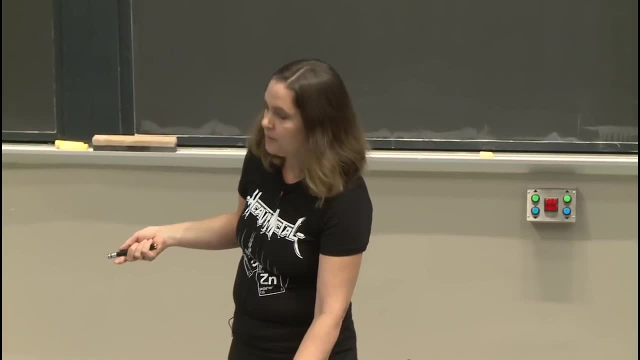 of the periodic table, where those d orbitals allow for properties that are incredibly useful for our health and for doing all sorts of stuff. So I love this part. Again, Some of the biological global cycling of nitrogen. We talked about nitrogen fixation, that triple bond. 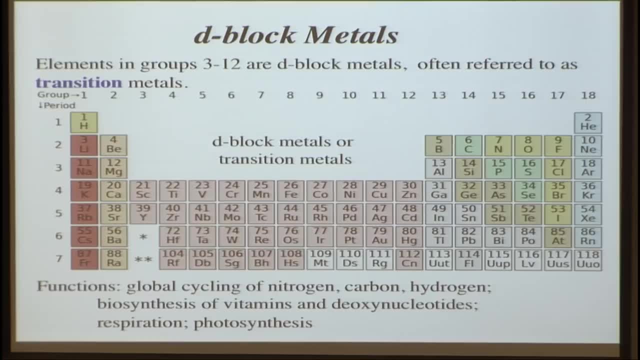 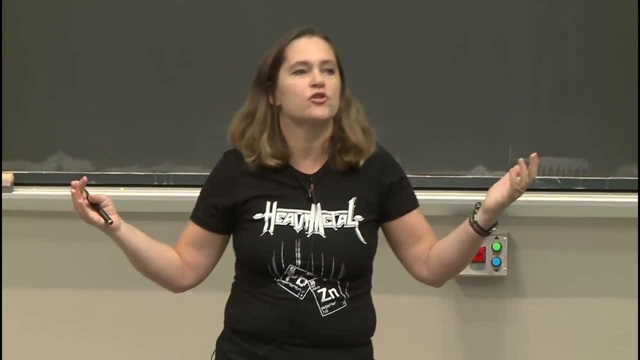 It's really hard to break nitrogen apart, But bacteria can do it. It does it using transition metals Fixing carbon Hydrogenase. People want to make hydrogen fuel cells that are more biological. Again, biology uses transition metals in this. 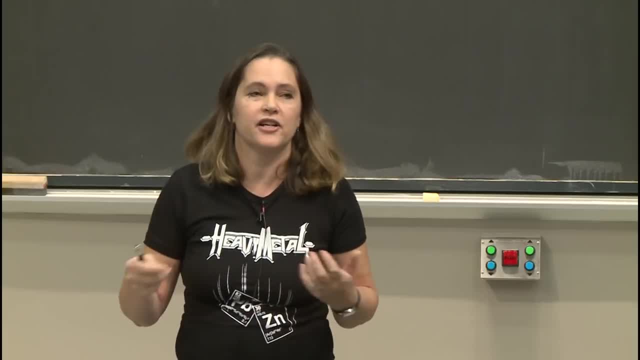 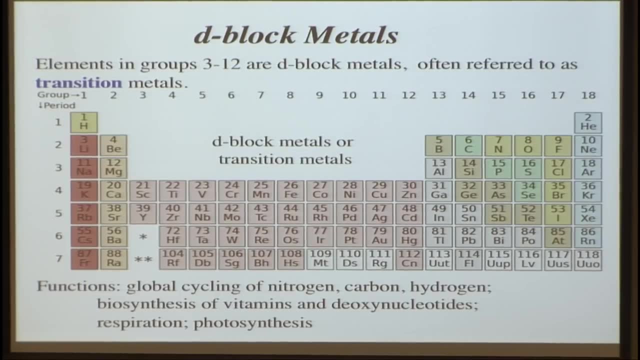 Making vitamins, making deoxynucleotides, respiration, photosynthesis- It's all due to transition metals. All right, We will start with just one example, or one of our, in our own words, segment, And this focuses on nickel, which. 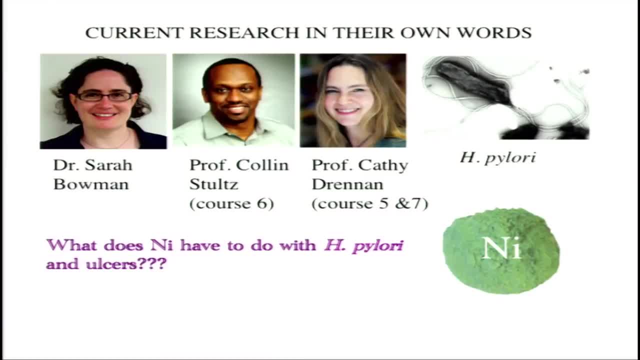 is something very important in bacteria, And this is actually an example from a collaborative project between my lab and course six, And I know a lot of you are thinking about being course six majors, So I thought I would tell you about some research of Colin Stultz, a course six professor. 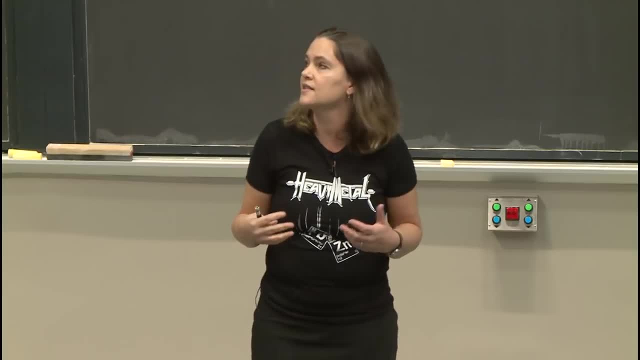 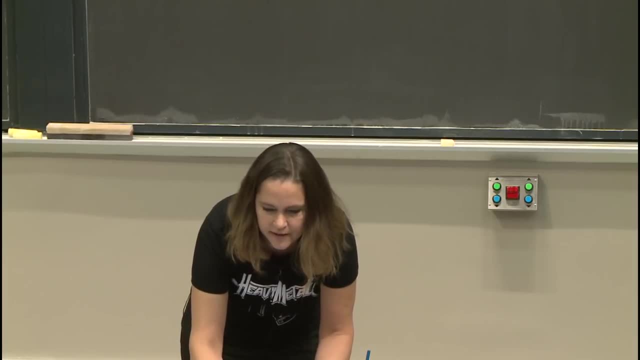 So he was doing some computational analysis on these proteins that we're studying. Many of you at this point in the semester probably feel like you might be getting an ulcer, But unless you have H pylori in your gut you probably are not actually getting an ulcer. 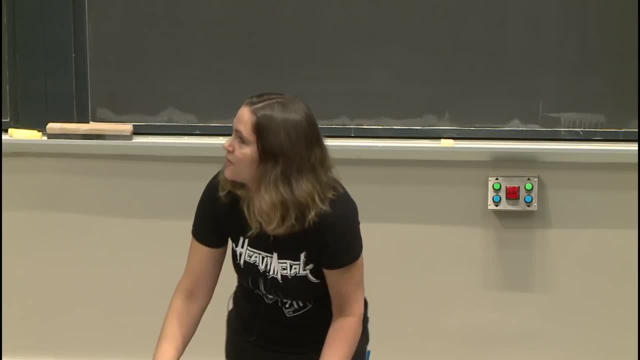 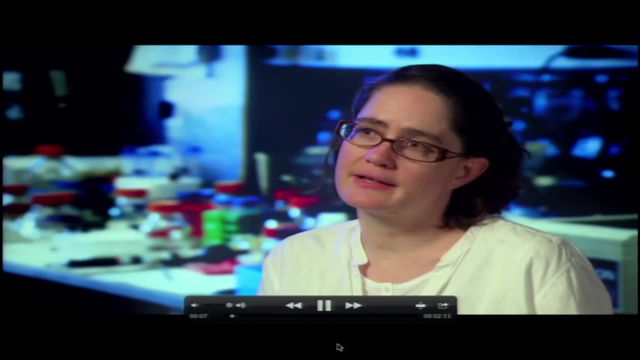 And you just take a little B12, you'll feel a lot better. OK, So here's the video. My name is Sarah Bowman And I am a postdoctoral fellow at MIT. I am working on studying a protein from Helicobacter pylori, which is pathogenic bacteria. 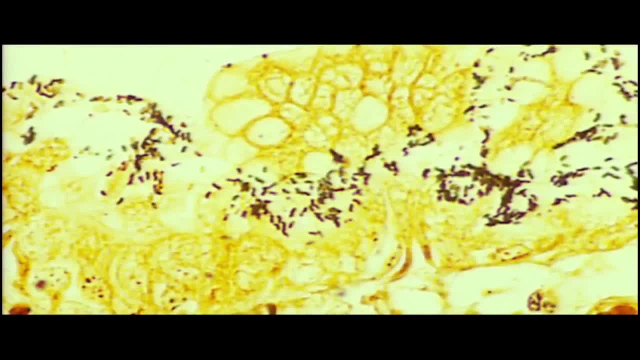 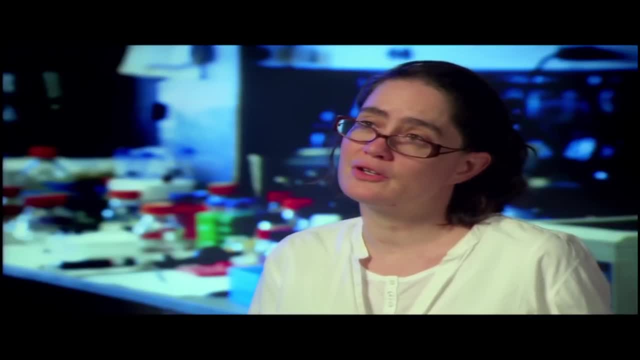 Its kind of ecological niche is in mammalian stomachs. It's actually very difficult to treat using antibiotics Because a lot of times when you're given antibiotics they're going to actually be broken apart by the acidity of the stomach before they actually ever. 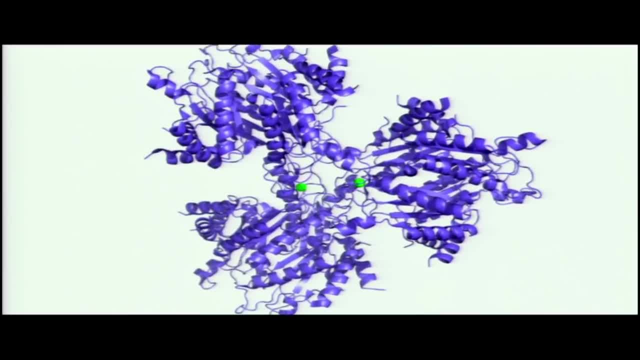 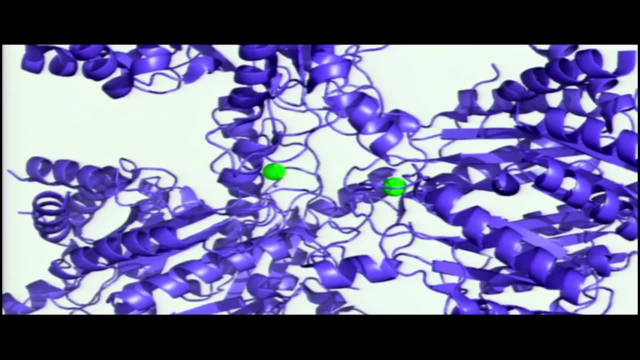 get to killing the Helicobacter pylori. Transition metals in biological systems are actually really important. They increase the range of reactivity that proteins and enzymes are able to access. Nickel is a transition metal And it's a very, very important ingredient. 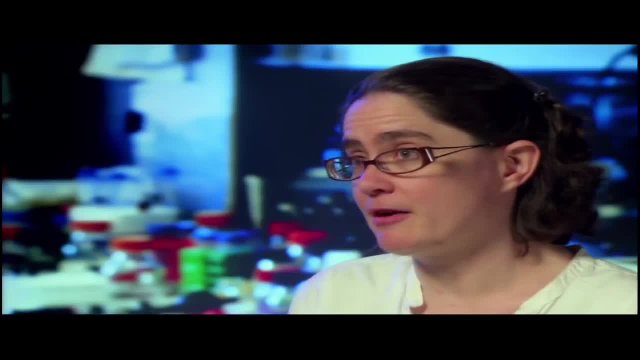 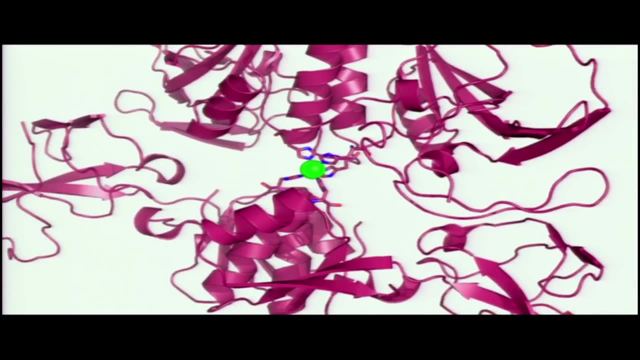 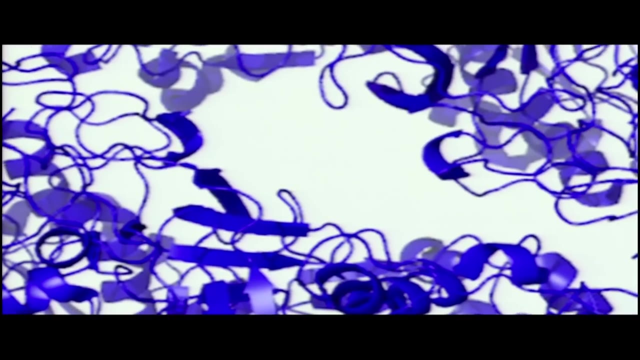 I mean, it's a transition metal that's actually fairly rare in biological systems. So one of the big things that H pylori uses nickel for is an enzyme called urease. Urease requires something like 24 nickel ions, which is a lot. Urease is one of the proteins that allows for a lot of buffering capacity of the organism, of the H pylori organism. The stomach pH is very low, so pH 2 something, And this bacteria has to swim through the stomach and then colonize it. 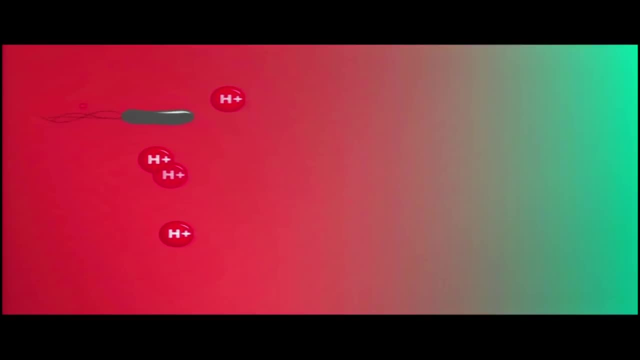 And you'd think that the stomach would just break it apart, like it breaks apart your food, But in fact the bacteria itself has mechanisms in place that allow it to create buffers, that allow it to move through the stomach and live in the stomach, And one of those enzymes that's really important for that. 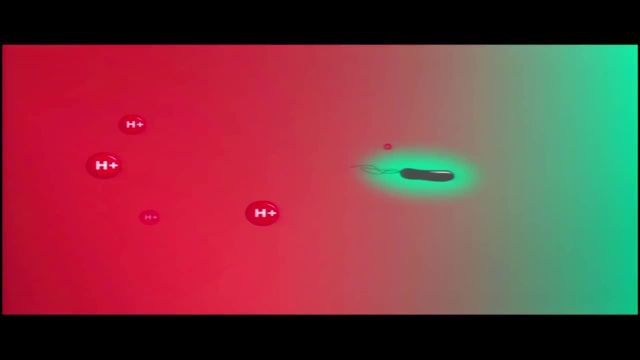 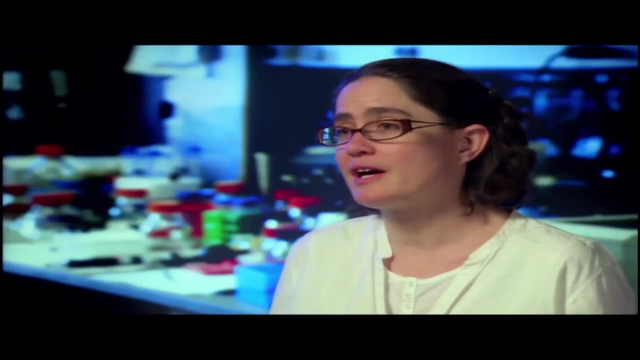 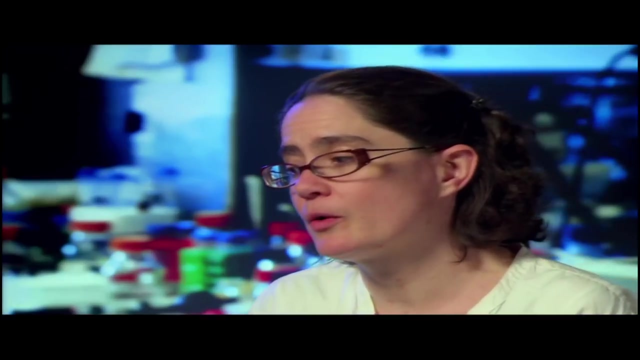 is urease. In humans, nickel, as far as we can tell, is not essential for any enzymes, Whereas in Helicobacter pylori, for instance, nickel is an essential transition metal, And so a really intriguing thing to kind of think about. 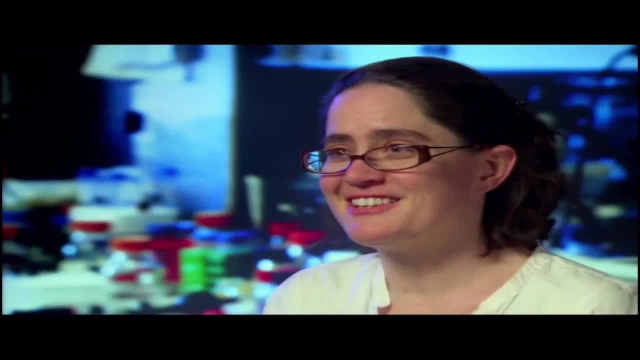 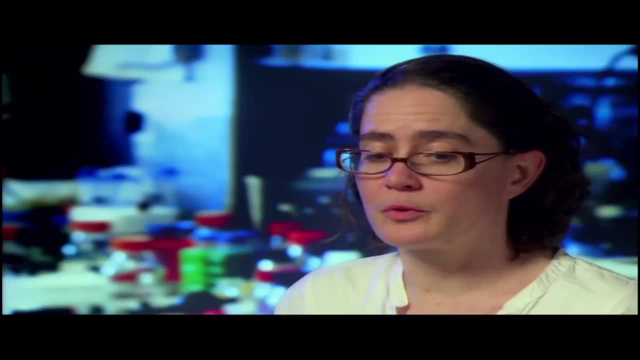 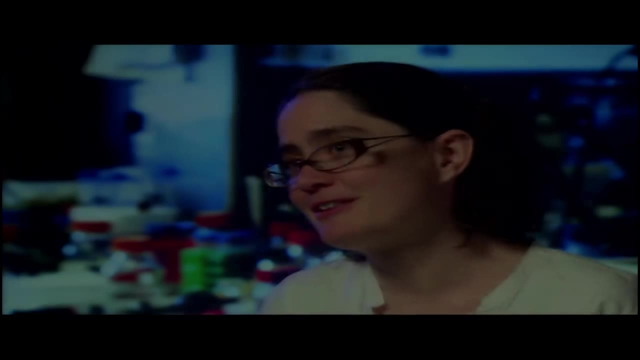 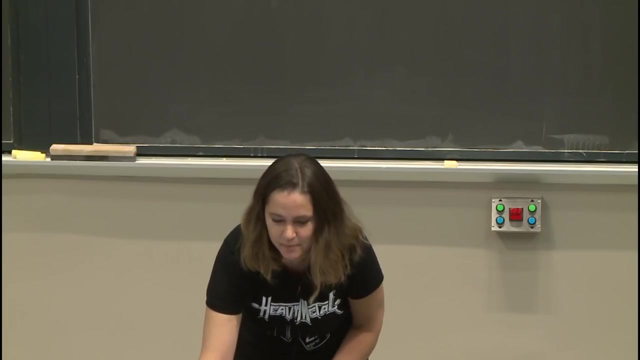 is just whether we could somehow target the nickel requirement in this organism and in other bacteria. That would allow us to kill these pathogenic bacteria while not doing anything that would be harmful to humans. So I like that video, partly because it brings back acid base and buffers as well as talking. 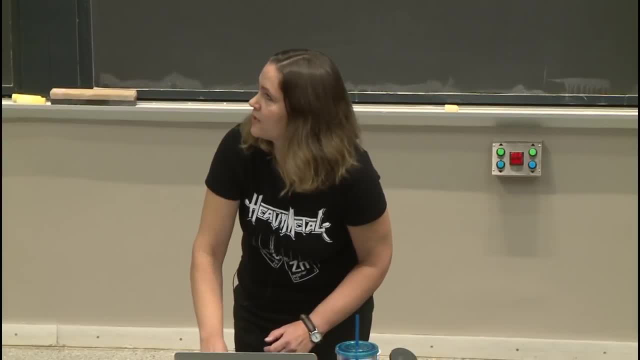 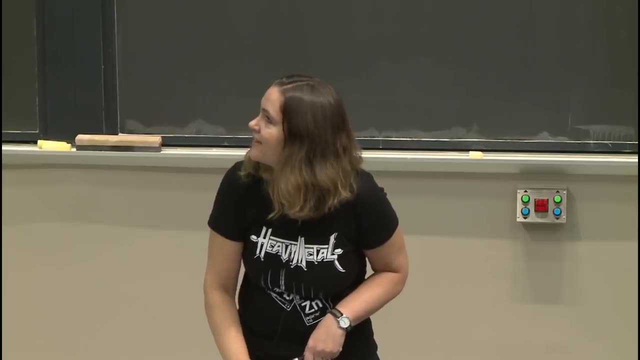 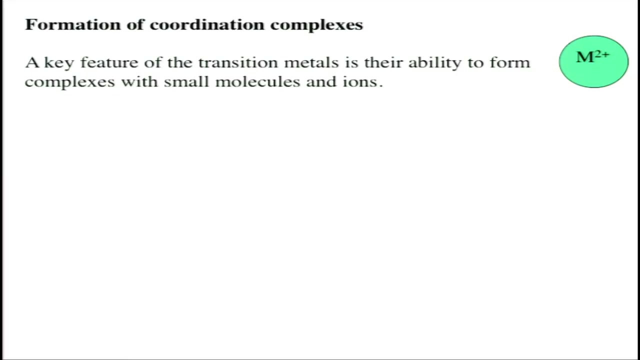 about transition metals And I love the bacteria being attacked by the acid and then making a buffer and saving itself. It's awesome. OK, OK, OK, OK, OK. So one of the reasons why these transition metals are so powerful: they can do so many things. 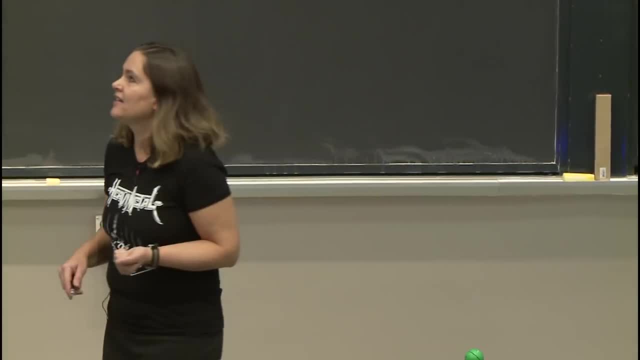 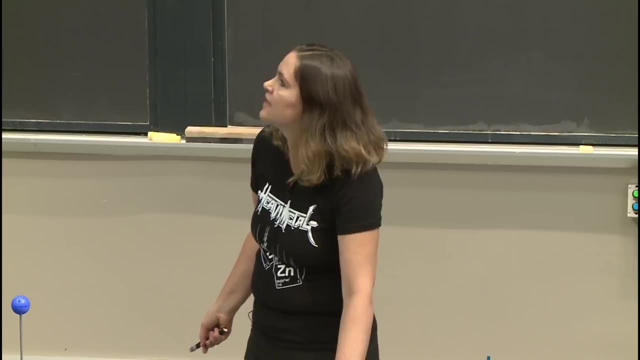 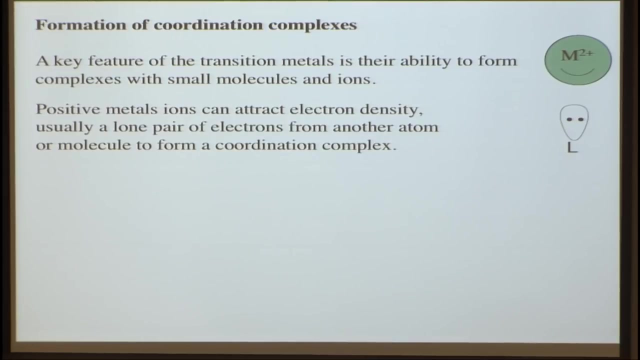 is that they like to form complexes. And they like to form complexes with small molecules or ions, And those ions often will have a lone pair of electrons And the metal wants that electron density, It wants the benefit of that lone pair. So when you have this lone pair, 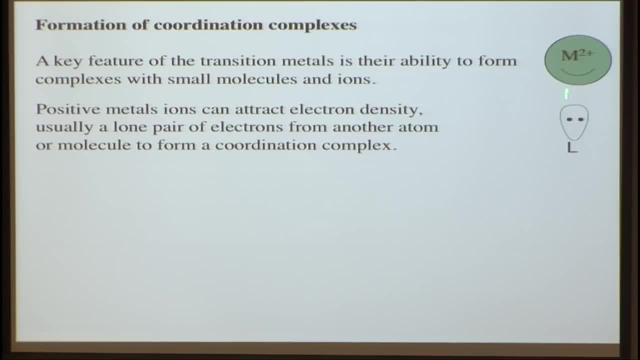 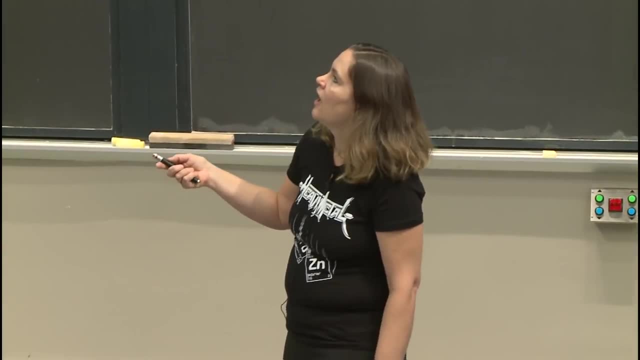 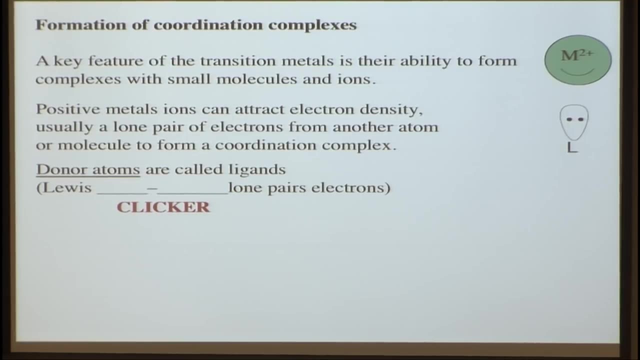 And the metal will come in contact with that lone pair and it will make it very happy, very happy metal. And we can think about this interaction here as the donor atoms are called ligands. And now let's review something we learned before about whether this is a Lewis acid or a Lewis base. then 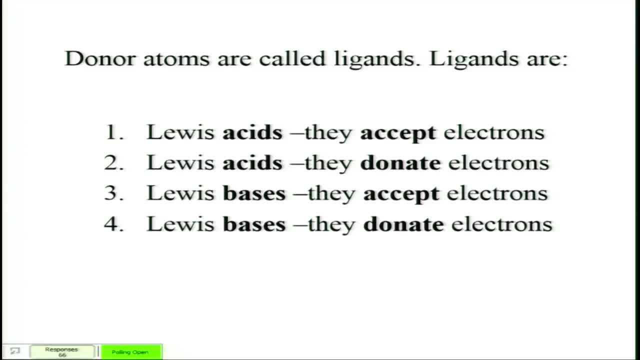 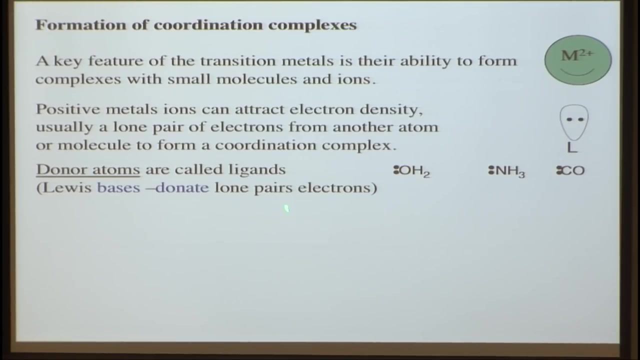 OK, 10 more seconds, That's right. So it's a Lewis base. So if we put this up here, donor atoms are called ligands, which are Lewis bases, And the Lewis bases donate the lone pair of electrons. And again we can think about the definition. 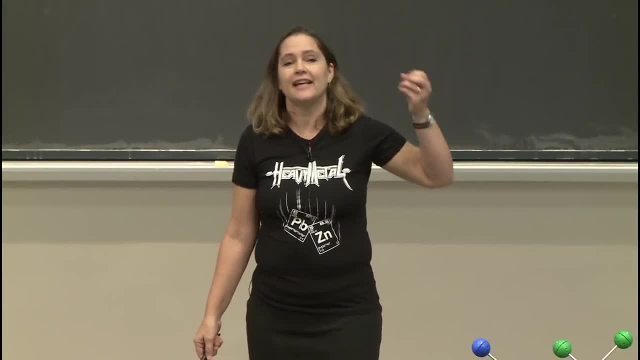 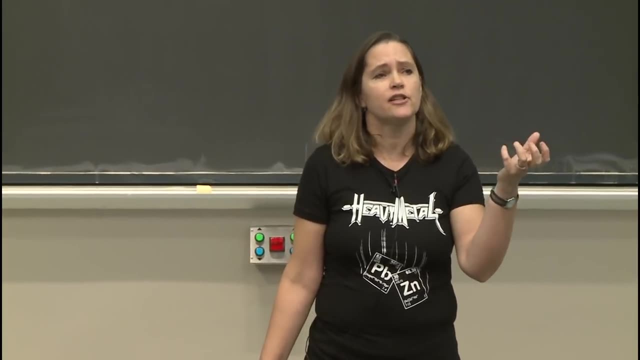 that we've been more used to. where a base is taking H+, It's accepting the proton from the acid, But there, when it's taking H+, it's taking H without its electrons. So it's actually donating its lone pairs to form a bond. 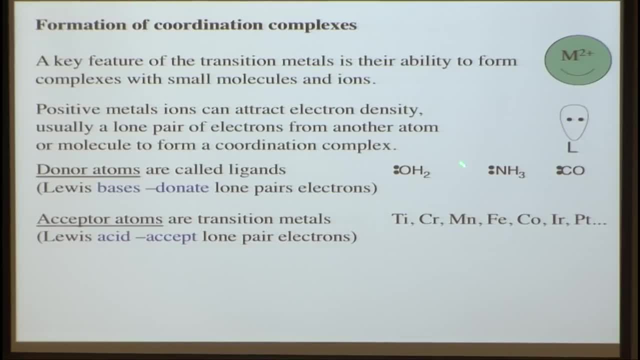 And then we can think about Lewis acids. So the acceptor atoms, which are our transition metals, are Lewis acids. They accept, They accept the lone pair, And when an acid that has a proton on it loses H+, it is taking the electrons with it. 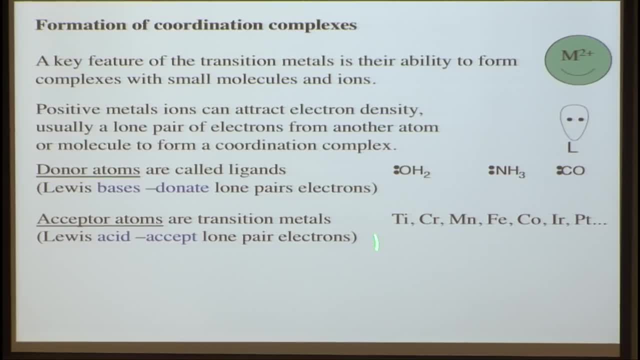 because H plus is leaving without its electrons. So these definitions work, but these are sort of more broad definitions. So here are metals. Any of our transition metals are going to be our acceptors, our Lewis acids, And here are a bunch of ligands. 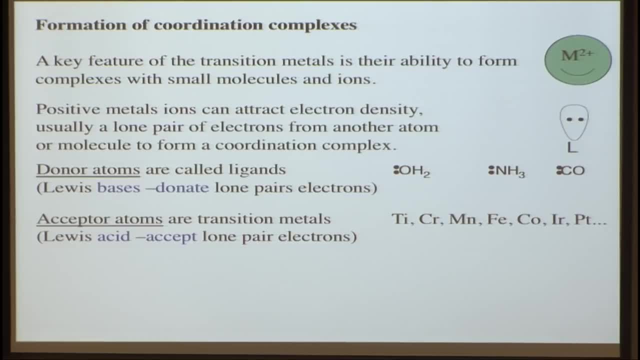 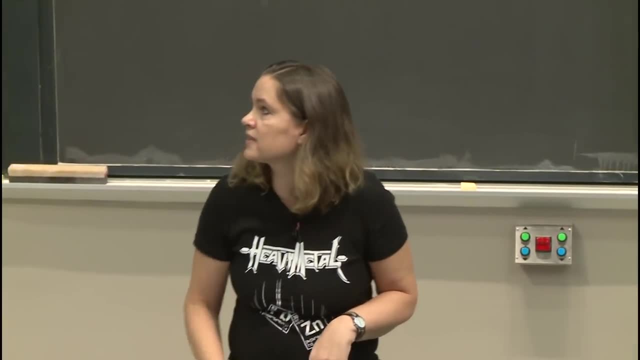 We have water, We have NH3.. We have CO. They have lone pairs, They can be donor atoms And the ligands form a bond. They form complexes with the metals And the kind of complexes they're often called coordination complexes. 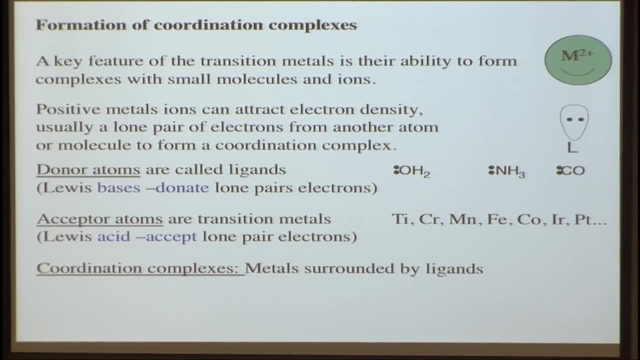 And that's a metal that's surrounded by ligands. And here's a little example: a metal in the middle And it has the ligands around it. So let's consider this coordination complex now and think about what this picture is telling us. 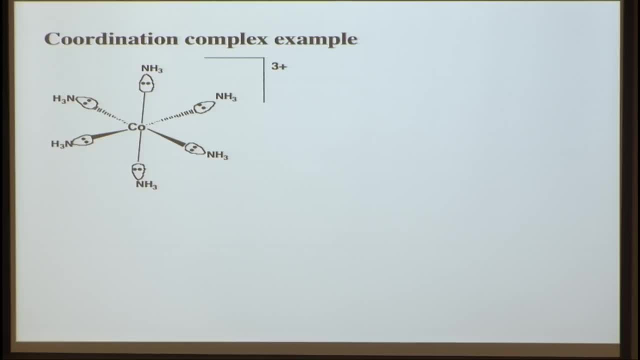 So we have our coordination complex. We have cobalt in the middle And we have NH3. And then we have the ligands around it And if you look at the picture, you can see that each of these three groups is our donor ligands. 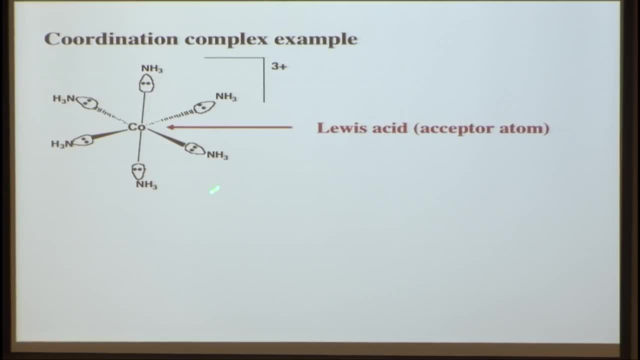 And here this bracket indicates the overall charge is plus 3.. Again, the transition metal is going to be the Lewis acid. It's going to be accepting the lone pairs from the Lewis bases, which are the ligands or the donor atoms. 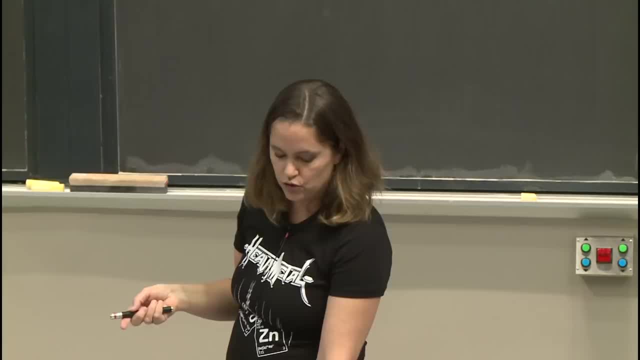 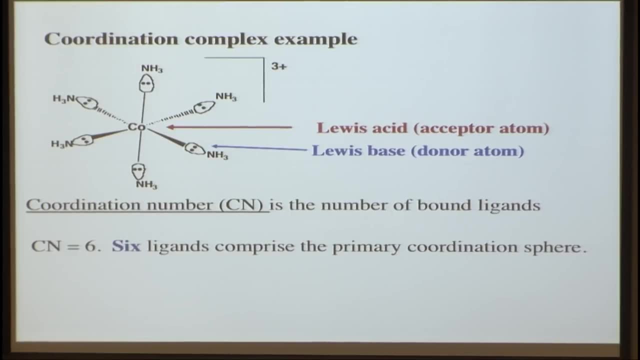 Now we can think about a new term called coordination number. So a CN number of 6 would indicate 6. ligands make up what's called the primary coordination sphere, which is the things that are bound directly to the metal. So CN numbers for transition metals range from 2 to 12,, but 6 is probably the most common. 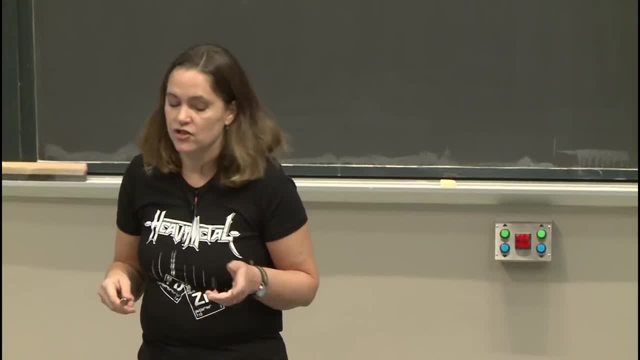 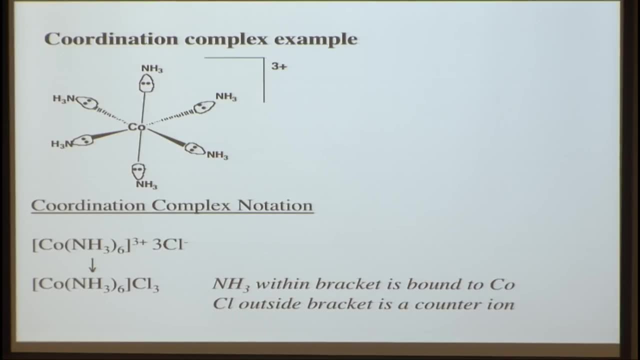 So before we think about the shapes of these molecules, let's just look at the notation for this. So coordination, complex notation. So I would write this structure up here within brackets: cobalt bracket, NH3, you have parentheses around NH3. There are six of those. 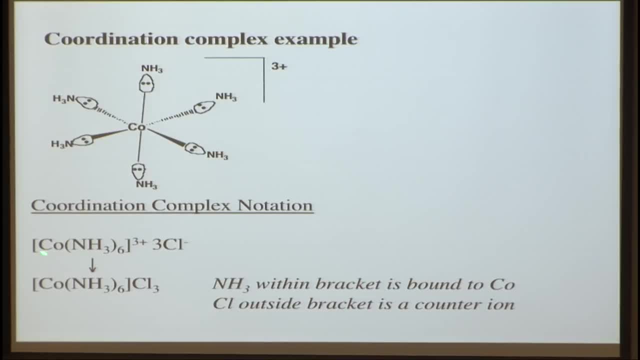 Another bracket here with a plus 3 charge indicating the charge on everything. this way, This whole structure- But often coordination complexes with a plus charge will have counter ions around, So there might be, say, 3 chlorine minus ions around, And so that could be written like this. or it could be written like this: 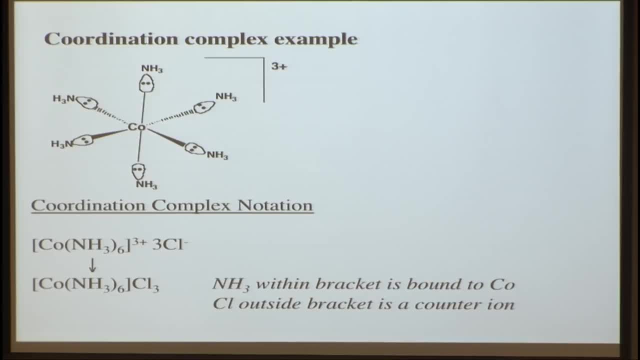 If you see Cl3 outside of those brackets, it means that there are counter ions. So if I looked at this, I'd say NH3 is within the brackets. That means it's bound to the cobalt. So that would tell you there are six things bound to the cobalt. 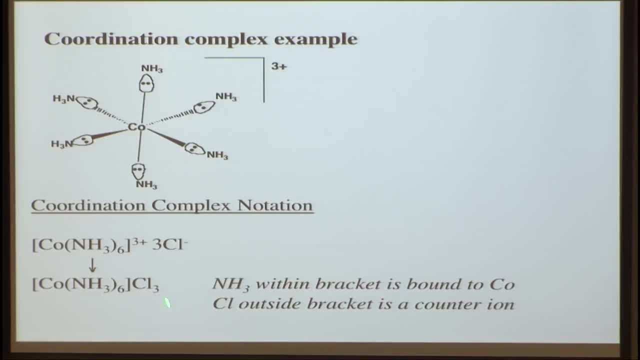 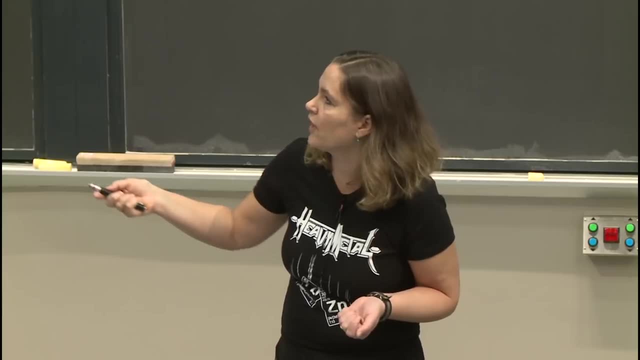 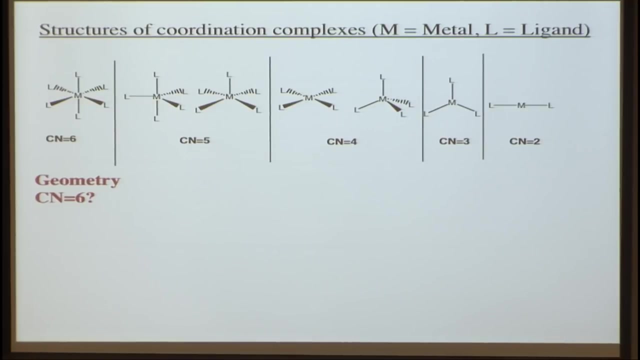 The Cl is outside, That indicates it's a counter ion. There are three of them. So there are three counter ions, which then tells you the charge must be plus 3.. So there is our notation. So now we're back to thinking about geometries. 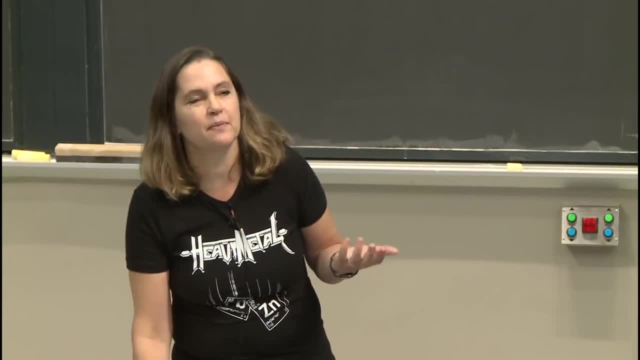 So this is one of the things I love about this part. I feel like some people in the course are just like: new topic, new topic. Oh man, when is the new material going to end? But you find you get enough indications. 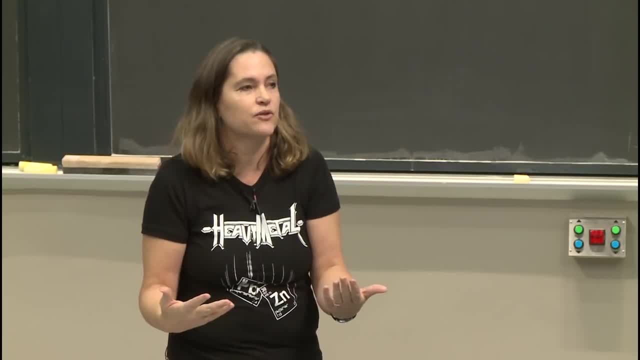 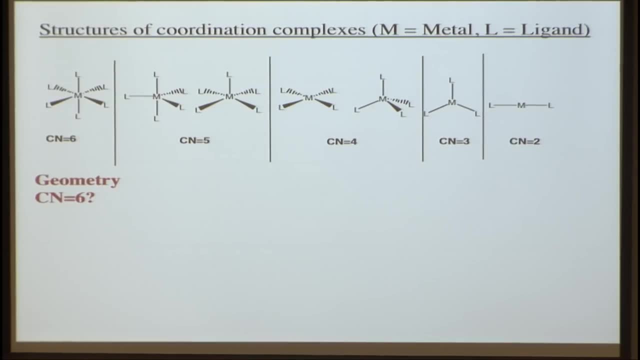 So you go into chemistry and you start revisiting topics you've already seen before. So this is great, All right. so coordination number six. We haven't maybe heard coordination number six, but that's pretty easy to remember. It's the number of atoms bound. 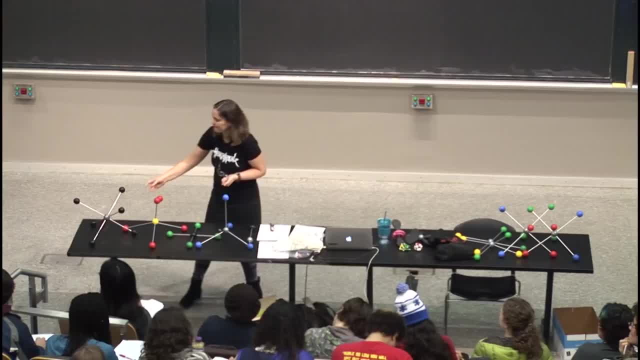 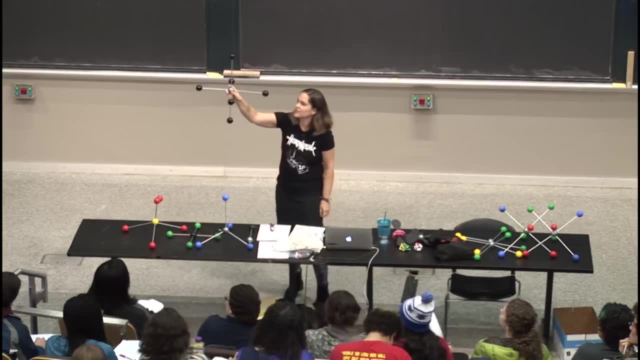 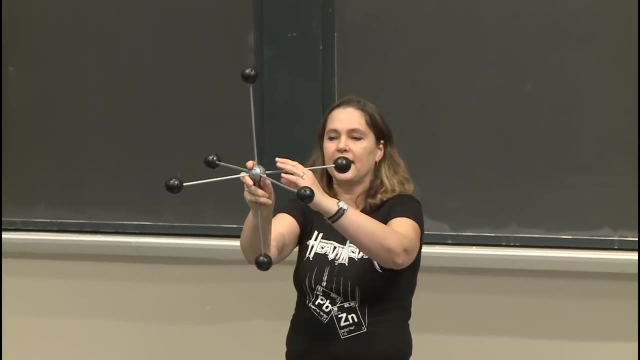 What type of geometry is this? You can just yell it out, All right, so that's octahedral geometry. Again, Again, the solid triangles coming out indicate they're coming out at you. Back dashes are going back and we have our axial. 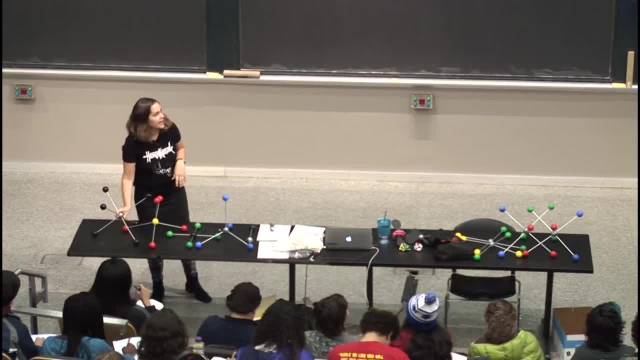 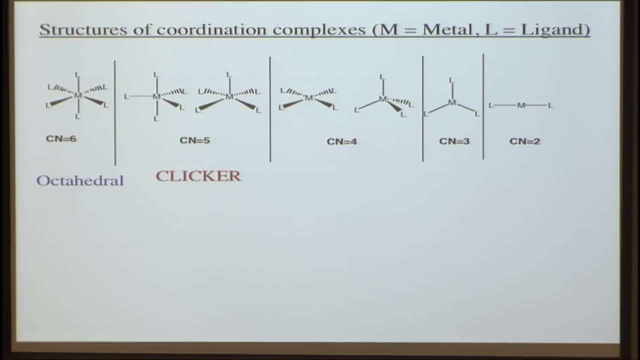 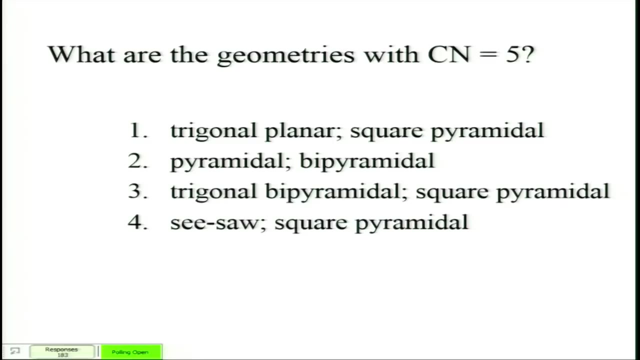 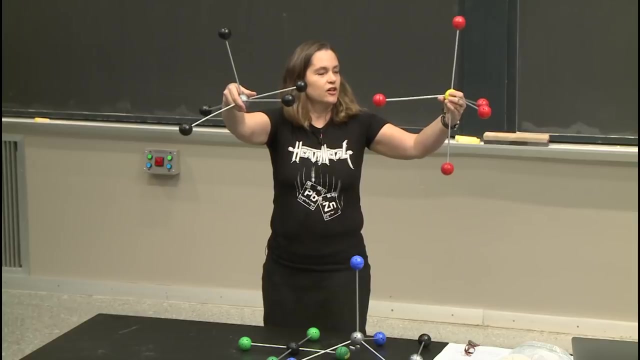 All right, so let's see how well you remember CN5 structures And you can keep this up here and you can tell me what the name of those two geometries are. All right, let's take 10 more seconds and here are our structures in real life down. 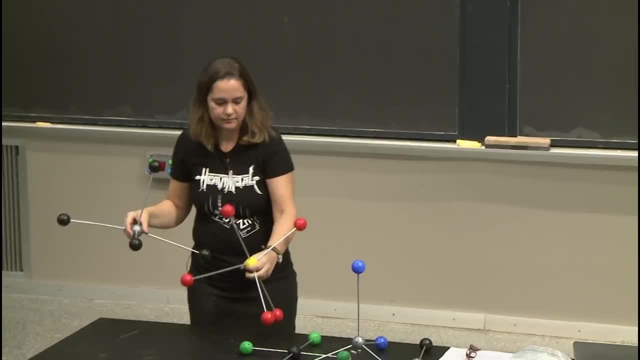 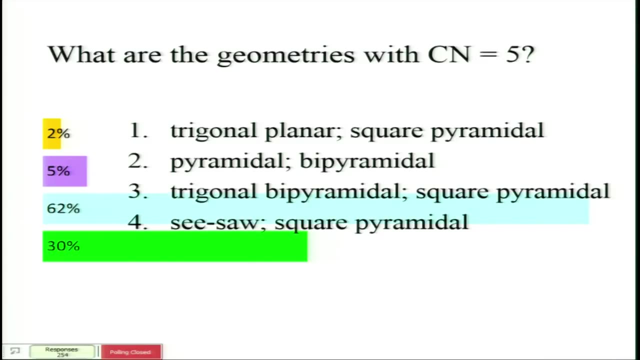 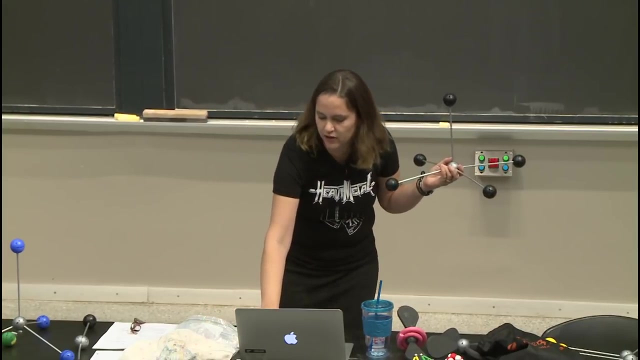 here People are just like I want to put seesaws. No, No, That is a parent geometry of seesaw, but not seesaw itself. OK, so we have the trigonal bipyramidal and the square pyramidal. 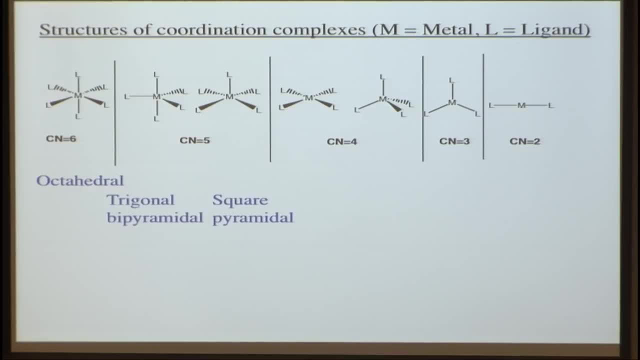 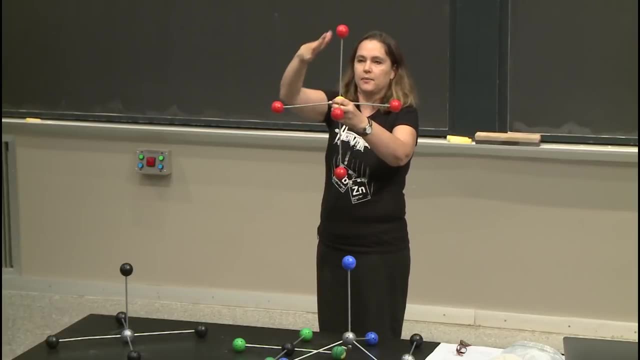 So I'm holding up the square pyramidal right now, And then we have the trigonal, Because it's trigonal along here, bipyramidal. So it's sort of like one pyramid here, one pyramid there, So bipyramidal. 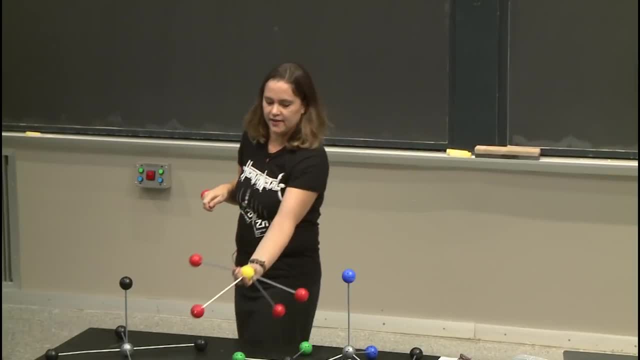 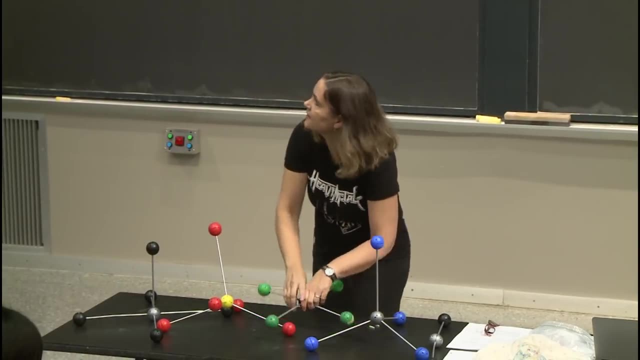 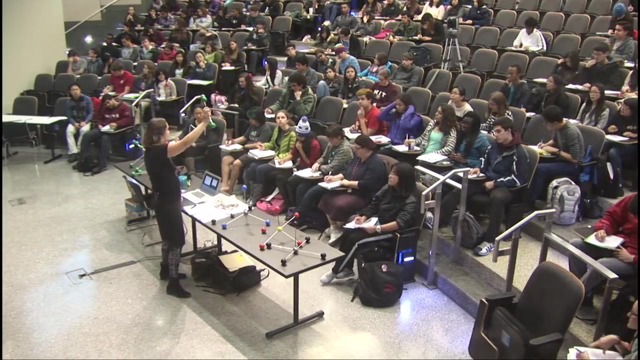 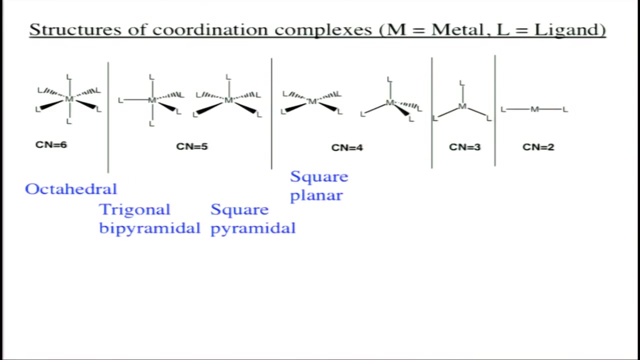 And if I took off one and we had a lone pair, then we would get our friend the seesaw. OK. Next we have this: What's that one called Square planar? Yep, And this one Tetrahedral. 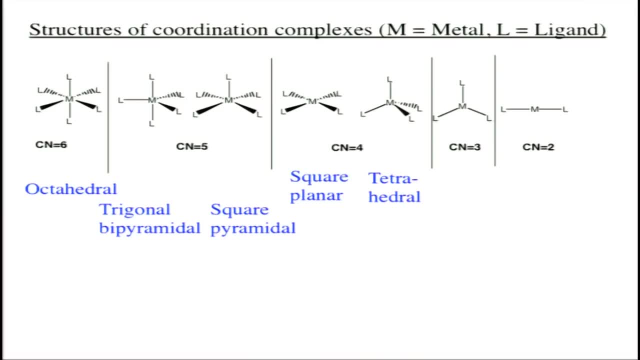 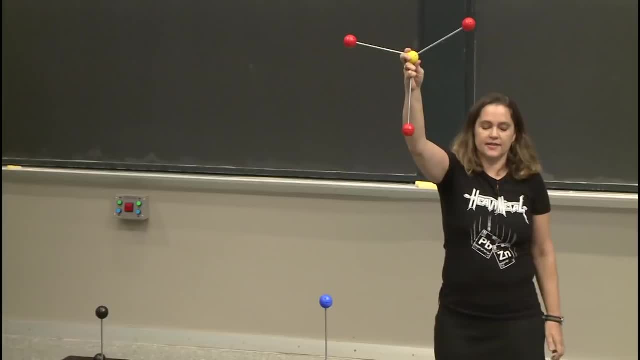 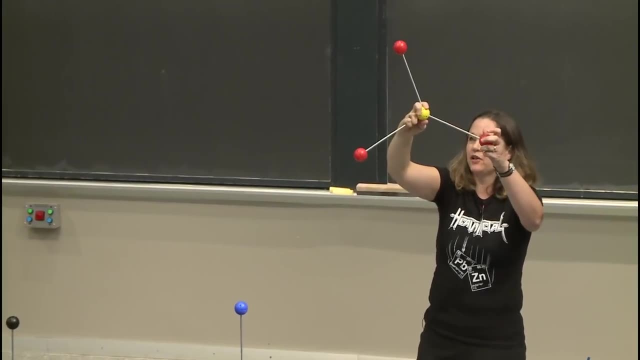 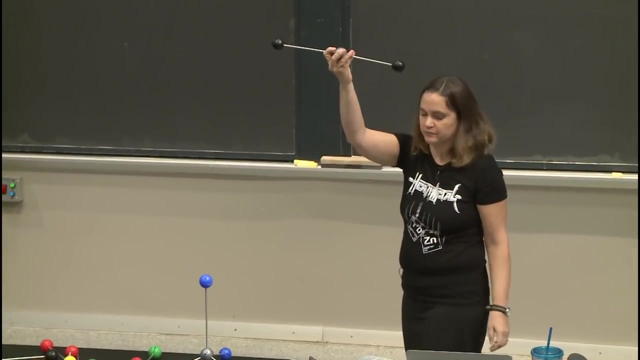 And now see a number of three. What is this one? Trigonal, planar. It's in a plane kind of if I hold the bonds so they don't fall off, and it's kind of trigonal. And then what about the last one? 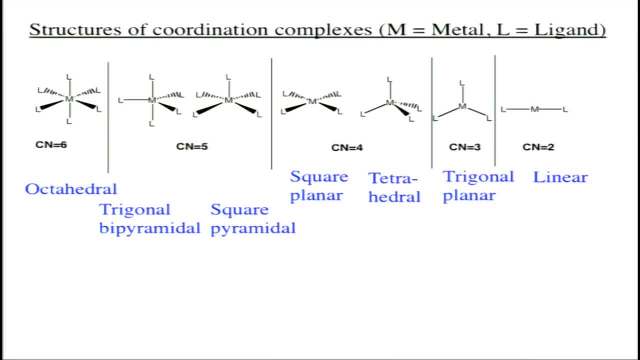 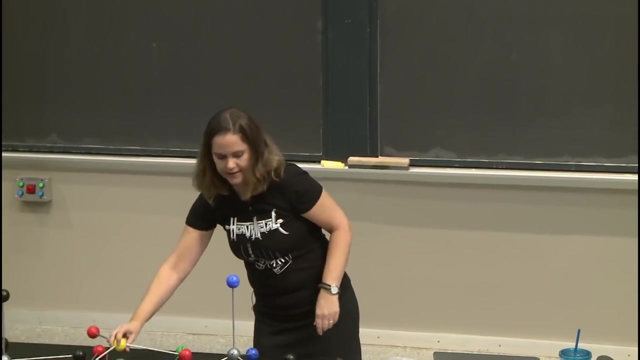 Linear. OK, And let's just run through and think about the angles as well. With octahedral, what are our angles? 90.. Trigonal, bipyramidal: 90 and 120, that's right. So we have 120 around here, and then the top parts were 90.. 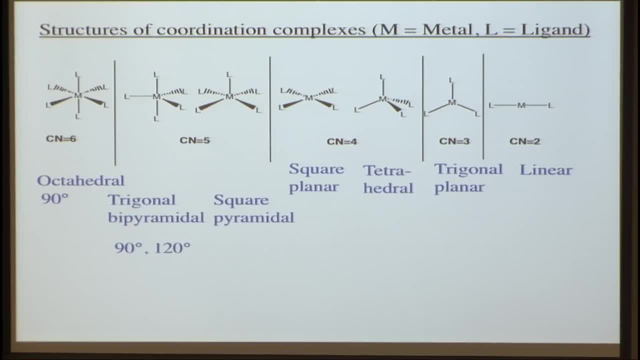 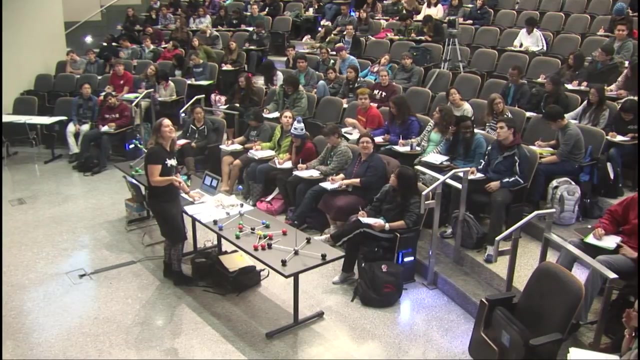 OK, We have the square: pyramidal: 90.. Square planar: 90. 90.. Tetrahedral: 109.5.. 109.5.. Give credit for 0.72.. That's quite close Trigonal planar. 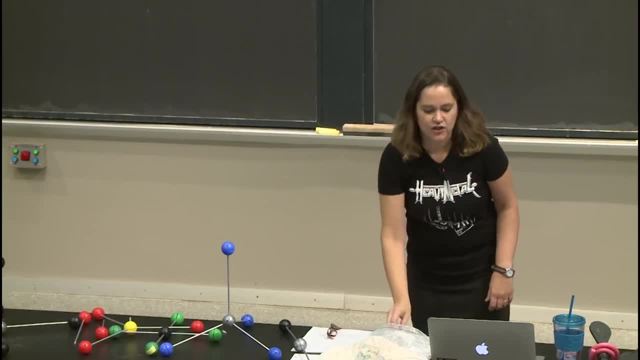 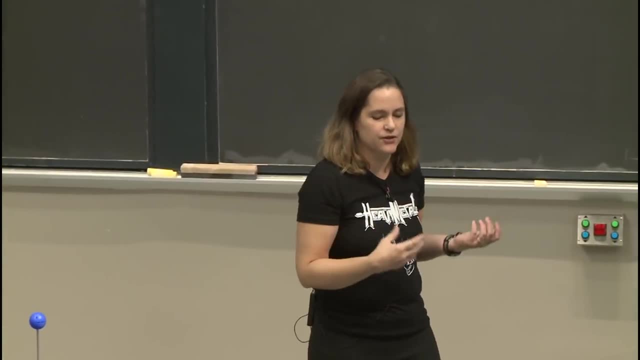 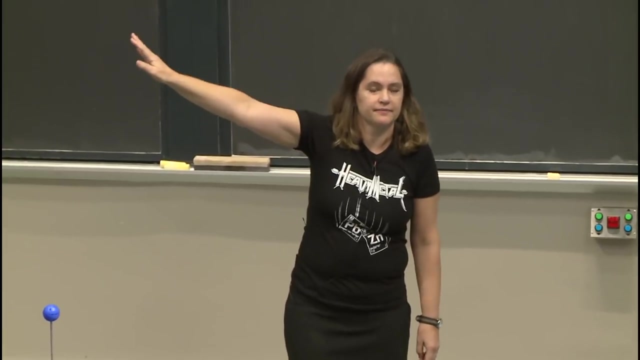 120 and linear 180.. Right, So you're going to need to remember these for this unit, but that's OK, because you need to remember them for the final anyway, So it gives you a nice review. All right, So we got everyone. so they got them down. 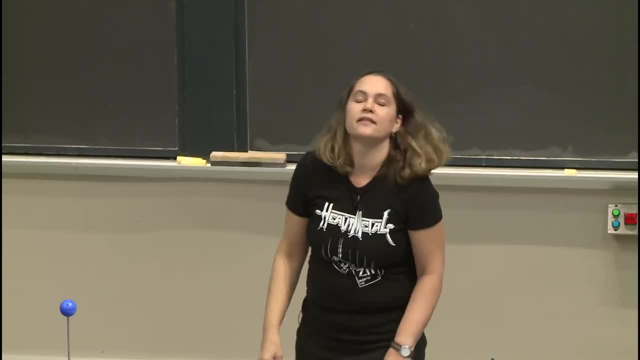 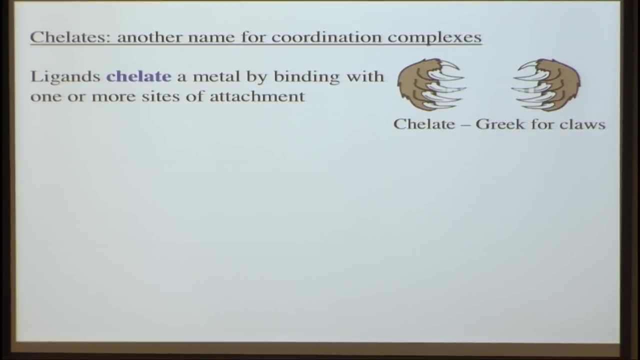 can look up your old notes, just review. All right, So coordination complexes also have another name. They can be called chelates, just another name for coordination complex. So chelates can be the thing, but you can also say that the ligand will chelate, as another way of saying. 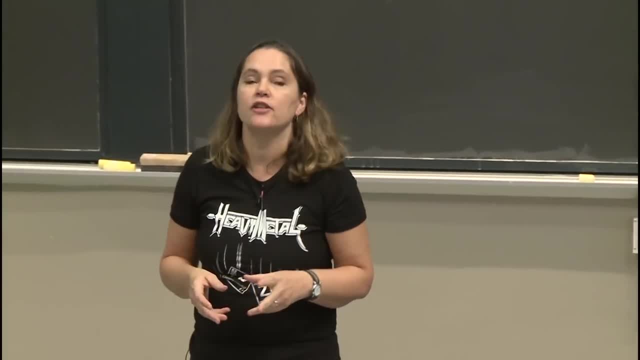 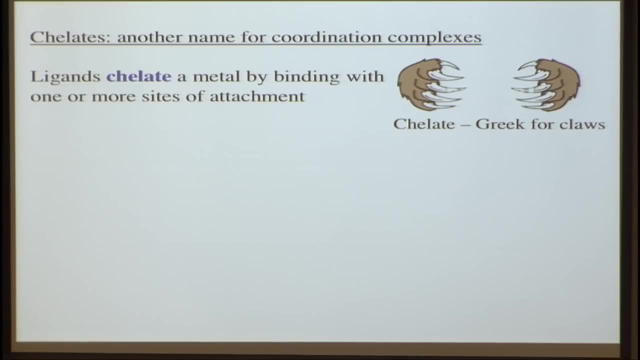 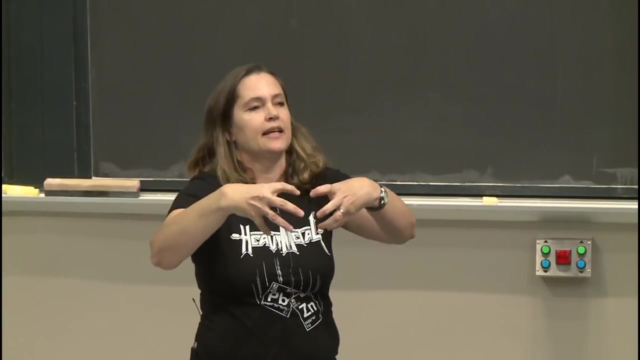 that it will bind to a metal And it can bind with one or more sites of attachment. And the word chelate comes from claws and I like that picture. I feel like, yes, these ligands coming in like claws and binding that metal, they're chelating that metal. 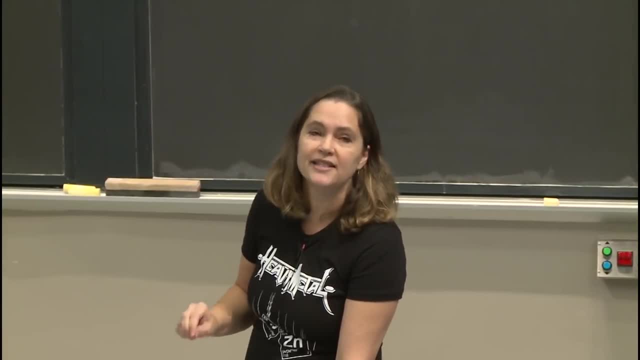 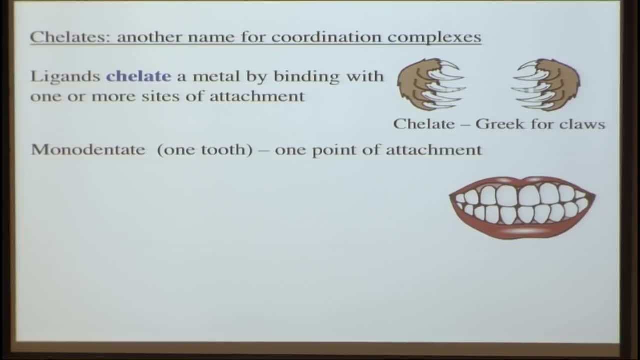 So they're different names depending on how many points of attachment they have. And we have what's known as monodentate, dent for dentist or tooth. So that's one point of attachment And I bet that without having seen this material ever before. 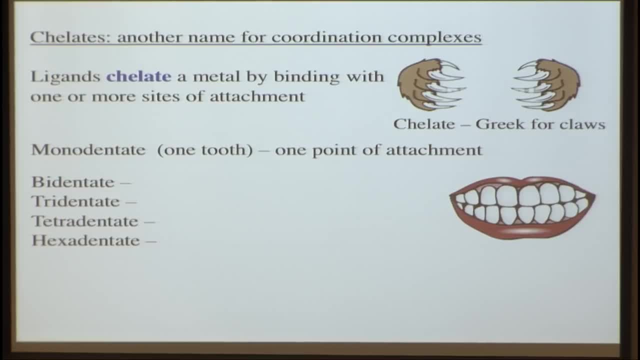 you can tell me what the rest is, What the rest of these are. What do you think? bidentate means Two, Two, Tridentate, Three, Tetradentate, Four, Hexadentate, Six, Six, All right. 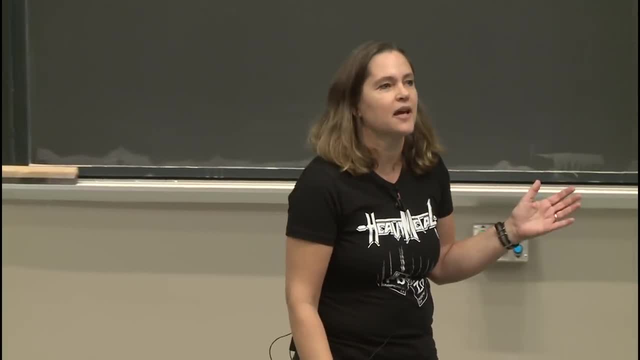 There's not one for five, But this is good, So don't lose a point on this. I feel like sometimes people lose a point on this in the exam. You knew it in class before I taught it. You know when I'd somehow work backwards. 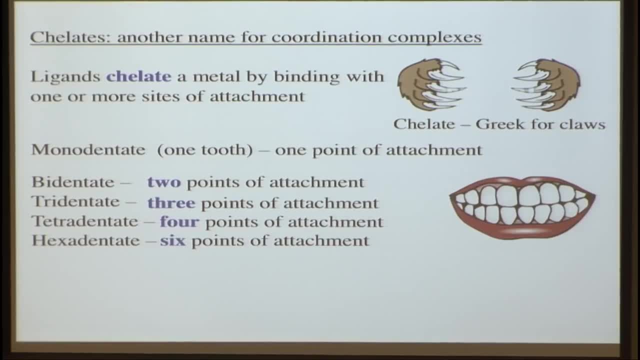 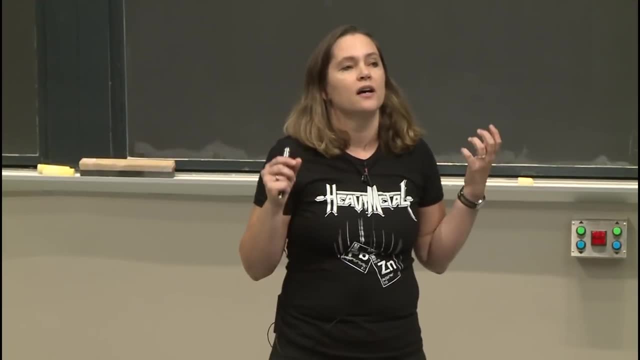 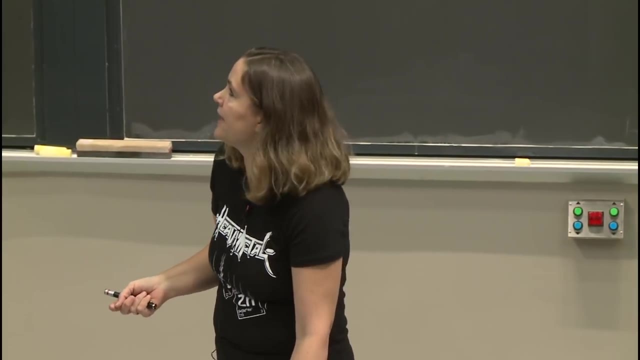 So this is easy: points right here. Just remember on the exam, wait a minute, maybe I already know this. All right, So let's look at some example of chelating ligands that bind with multiple points of attachment, And the first one. we're kind of on a theme today. 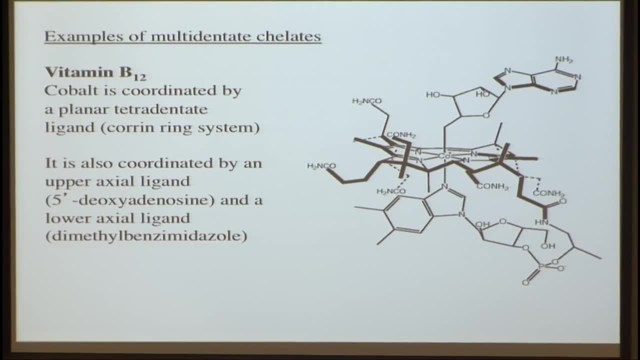 is vitamin B12 that we're going to look at. So this is called the Corin Ring. Cobalt is in the middle And that ring binds with four points of attachment. So it is a tetradentate ligand, this Corin Ring. 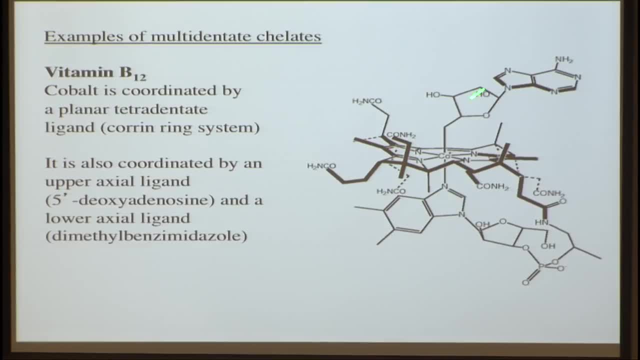 There is also an upper ligand, which is 5-prime deoxyadenosine, and a lower ligand that's called dimethylbenzamidazole. You don't need to know their names. Overall it has six ligands in octahedral geometry. 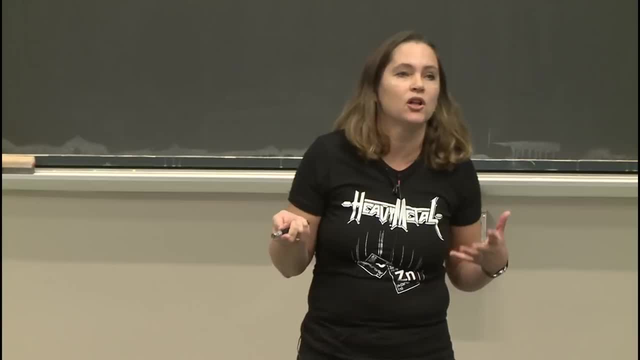 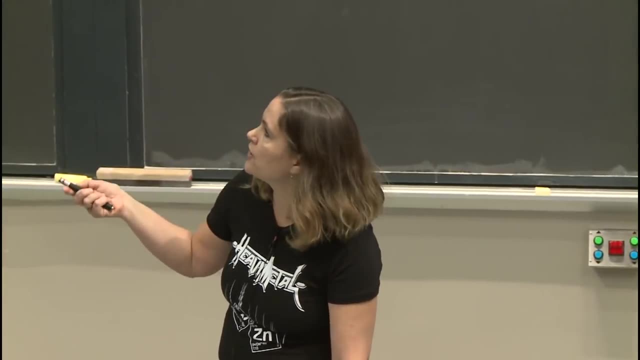 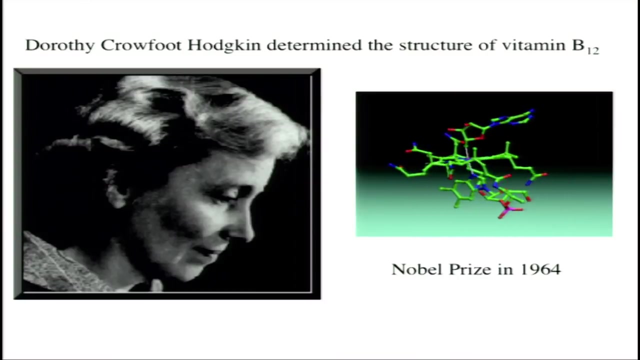 But the Corin Ring is a very nice biological example of a multidentate ligand. Heme would be the same. I thought I would show you this rotating around so you get a better sense, and tell you that this structure of this vitamin was determined by Dorothy Hodgkin, who 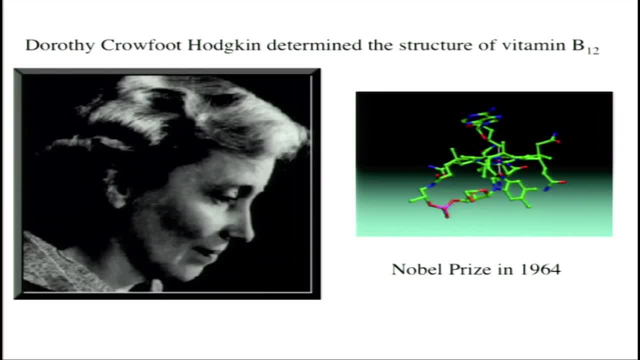 won the Nobel Prize in 1964 for determining the structure by crystallography and also solving the structure of penicillin. This was the most complicated molecule to be solved by crystallography And a lot of people said that technique could never. 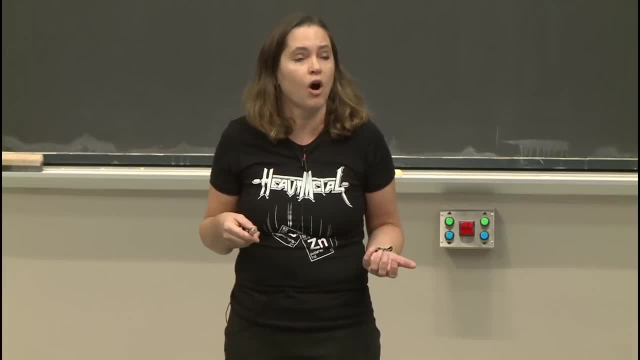 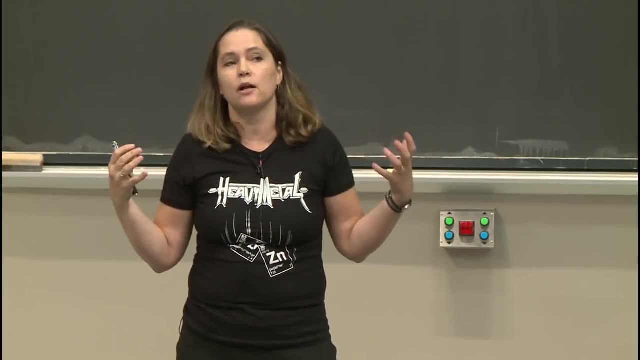 be used to do something that big. She showed that they were wrong In terms of determining the structure of penicillin. it was during the war And people wanted to make more penicillin, but they had no idea what the structure was. 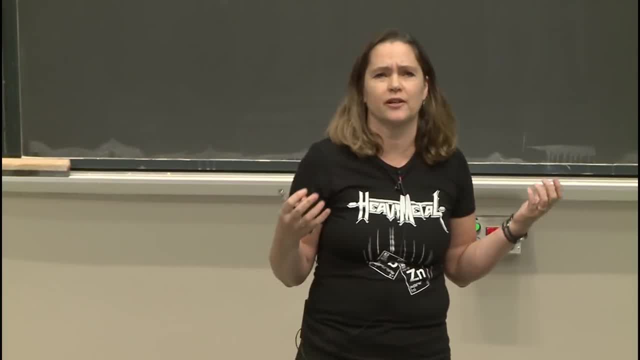 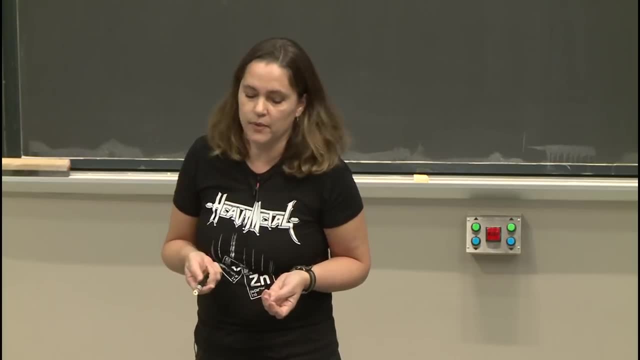 so they didn't know what to make. And she figured out the structure. And it's a weird-looking molecule so no one would have guessed it without knowing the structure. So for her pioneering work in crystallography she won the Nobel Prize. 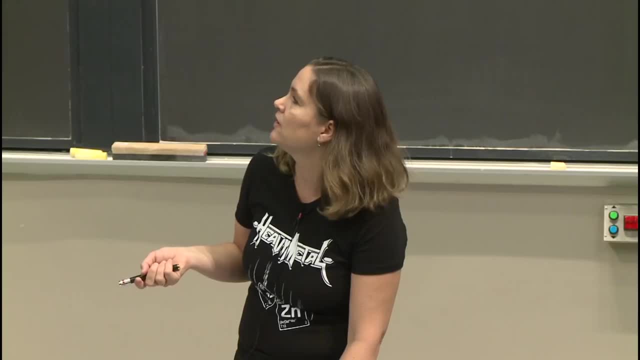 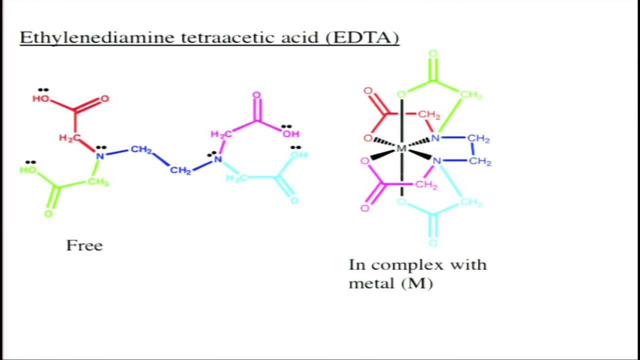 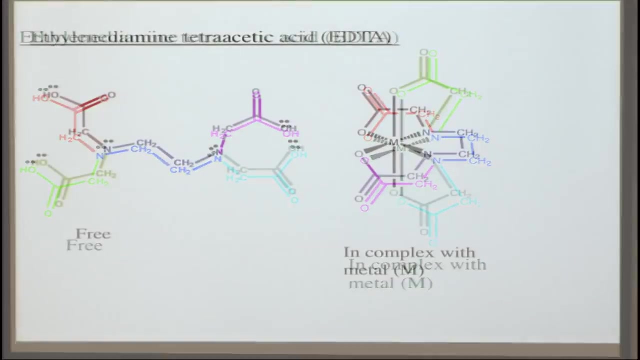 All right. so vitamin B12 is one example of a chelate. Another- that's probably more- that you probably hear about the most. it's almost synonymous with the word chelate is EDTA. OK, Here is the EDTA molecule. 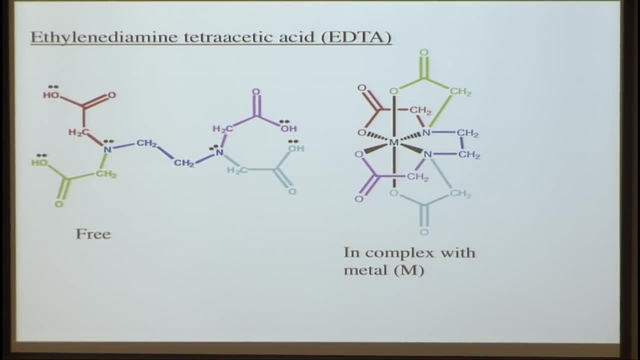 And you see that it has lots of lone pairs that are just dying to grab onto a metal. So we have six. We have one, two, three, four, five, six, Six things that are capable of chelating that metal. 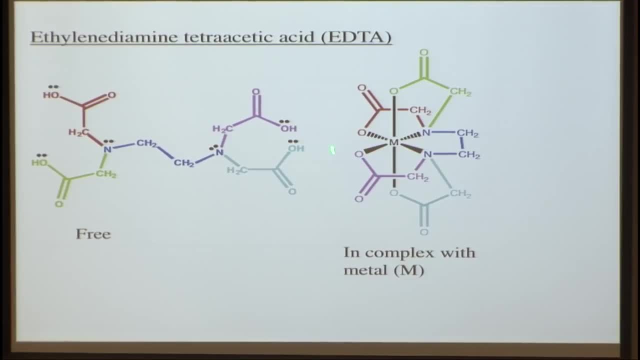 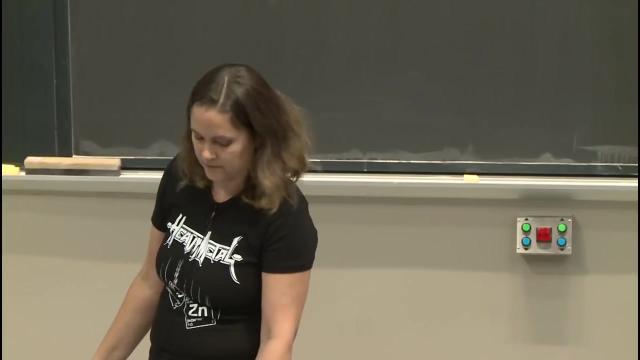 And so here is what the complex looks like. So the red oxygen can chelate, The green oxygen here can chelate, Nitrogen here in dark blue, the other nitrogen in dark blue here, light blue oxygen here, and also the purple oxygen. 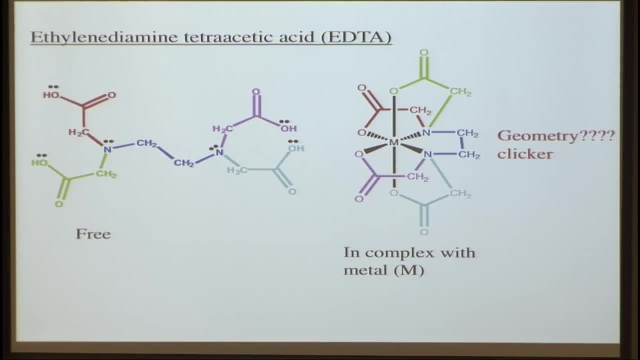 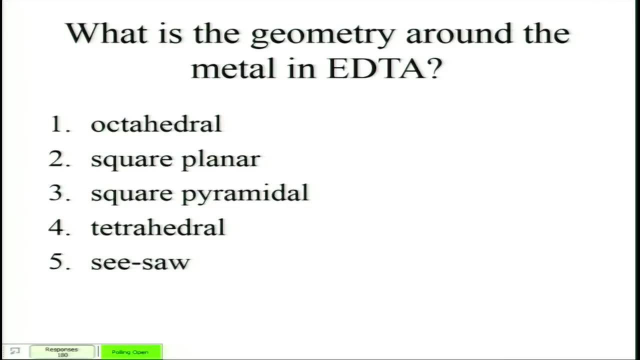 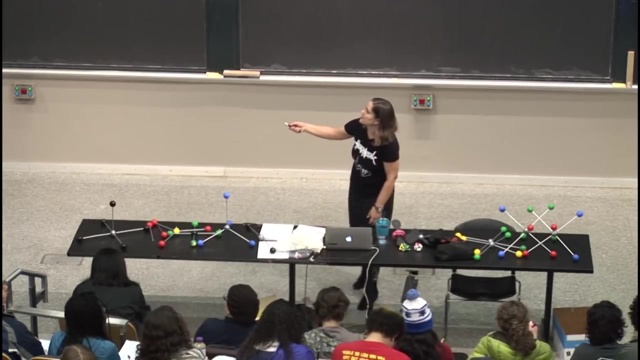 So now, why don't you tell me what the geometry of this would be as a clicker question You ready? Yeah, It should be fast, hopefully. Yeah, great 86%. It is octahedral And sometimes it's a little bit hard to see that. 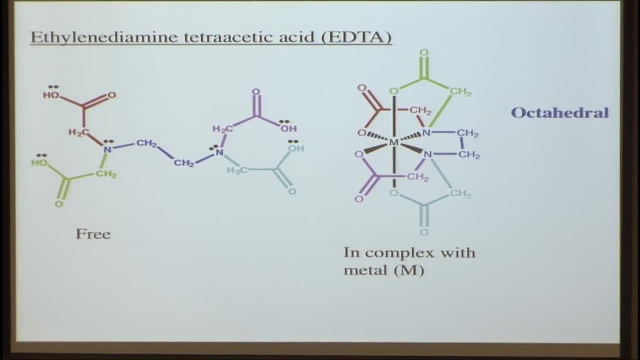 but I helped you out by drawing those bonds in black that you needed to look at. So we have four that are in the plane here, one above and one below here. So that is octahedral geometry. Also, how many points of attachment? 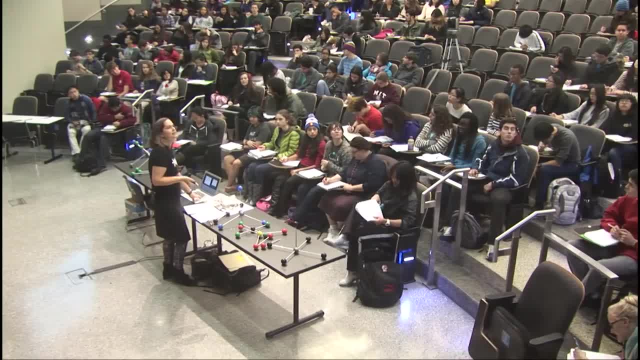 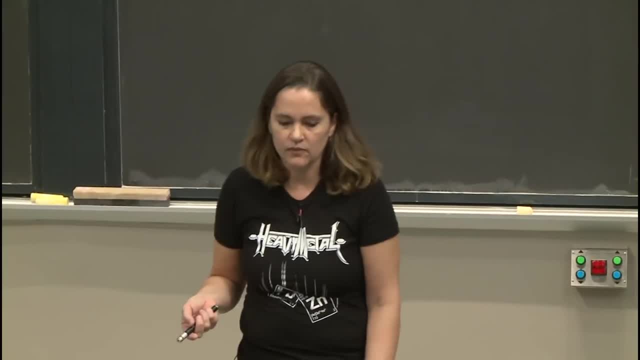 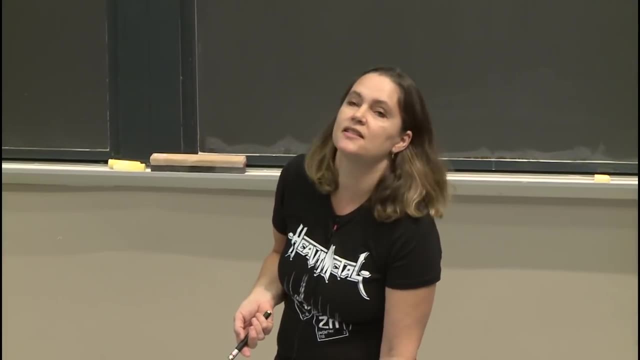 What kind of dentate ligand is this? It's hexadentate as well, So it has six points of attachment here. All right, So EDTA is a really good metal chelator And part of the reason that it is such an awesome metal chelator. 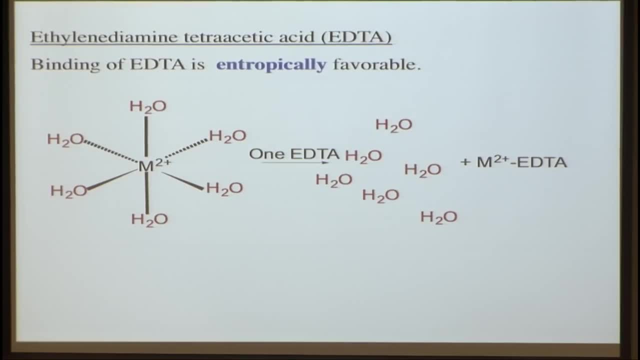 is because of entropy. So we're back to entropy again. So the binding of EDTA to the metal is entropically favored, And the reason for this is that metals that are, say, in your body, like if you happen to eat some lead paint. 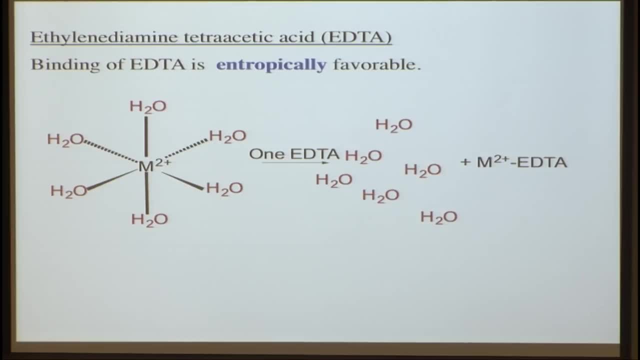 and that lead is hanging out. It's not just by itself, It's coordinating, hopefully just to water and not to proteins in your body. But when you take some EDTA to prevent it, to prevent your lead poisoning one molecule of EDTA, 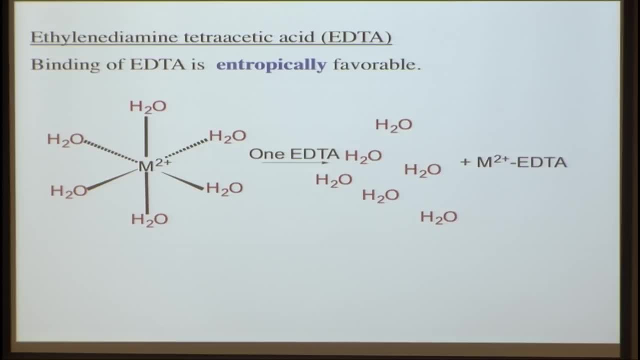 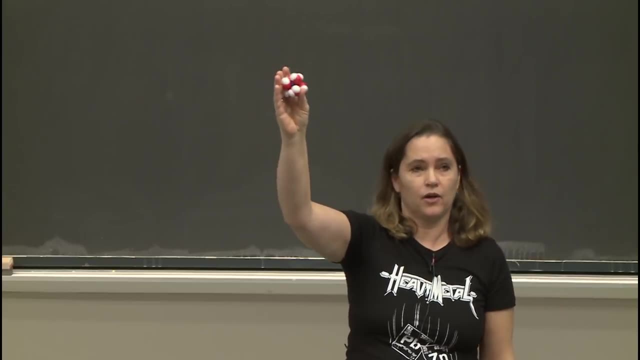 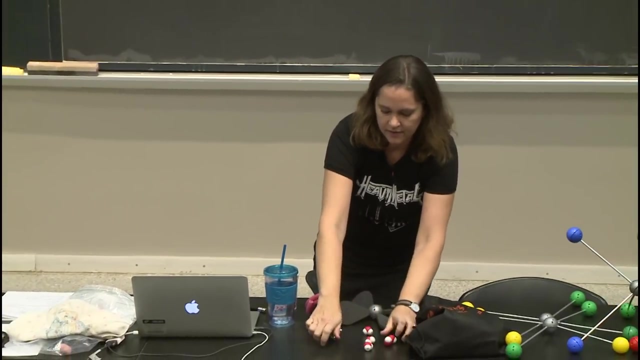 will bind the metal And all of these waters are going to be released. So I have over here some lead with a whole bunch of little waters. This is quite an ordered system, But if I take out all of those waters here that's a lot more entropy going on than what we had. 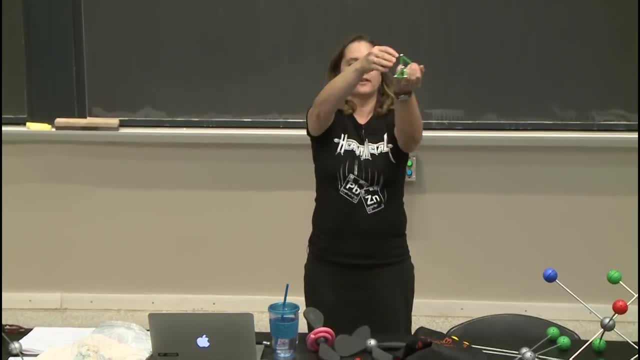 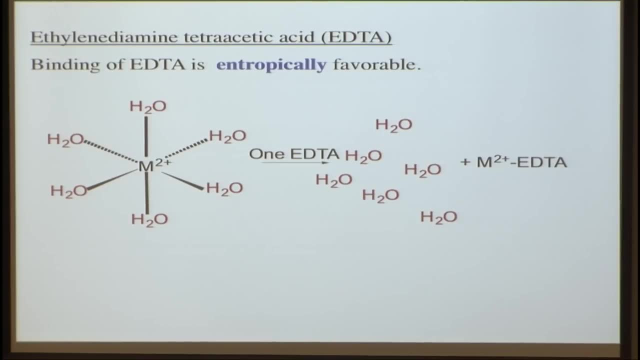 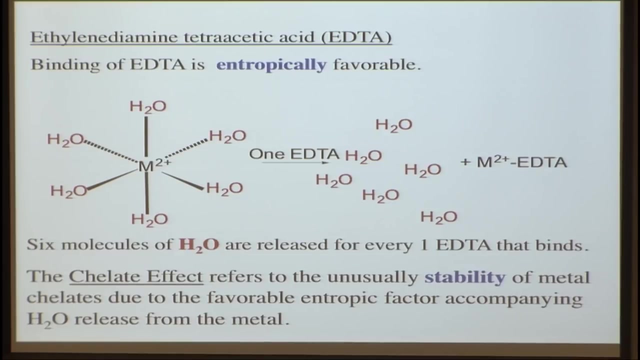 And then you have one chelating ligand here, And that's a pretty simple system. So this is ordered, This is disordered. So the binding of EDTA: one EDTA releases six water molecules, And that makes it very favorable to do this. 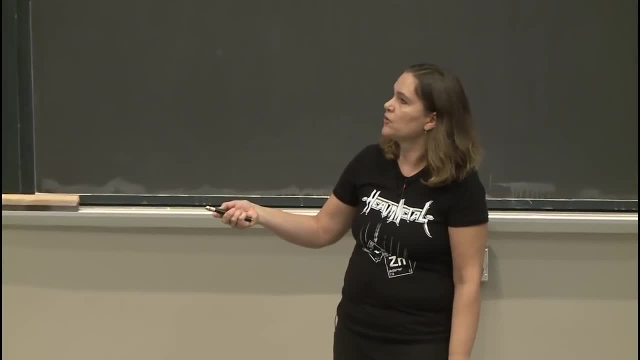 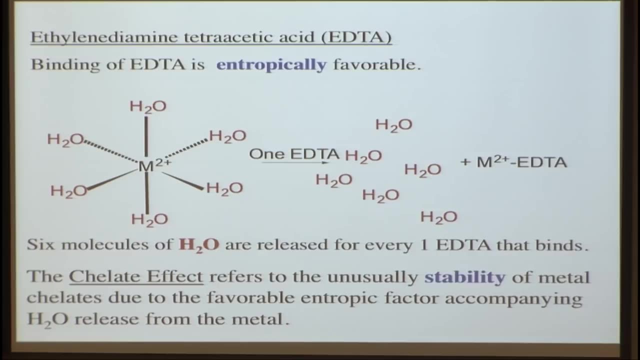 And because of that, chelating molecules, or the chelate effect, molecules that are chelates like metal-bound EDTA, are unusually stable because of this favorable and favorable entropic effect, this release of water. So the release of water, the release of increasing entropy. 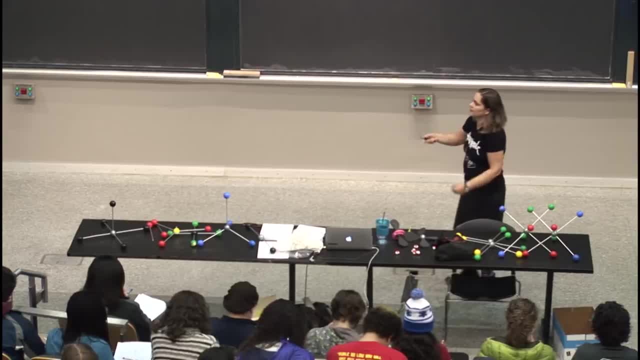 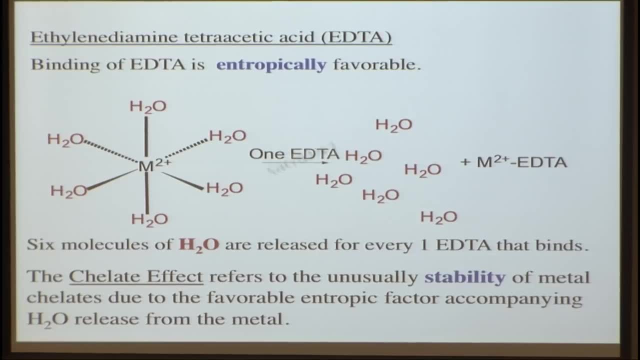 drives that metal chelation And you sequester your metal, which is really good if you're trying to avoid lead poisoning. So I think this is a nice example of our friend entropy driving a reaction. So a lot of you did really well on the exam. 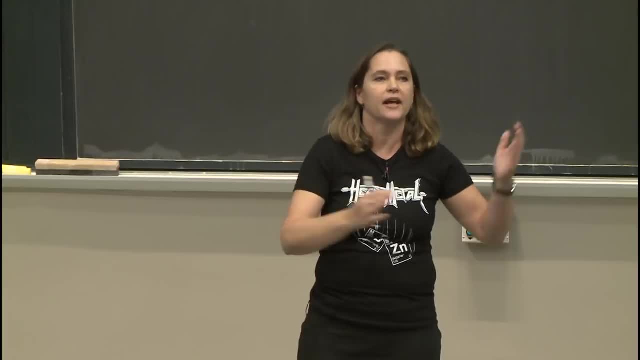 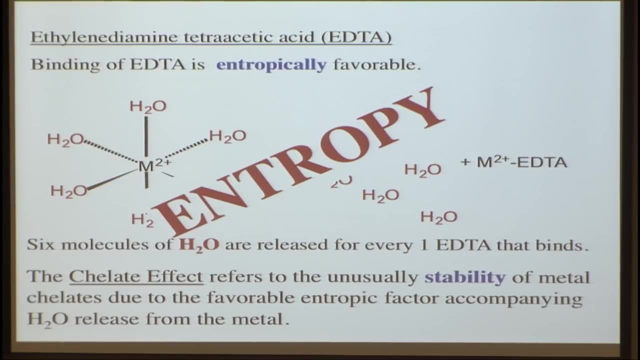 talking about factors of delta H and entropy, and when you'd have favorable delta Gs. Here's another nice example where the chelate effect explains why metal chelates are so unusually stable. All right, So uses of EDTA. I already just told you one. 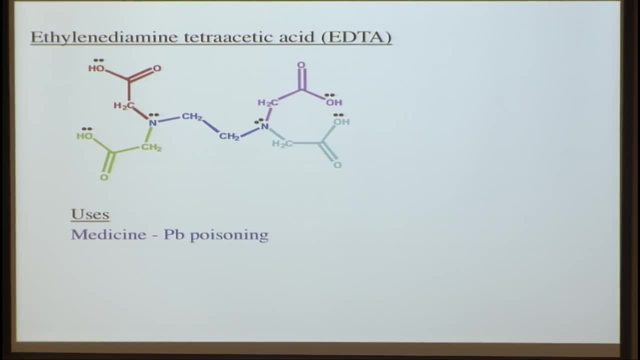 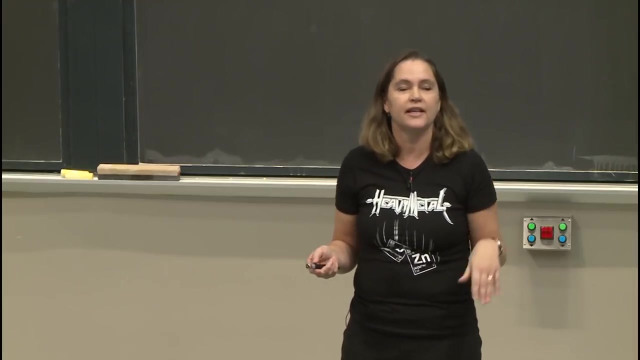 Lead poisoning: All ambulances have EDTA in case someone is eating some lead paint. Another thing that EDTA is used for, which I think is fun: you should all go check if you buy little packaged goods And they have a long list of chemical ingredients. 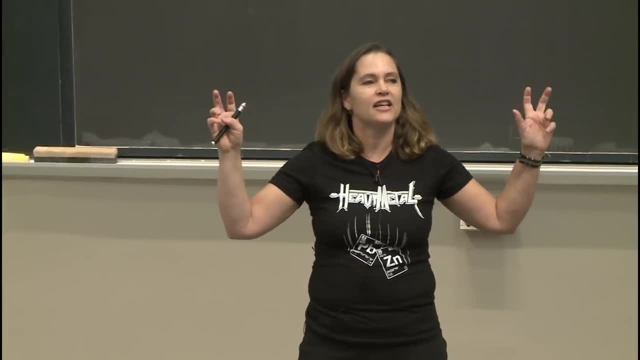 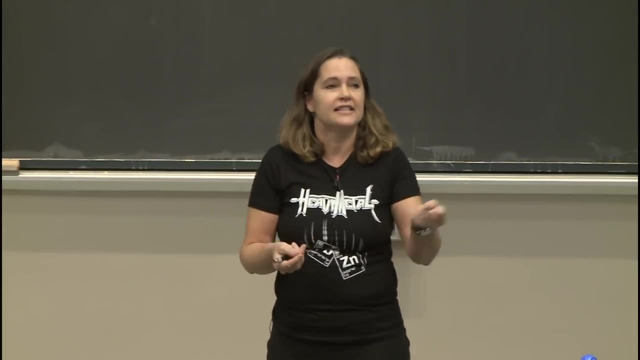 Look for EDTA. It's often there And it says it Added for freshness, which means that bacteria need metals. You have EDTA. EDTA sequesters the metals so the bacteria can't live on the food that you're eating. 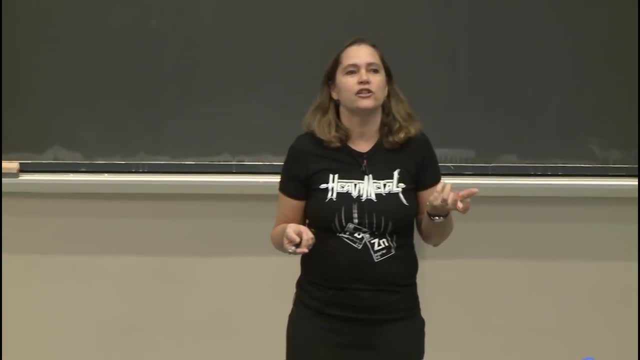 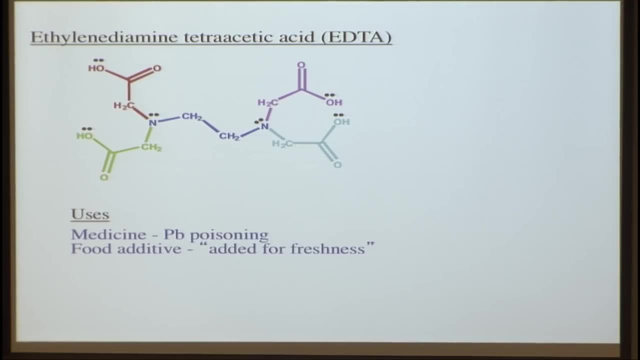 So instead of saying food additive, added to kill the bacteria that were otherwise growing on your food, they say added for freshness, And I do think that is an improvement. All right. Another thing: we've already talked about the importance of cleaning bathtubs. 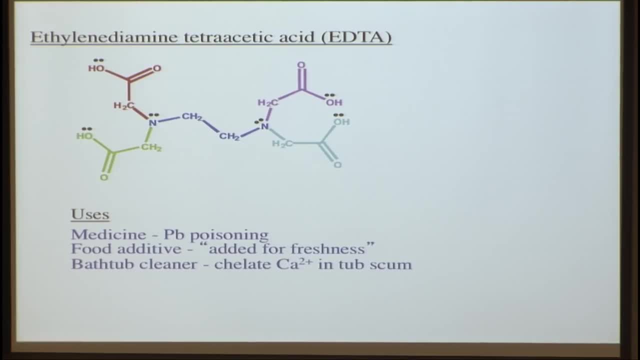 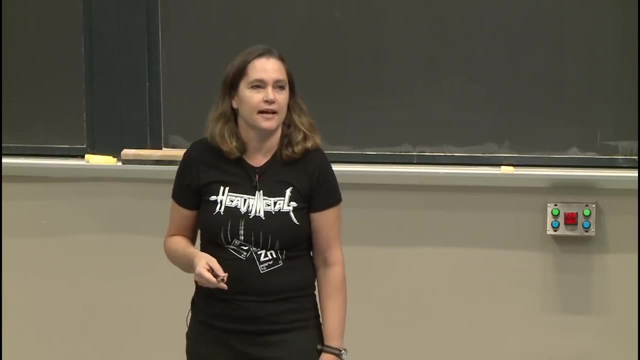 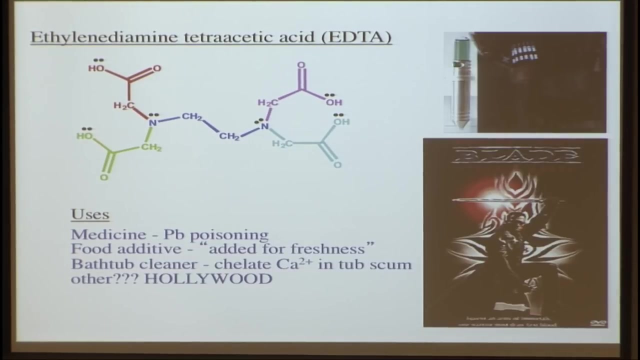 To chelate calcium out of bathtubs- scum- you have EDTA or other metal chelates And then I have my favorite other example of the use of EDTA. This favorite example is in Hollywood, the movie Blade. How do you kill a vampire? 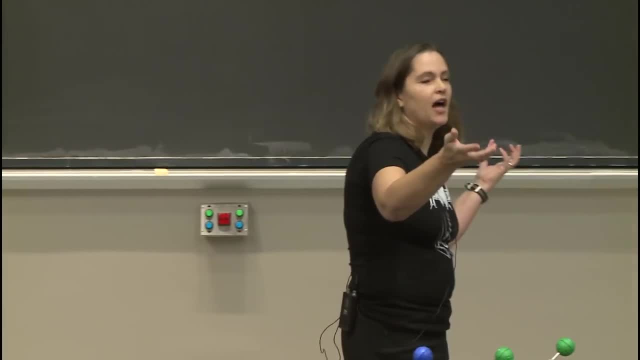 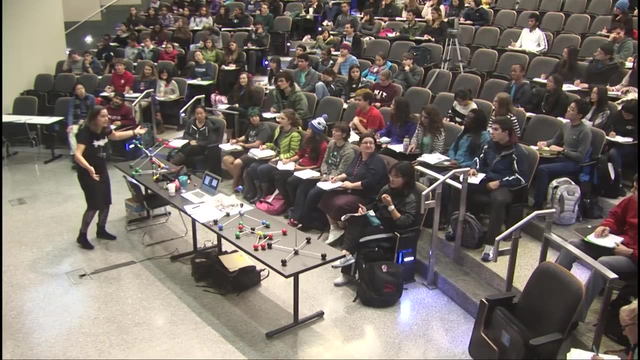 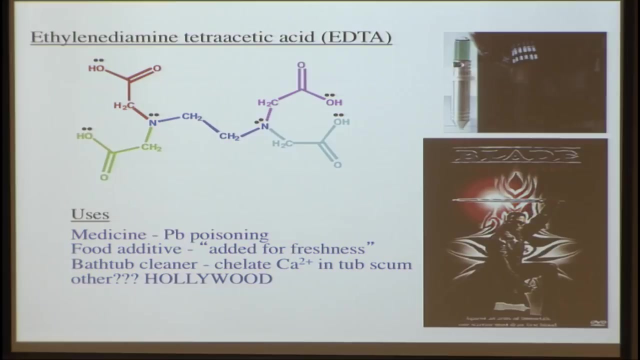 Vampires drink what Blood? Blood has iron. EDTA chelates Iron, So you get a little dart And you have. you can kind of see them maybe up here. They're filled with liquid. That's EDTA. 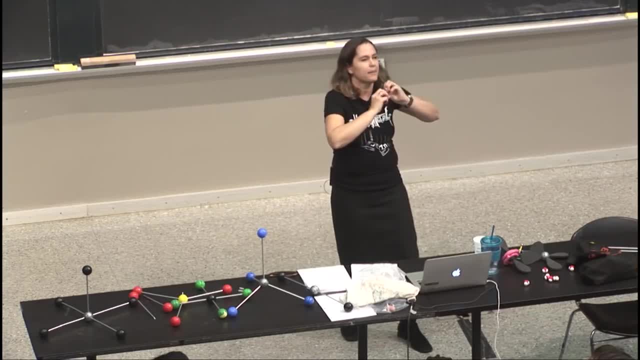 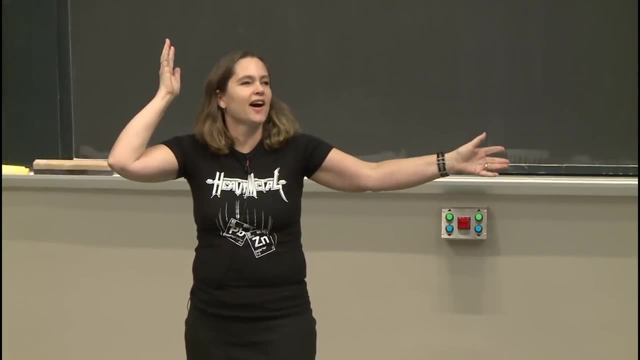 You shoot the vampire with EDTA and the vampire just disappears, just kind of turns to sort of dust, Because it's like mostly iron and the iron gets chelated. But it happens right away. But anyway, I think that's cool. 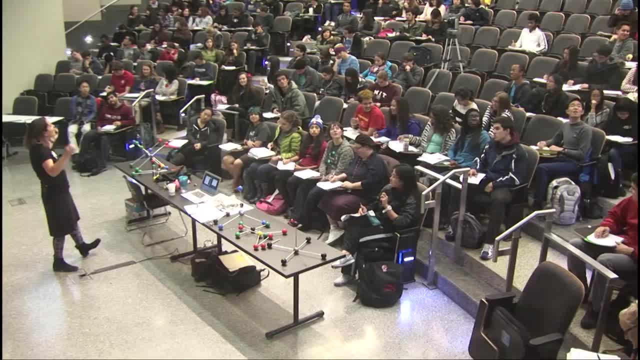 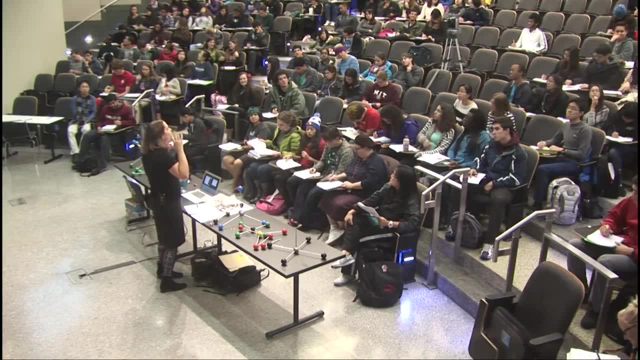 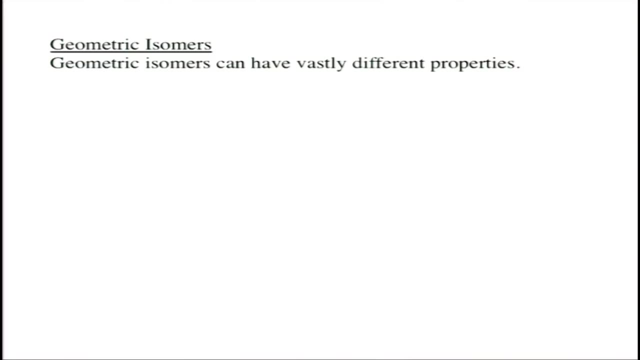 Yes, what a good way to kill a vampire. EDTA- it's brilliant. Excellent use on Hollywood's part for EDTA. OK, Metal chelates- all sorts of potential values that they have OK. So when we're talking about coordination complexes, 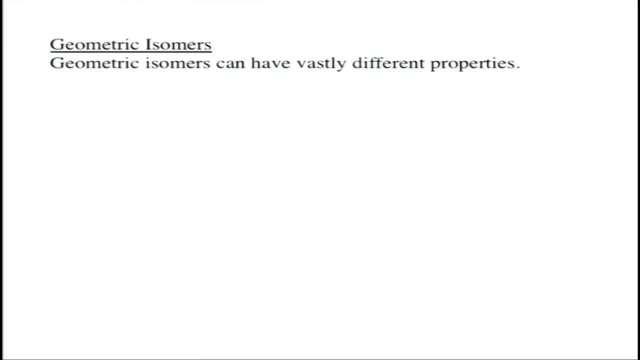 we're talking about geometries. sometimes the atoms can be arranged in different ways, And when you have these geometric isomers, they can have very different properties. So just look at an example here. It's a platinum compound, a platinum compound who has two NH2 groups and two chlorine groups. 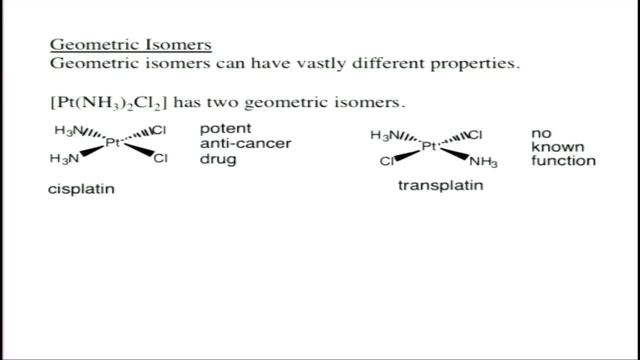 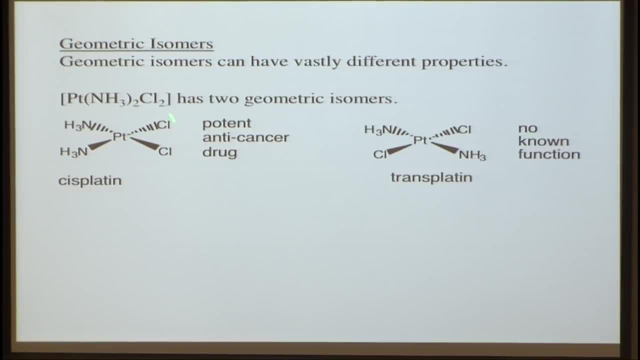 And you could arrange those in two different ways. You could put the NH3 groups on one side and the chlorine groups on the other side, And that would be cis. These are cis to each other. Or you could put a trans configuration where chlorine is here and then the nether chlorine. 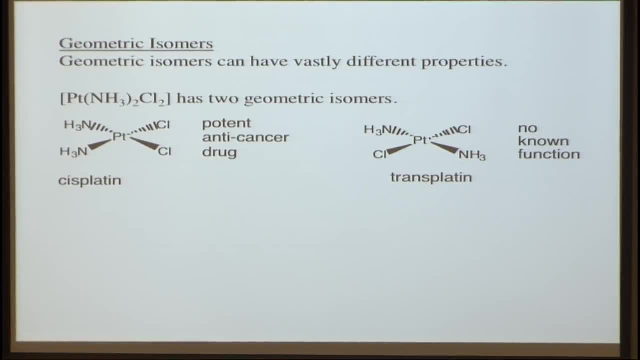 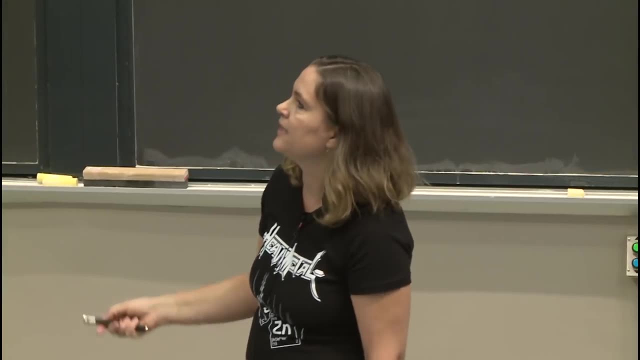 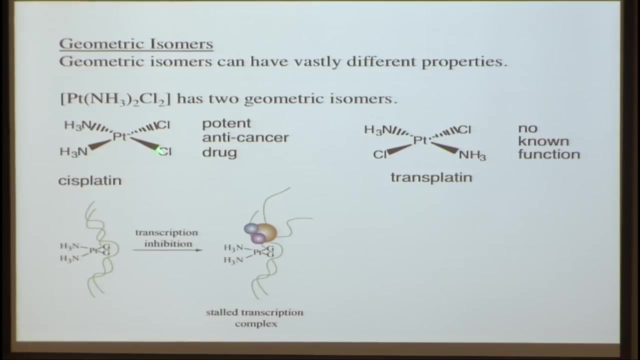 is trans on the other side and the same with this. So cis platinum here is a potent anti-cancer drug And it has to be cis platinum because it binds to DNA And the two bases of DNA displace these chlorines. So if they're not on the same side, 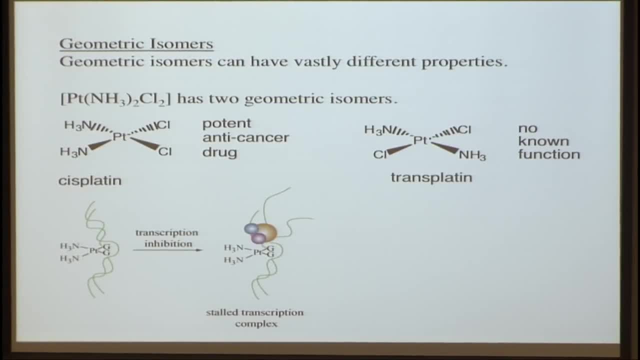 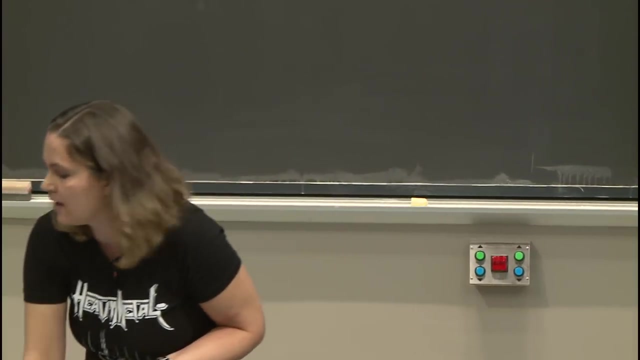 it can't bind to the DNA, And so this prevents the cancer cells from being repaired from damaging agents. Trans platinum does absolutely nothing than anything Anyone knows. So it's exactly the same composition, but because they are different isomers from each other, 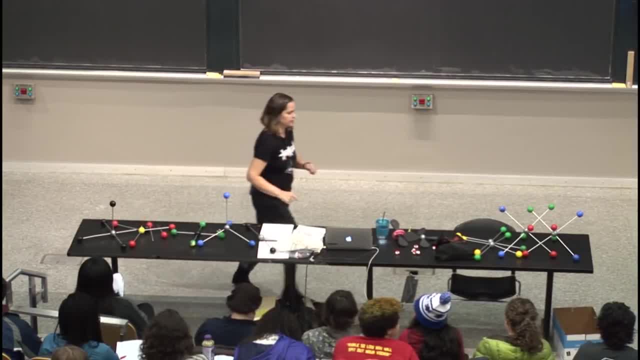 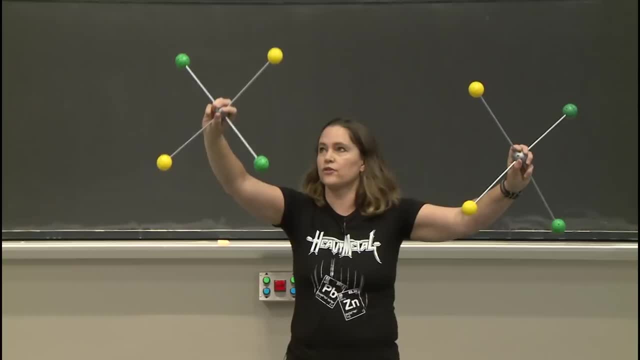 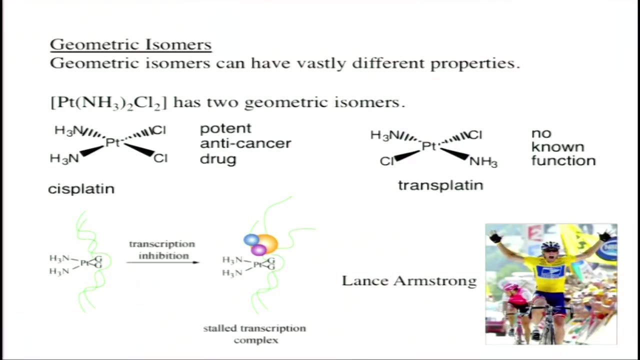 And I have- let's see over here- different isomers of each other, And so chlorines on the same side, cis versus the trans have completely different properties. So cis platinum got a lot of fame because it cured Lance Armstrong of cancer. 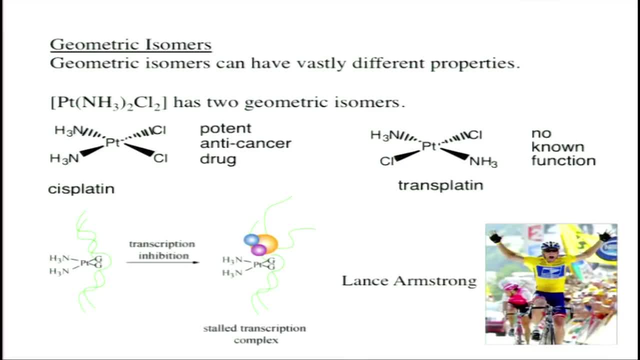 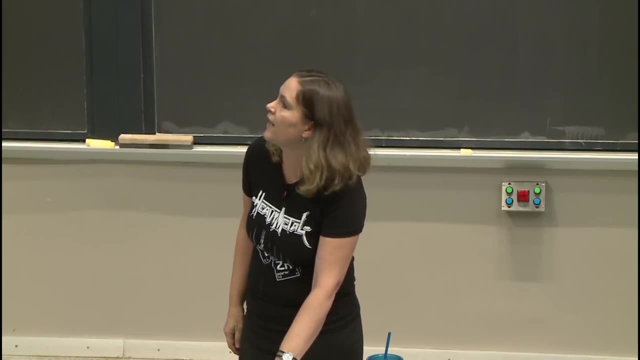 Lance Armstrong now, of course, is a much more controversial figure than he was at the time, But still he created an amazing charity that hopefully, is still doing well despite some of his fall from fame. OK, So another type of isomer are called optical isomers. 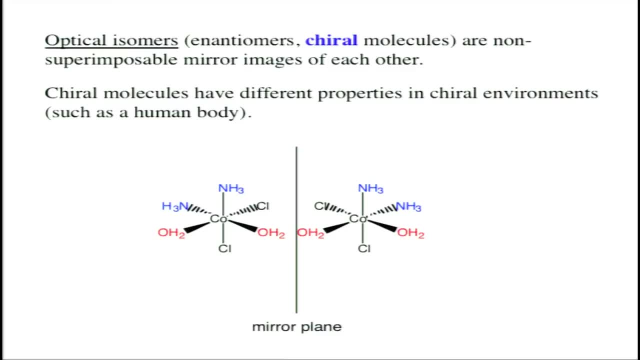 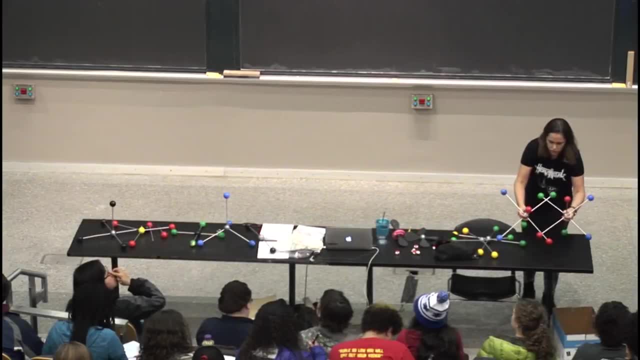 also called enantiomers or chiral molecules. And these are one. again, you have the same composition, but they are non-superimposable. They are, in fact, mirror images of each other. So if my head was a mirror, these, 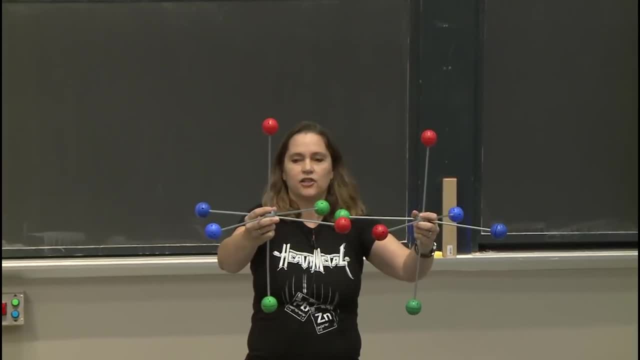 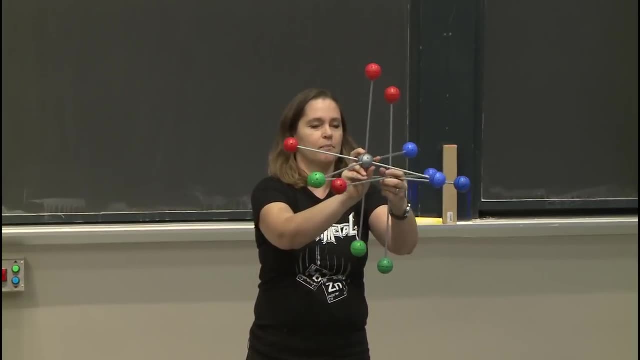 would be mirror images of each other And I could try very hard to superimpose them, bringing the blue molecules over here, but then the green and the red don't match. You can come and try. These are in fact non-superimposable mirror. 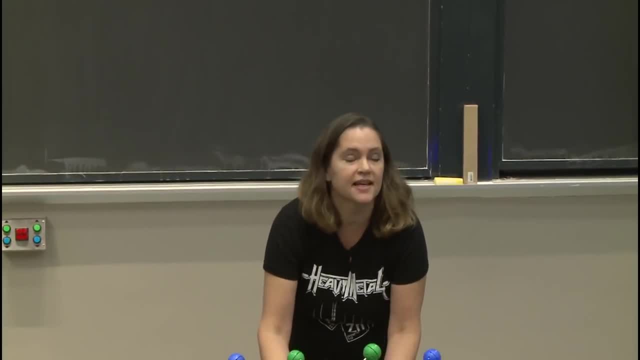 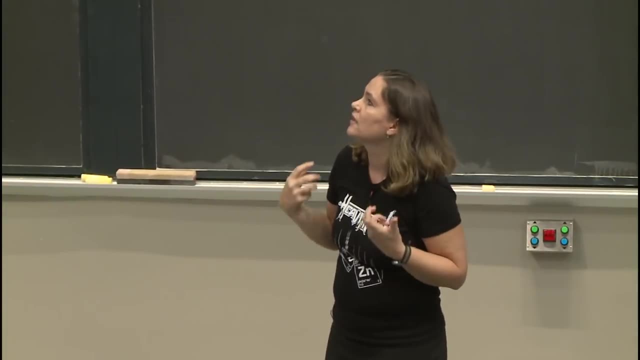 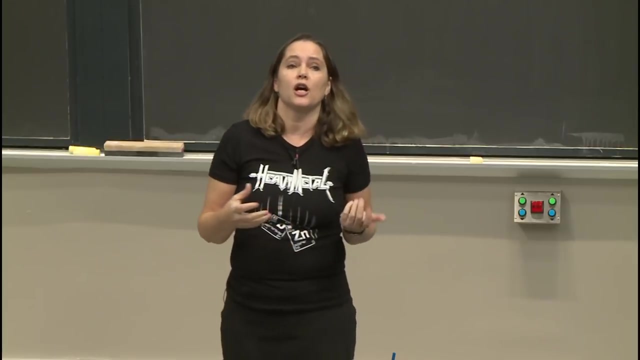 images from each other And sometimes they can have very similar properties. It depends, But if you put molecules like that that are known as chiral chiral molecules, ie enantiomers, non-superimposable mirror images, the human body is very much of a chiral environment. 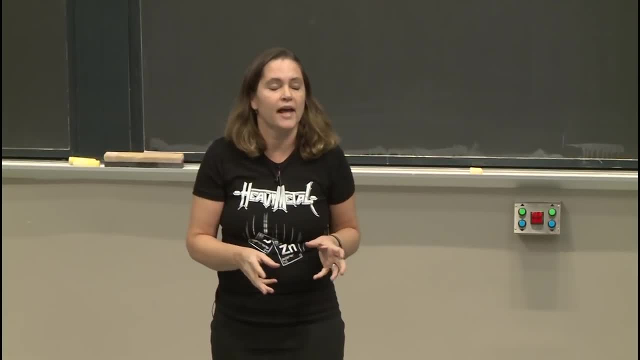 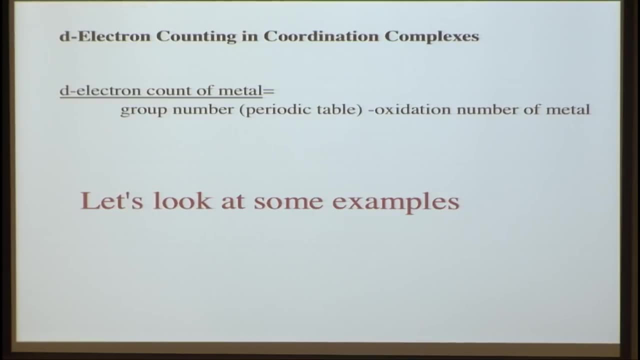 You have enzymes designed to bind things in a particular way, So they can have very, very different properties. OK, So we have to do some d-electron counting before we end today, And I love this because it's really pretty simple to count d-electrons. 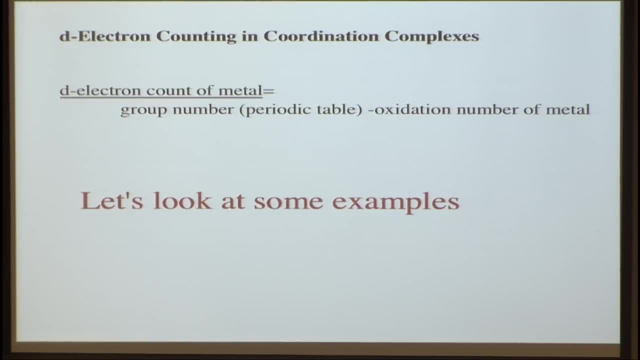 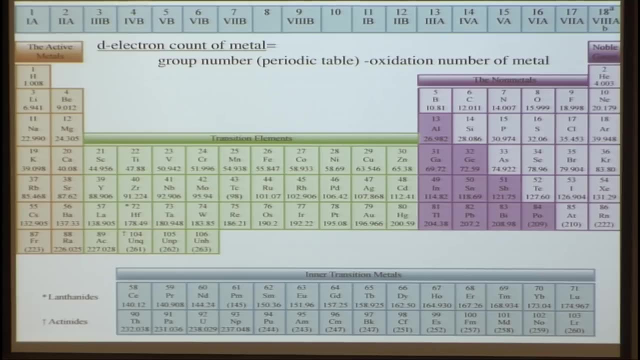 And so we're going to just take a look at some examples And for this, doing this part, we're going to start using our friend the periodic table again, And we need to find oxidation numbers, which we just talked about in the last unit. 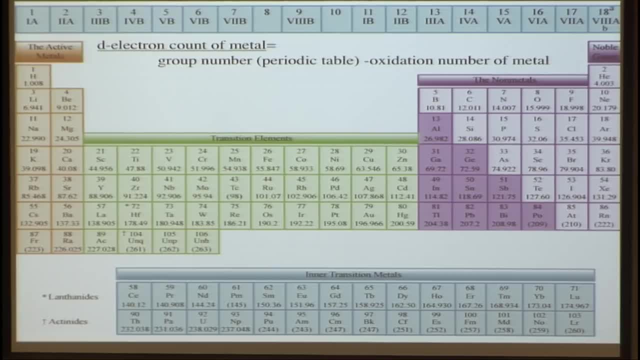 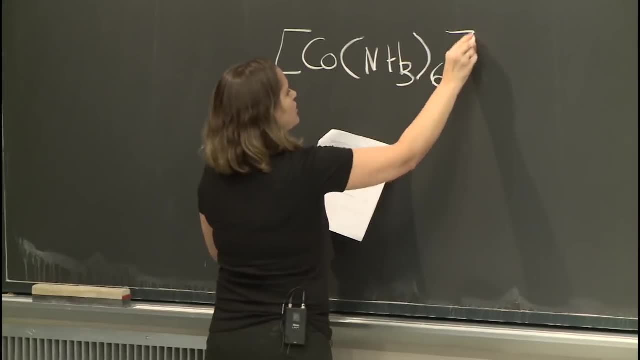 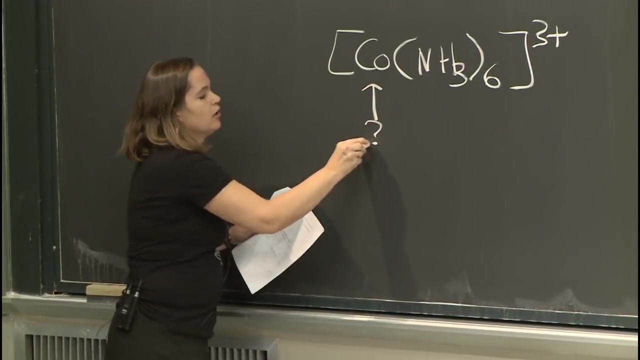 So if we have a coordination complex with cobalt, and this cobalt has those six NH3 groups and our plus 3-chloride, So this is the complex that we have been talking about. Let's now figure out what the oxidation number of this is. 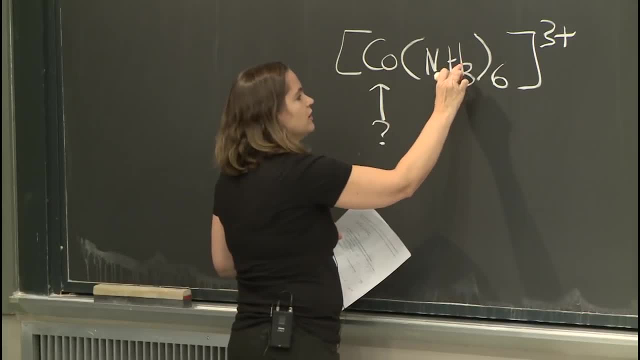 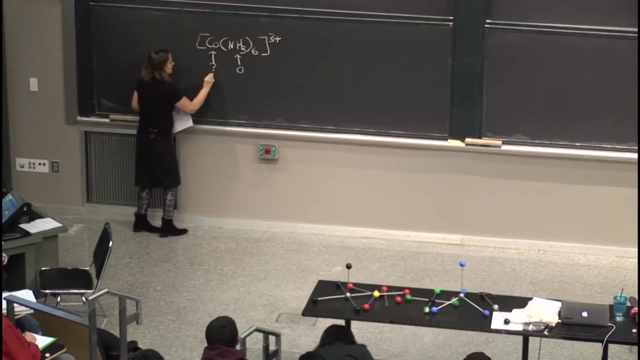 And so this NH3 is neutral. So that's given as a hint: Many of our ligands are going to be neutral ligands. So if that is 0, what is the charge on the cobalt Plus 3.. Now we're going to use the rules of d-count. 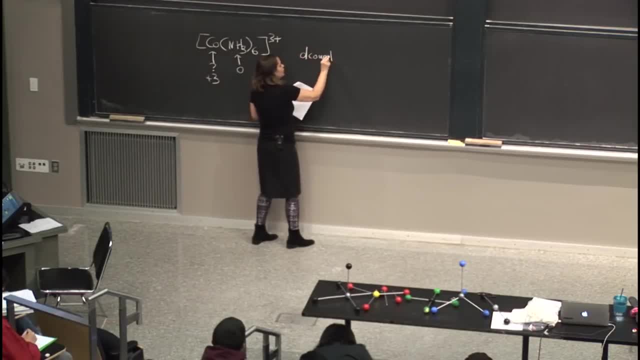 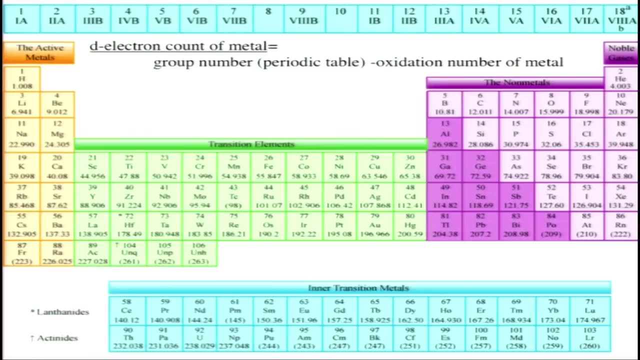 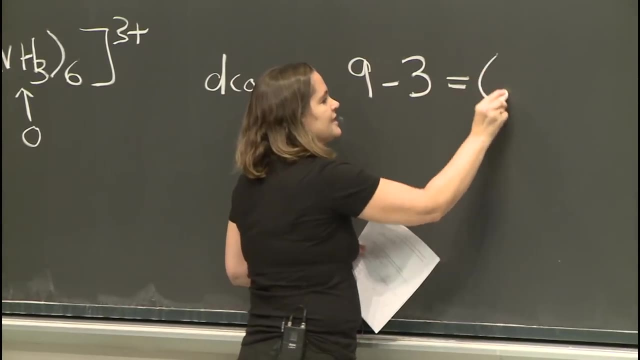 So we have a d-count. We need to look up the group number from the periodic table, which in this case is 9.. Then we have minus the oxidation number, So we have 9 minus 3, or 6. And so this is a d-6 system. 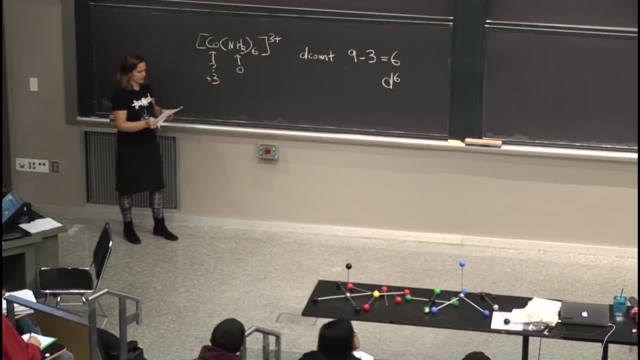 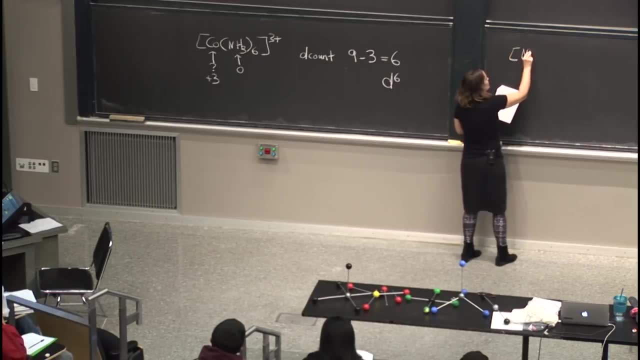 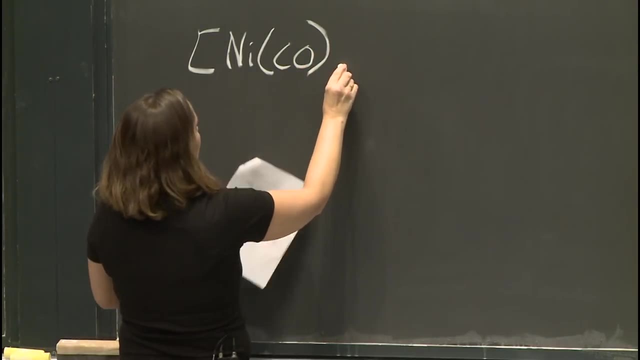 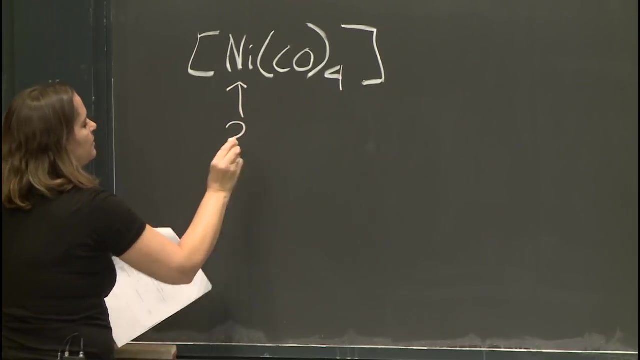 And that is all there is to doing with these counts, So let's just try another one. So we heard about nickel. We'll do nickel. Nickel is coordinated by carbon monoxide And there are four of those. So what is my charge of the nickel? 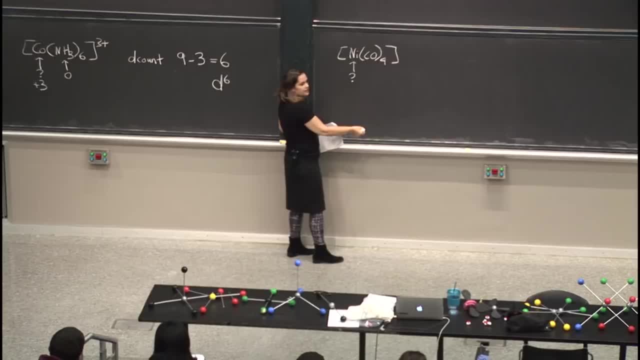 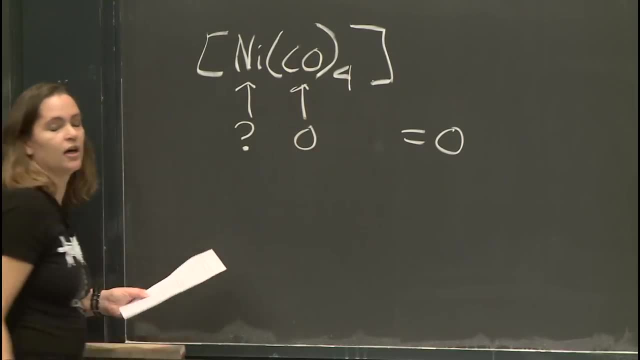 going to be my oxidation number of the nickel. So what's my overall charge of this complex? 0.. CO is also going to be 0.. There's no charge on CO, So what is the oxidation number of nickel? 0.. 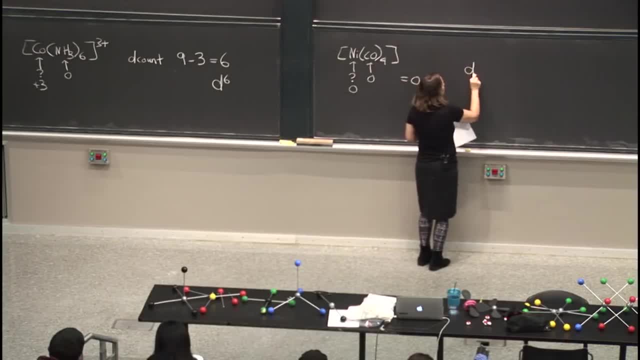 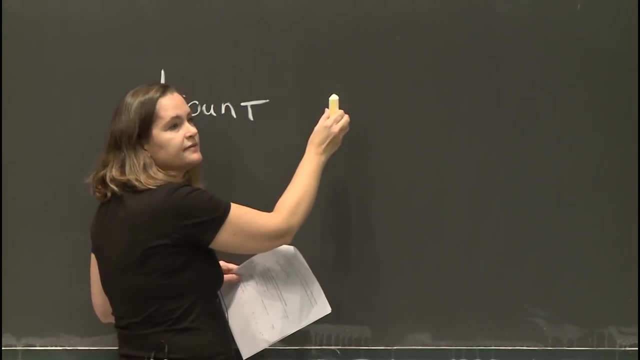 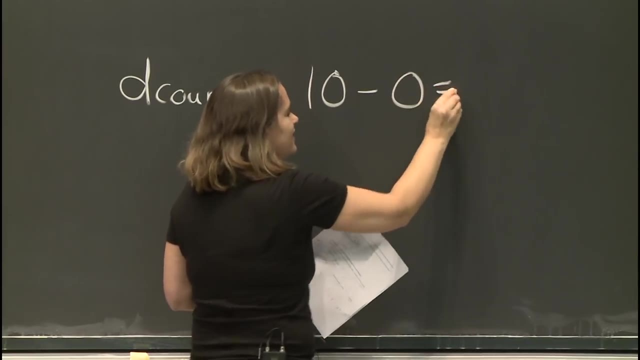 0.. So then we can do our d-count The d-count. what is the group number for nickel? What is it? 10. 10. This is the kind of math that always makes me very happy. 10 minus 0 is. 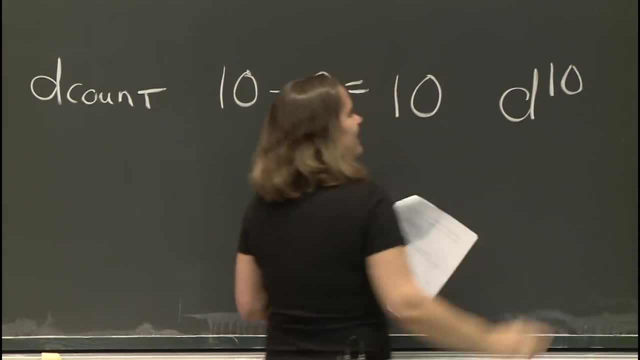 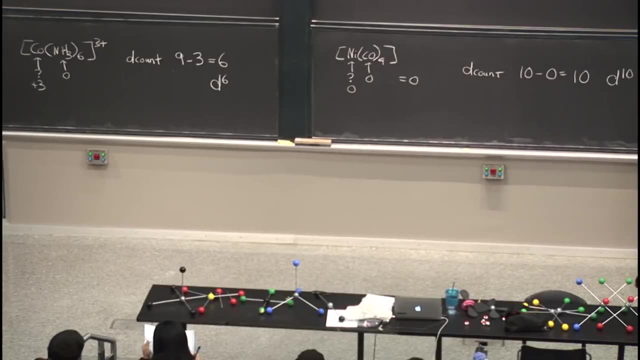 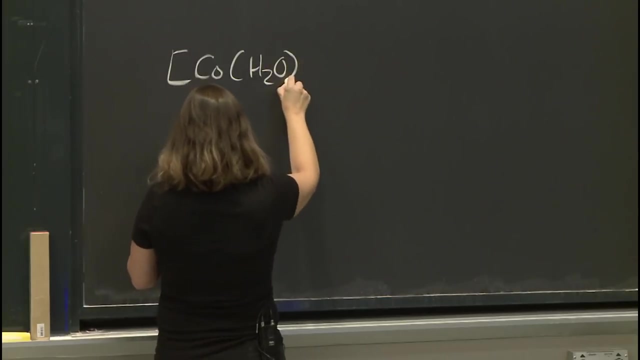 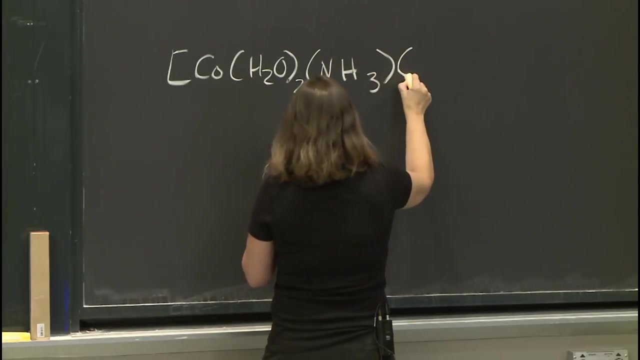 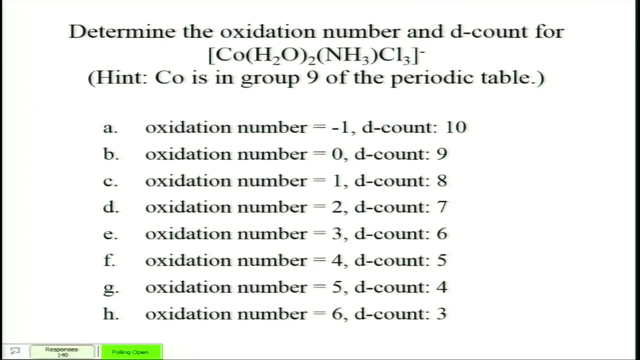 10.. So that is a d-10 system. All right, We'll do one more over here, And the next one is a clicker question. It gives me time to write 0.. 1, 0 is going to be 1.. 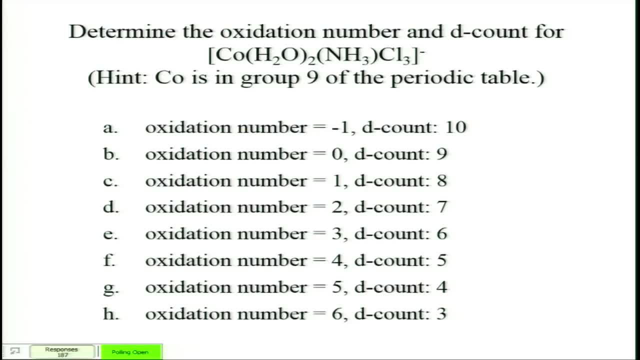 Let's just figure out what that number is. Yeah, it's going to be 1.. All right, let's just do 10 more seconds. Let's see if we can do 10 more. Oh, we're good, That should be good. 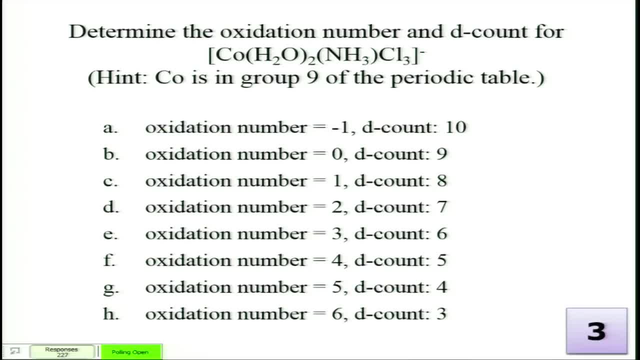 OK, so we're going to do one more of these. Let's just figure out what that number is. 0 is going to be 1.. Yeah, it's going to be 1.. Yeah, it's going to be 1.. 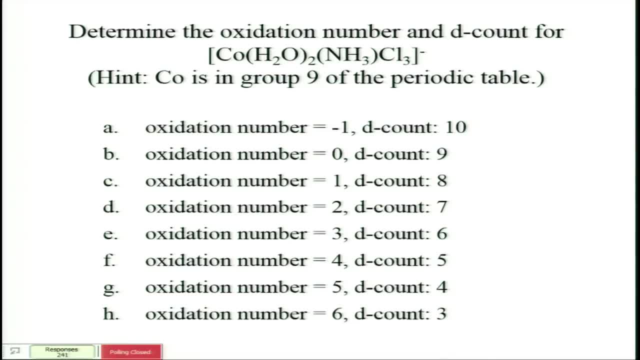 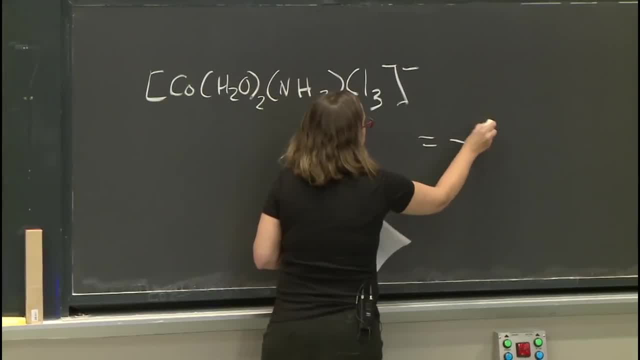 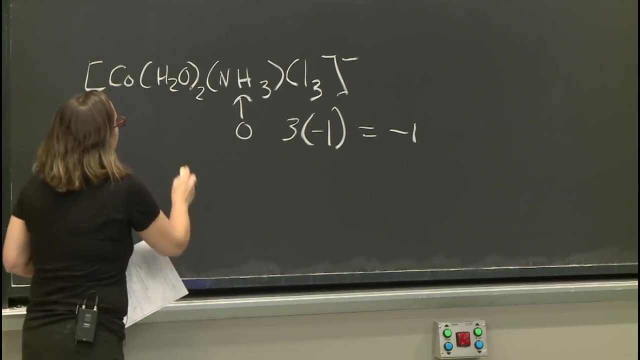 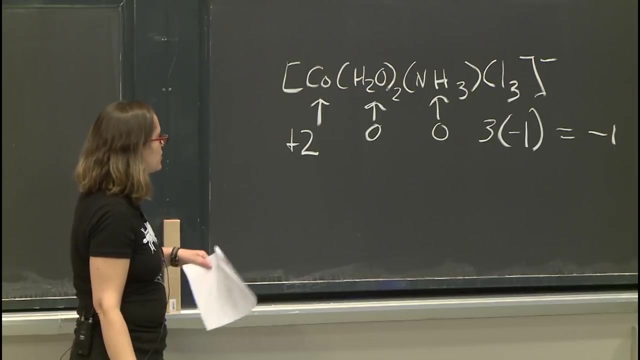 Let's just figure out the number of the different times: Yep. so here our overall charge is minus 1, we have: the chlorines are minus 1, NH3 is 0, water is 0, so this has to be plus 2, because plus 2 minus 3 is minus 1, we. 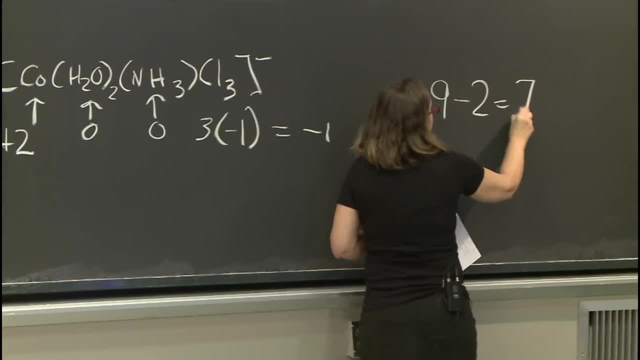 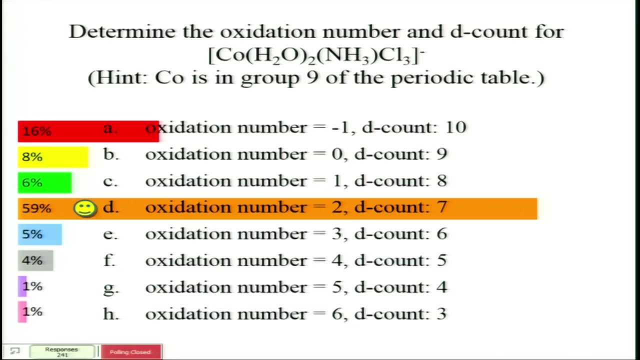 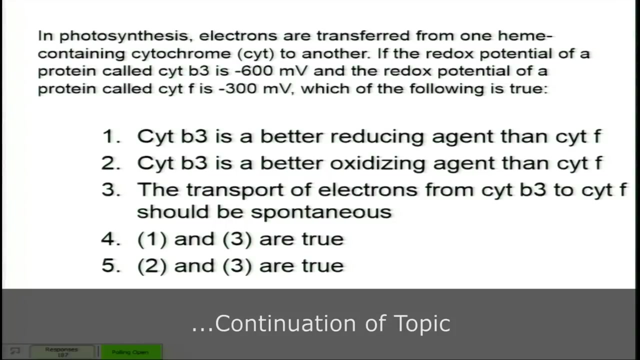 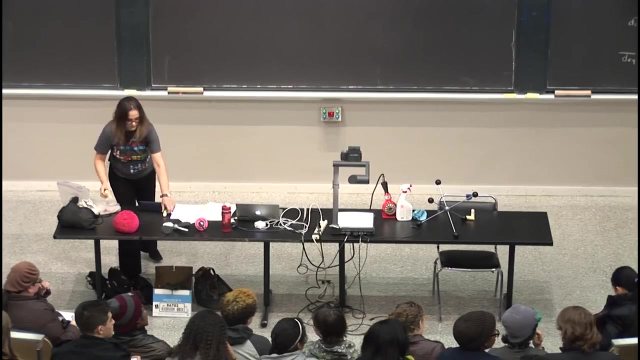 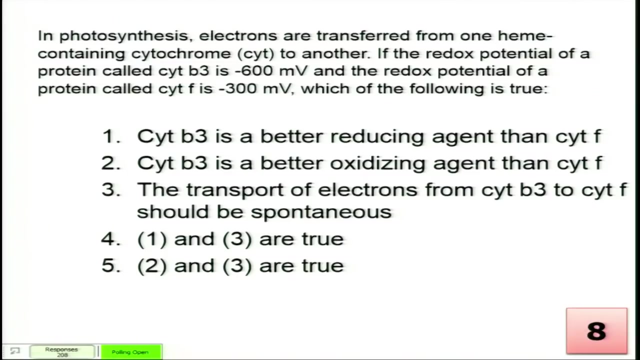 have 9 minus 2 is 7, so it's a D7 system. All right, so Wednesday d orbitals. I cannot wait. Yes, all right, 10 seconds. Okay, does someone want to tell me why that's the right answer? 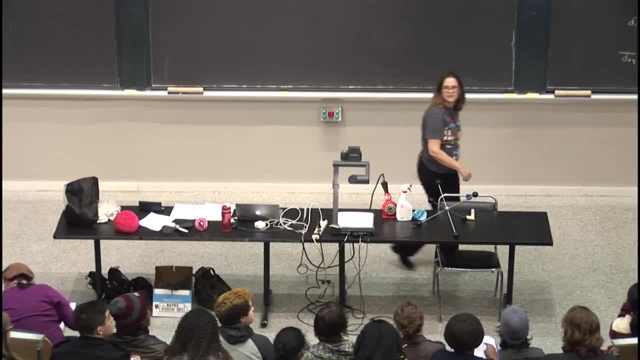 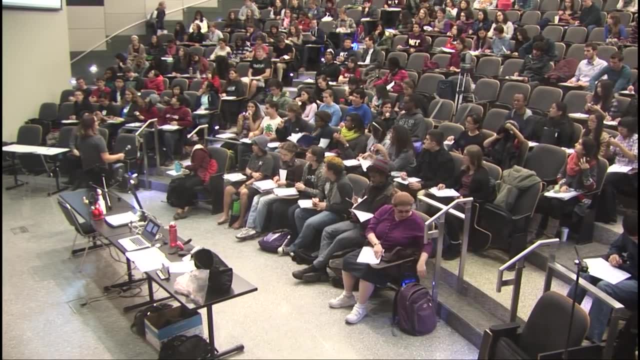 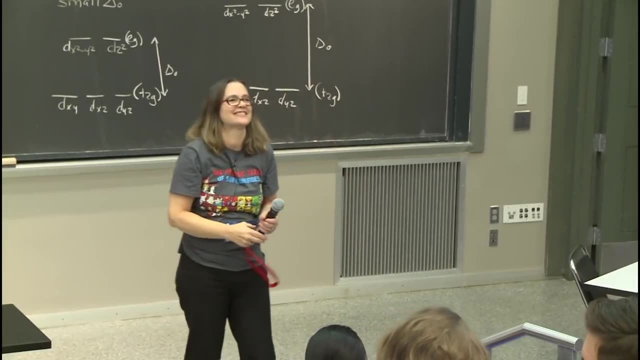 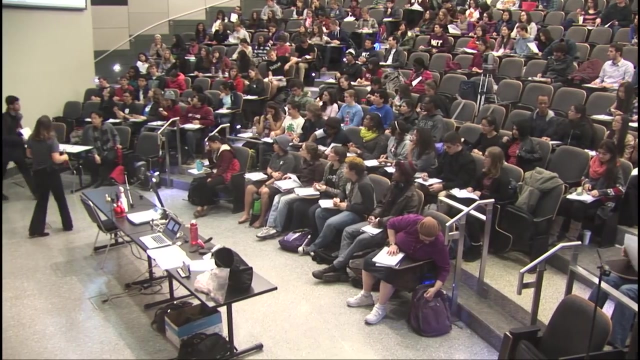 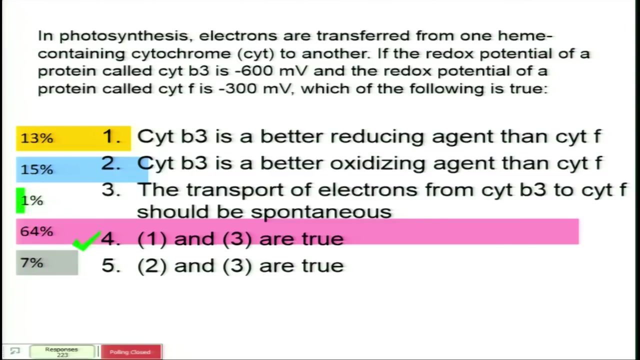 Okay, anybody We got. we got a nice dangly thing for your keys or ID. no, All right. so here we're thinking about whether things are better reducing agents or better oxidizing agents, and here we're given two different redox potentials, minus 600 and 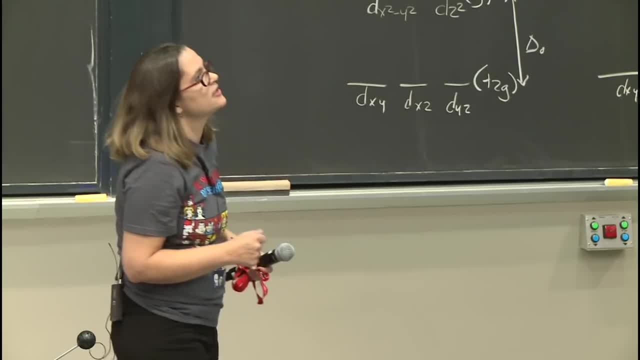 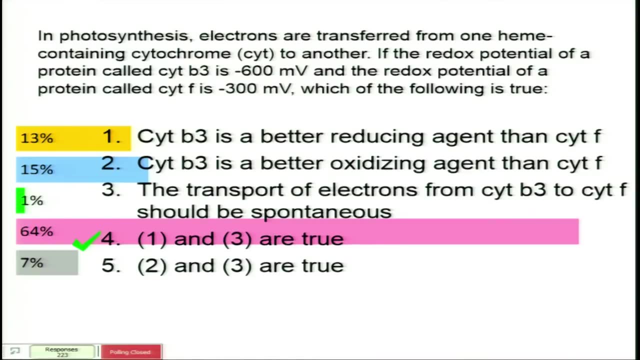 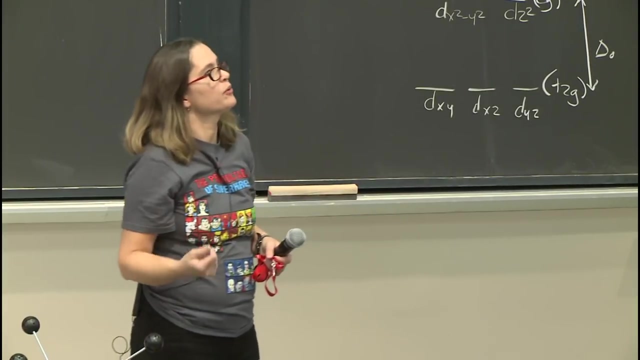 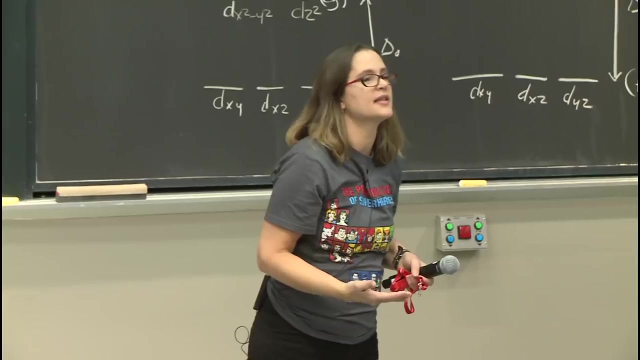 minus 300.. So the one that is going to be the lower number is going to be better at reducing other things. it wants to be oxidized itself And then we can think about whether it's a favorable process in terms of whether the thing that likes to reduce is actually doing the reducing that's going to make it a spontaneous. 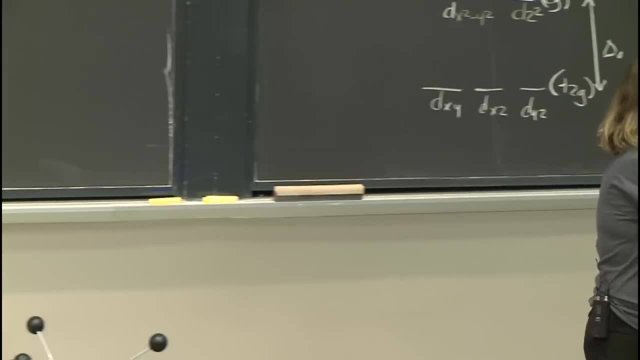 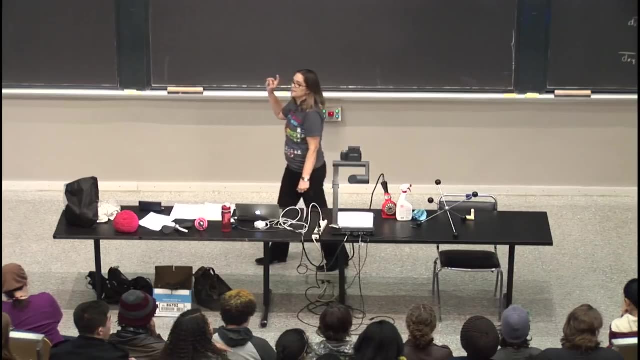 process. All right, so these are the kinds of questions for the oxidation reduction unit. So we're going to be looking at two units that we just finished, and this will be on exam 4, which, amazingly, we just finished an exam and there's another one. 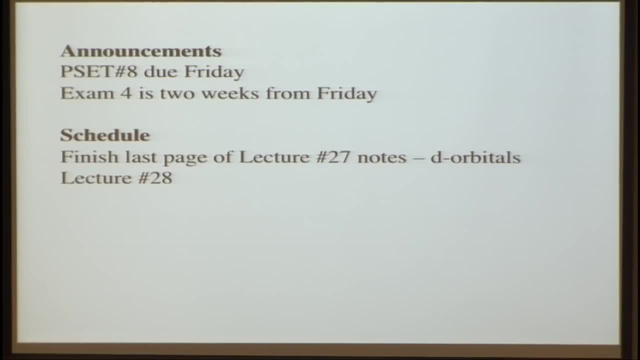 So exam 4 is 2 weeks from today, All right, or from Friday, sorry, 2 weeks from Friday, All right. so today we're going to continue with this unit on transition metals. the next exam is going to have oxidation reduction and transition metals and a little bit of. 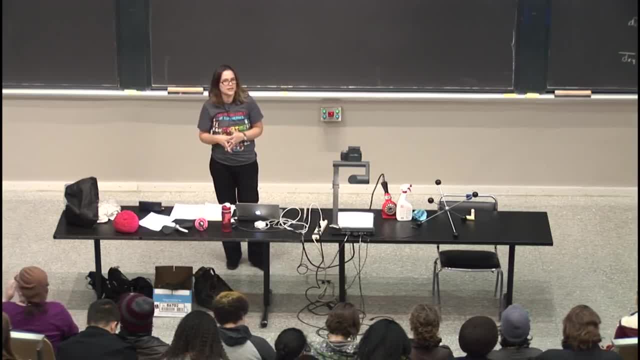 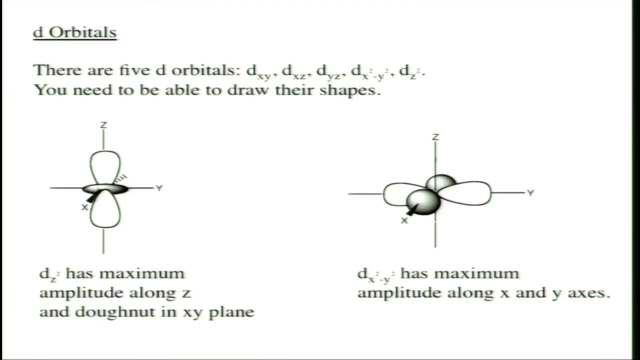 kinetics. Kinetics is our last unit, so we're getting very close to the end of the semester. All right, so that's the first unit. So we're finishing up the handout from last time. Again, we're back to the periodic table. 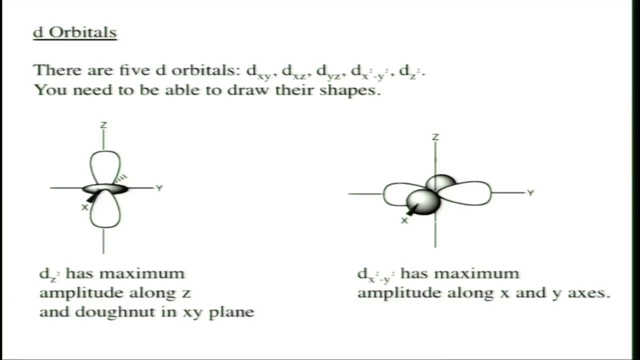 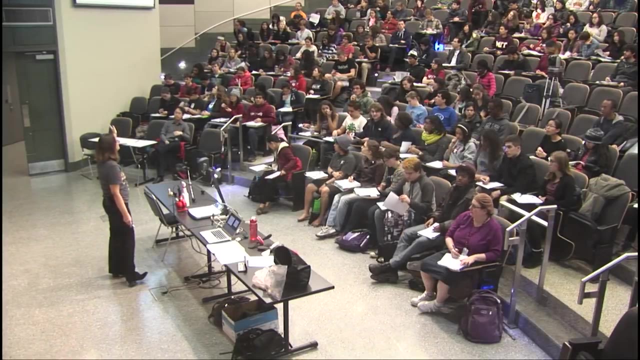 We're thinking about transition metals, We're thinking about that middle part of the periodic table, And so we're thinking about d orbitals. So there are five d orbitals. How many s orbitals are there? One? How many p orbitals are there? 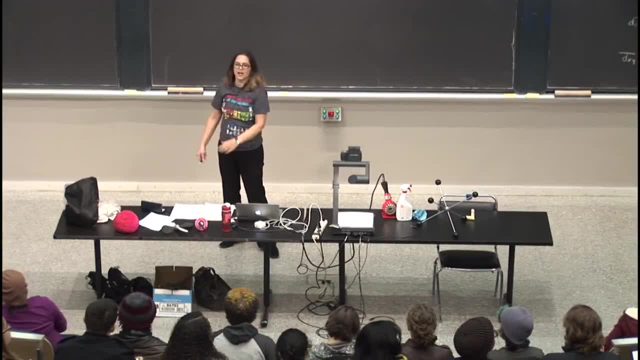 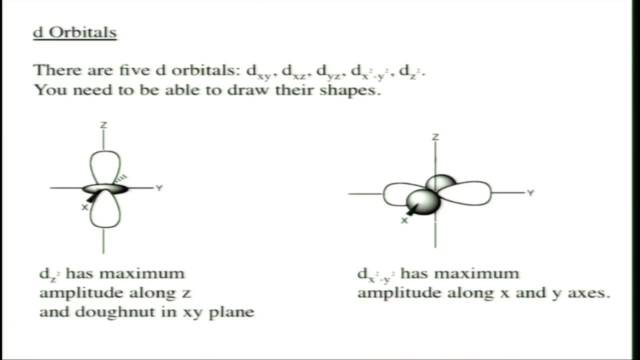 Three And so d orbitals have five, And we're not going to talk about really anything beyond d orbitals in this class And frankly not very many people do. But d orbitals are amazing so we have to fit them in. 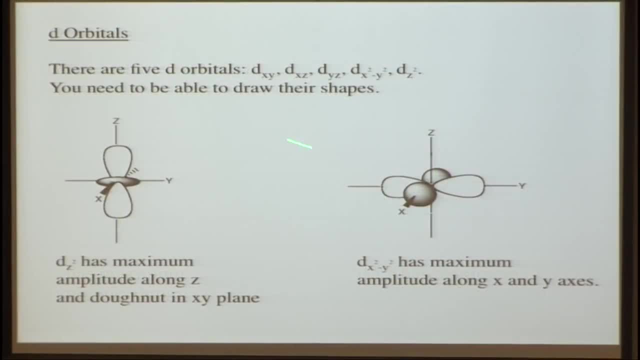 So there are five d orbitals And they're up here And you need to be able to draw their shapes, And the bar for drawing the shapes is actually pretty low. So these are my drawings that I made, And so you can probably do just about as well. 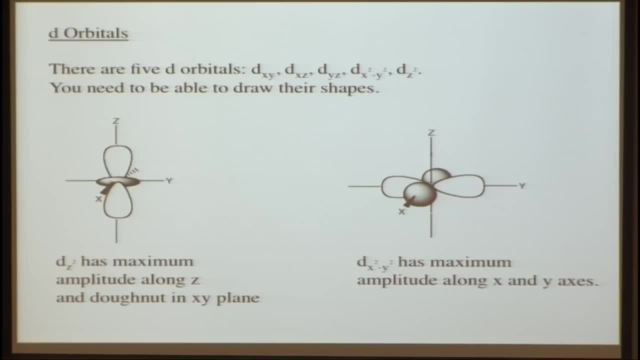 All right, so the one that has the most unusual shape is the dz squared, And so it has its maximum amplitude along the z-axis, And for this unit, our z-axis is always going to be up and down. here y is in the plane of the screen. 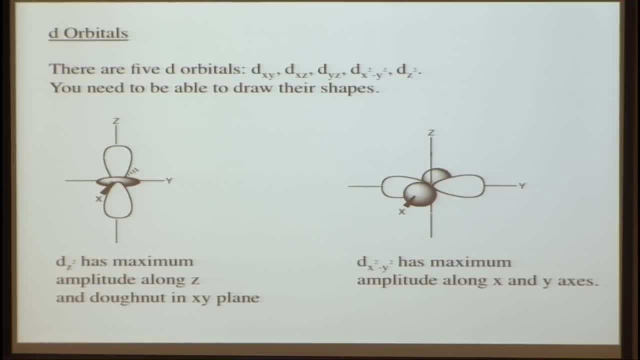 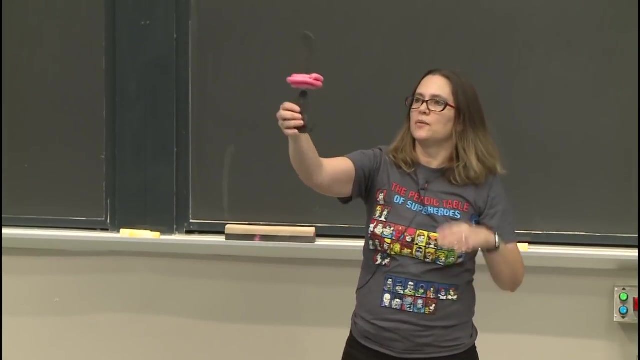 And x is coming out towards you and also going into the screen, And so dz squared is its maximum amplitude along z, And it also has a donut, OK, In the xy plane, And so I also brought a little model of this. 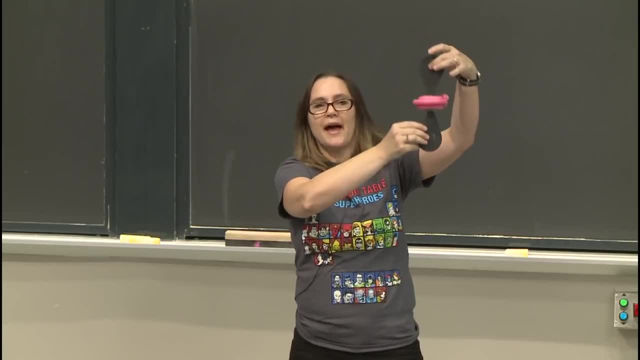 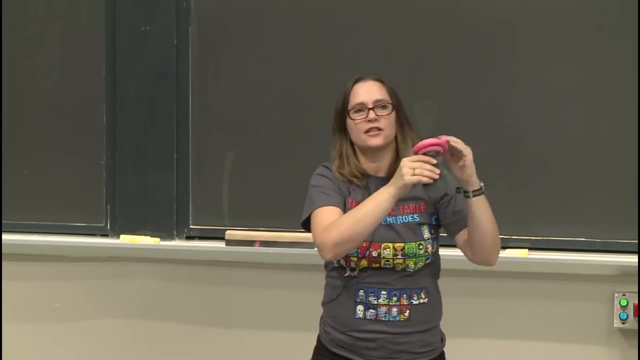 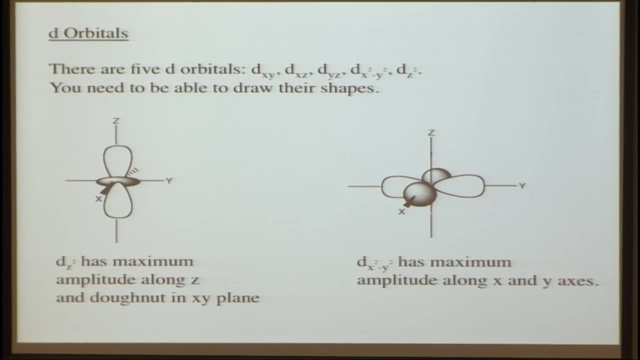 So here's dz squared. We have a maximum amplitude along the z-axis up and down, And we have our little donut in our xy plane. So then we have dx squared minus y squared, which has maximum amplitude along x and along y. 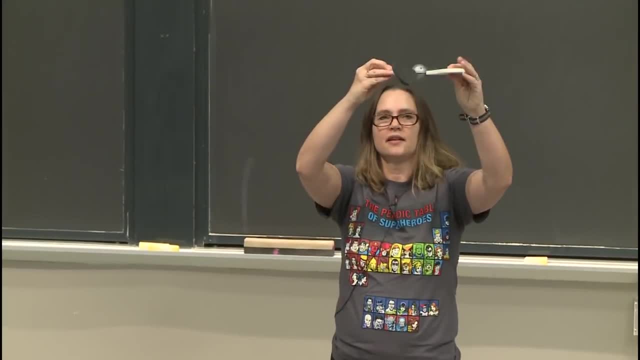 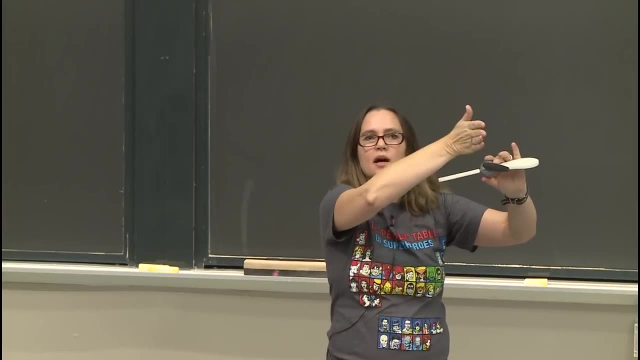 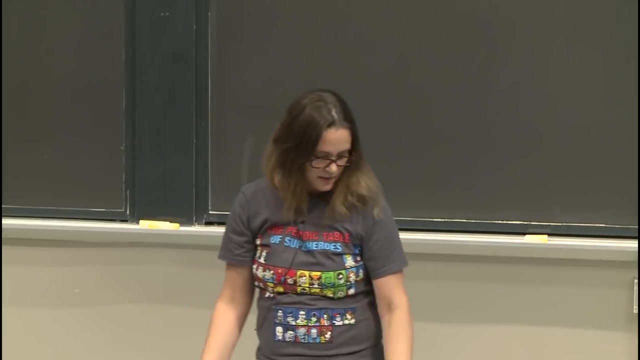 And that Would look like this. So we have our maximum amplitudes that are right on axis. So if this is y-axis and x is coming out towards you, those orbitals are pointing right along that coordinate frame. The other three orbitals look a little bit like dx squared. 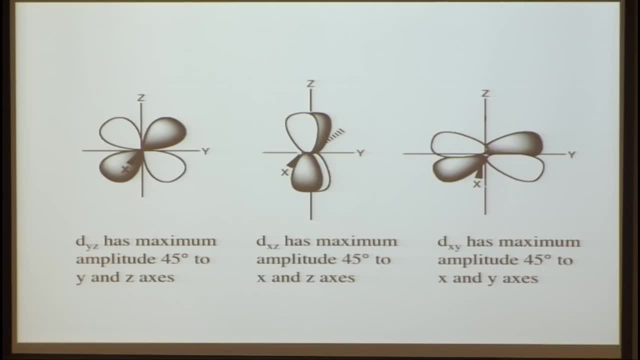 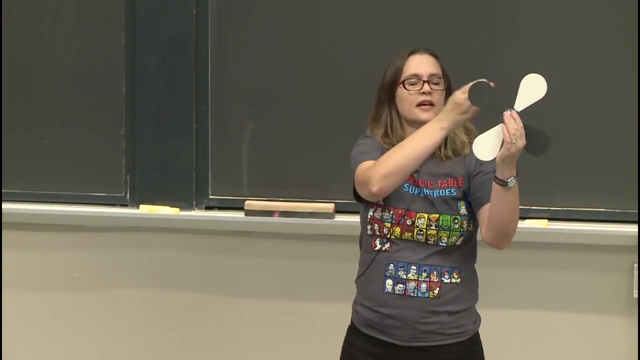 minus y squared. But they're not on axis, They're off axis, They're in between the axes. So we have dyz. It has its maximum amplitude 45 degrees off of the y and the z-axis. So if this is z-axis, here there's. 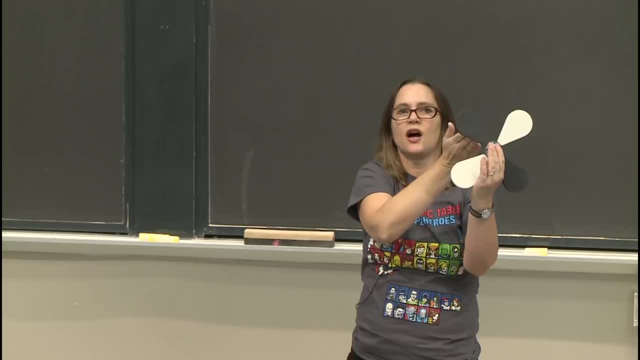 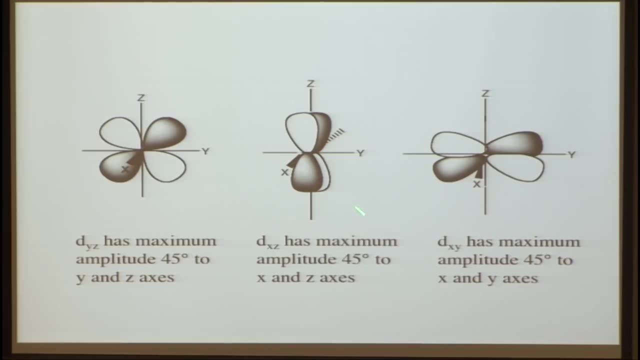 no maximum amplitude along here. It's 45 degrees off. So it's right in the middle between the z and the y. So dxz has its maximum amplitude along, or 45 degrees between x and z. So that would be pointing the other way. 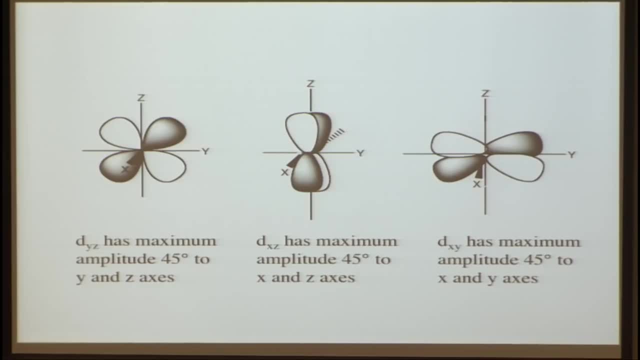 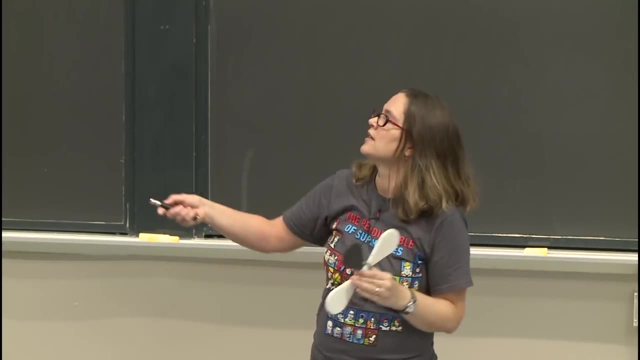 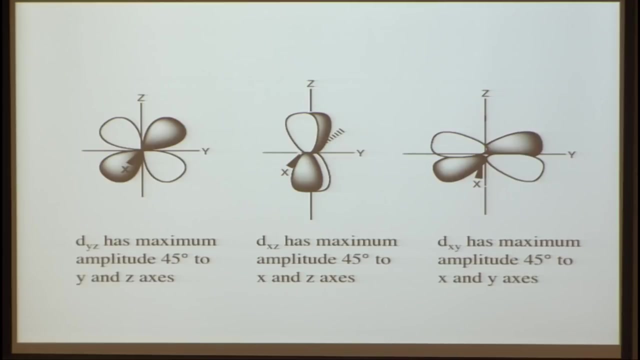 And so I tried to draw this, keeping the reference frame the same. It's a little hard to see the orbitals, but it would be kind of this: So we rotate that around, And so that's what that would look like. And then dxy- we have maximum amplitude: 45 degrees. 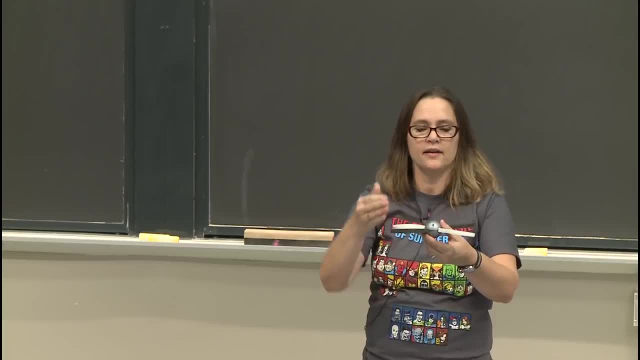 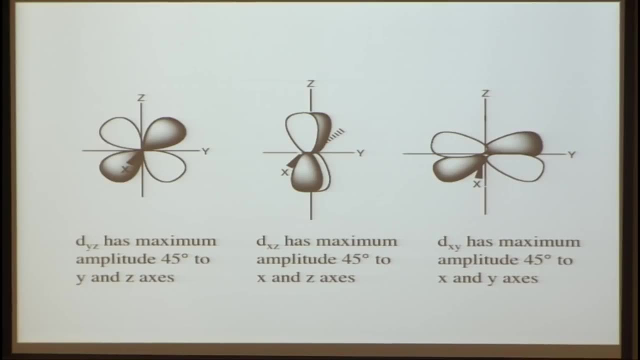 in between the x and the y, So x coming out, y in the plane, And so this is again a little bit hard to draw. If I drew it absolutely perfectly and not tilted at all, you kind of wouldn't see anything. 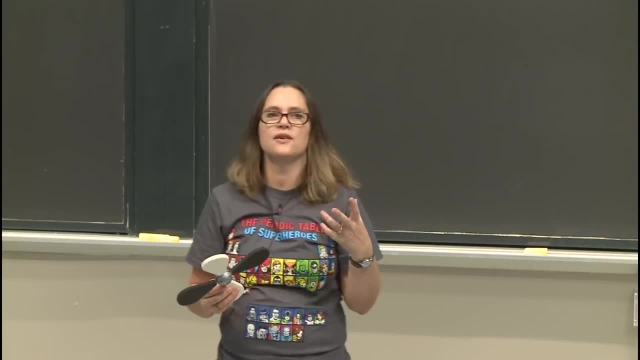 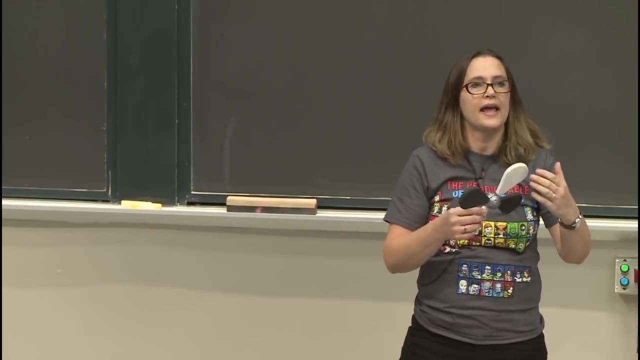 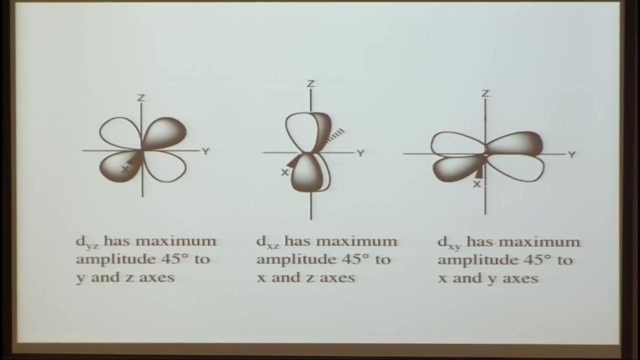 But that's what that would look like. So again, the names of this. it tells you about the relationship between that orbital, that maximum amplitude and the axis that we have defined. So this is very important to know that these guys are in between the axes. 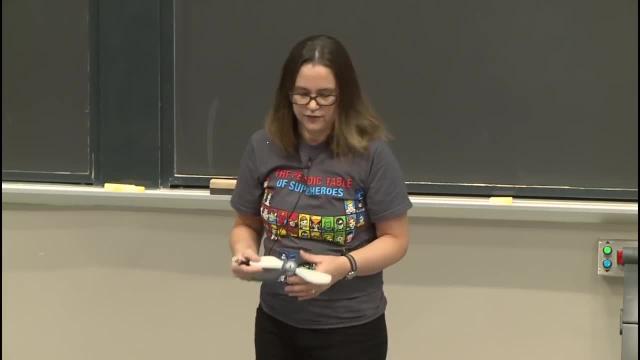 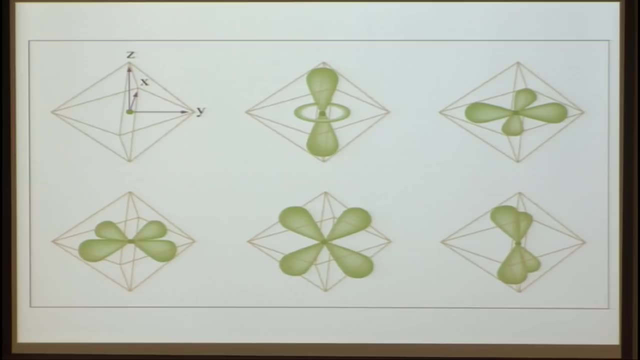 right in the middle, 45 degrees, And you'll see why in a few minutes, why that's important. OK, so just to practice, here are some slightly better pictures of the orbitals, And this is the coordinate frame over here. 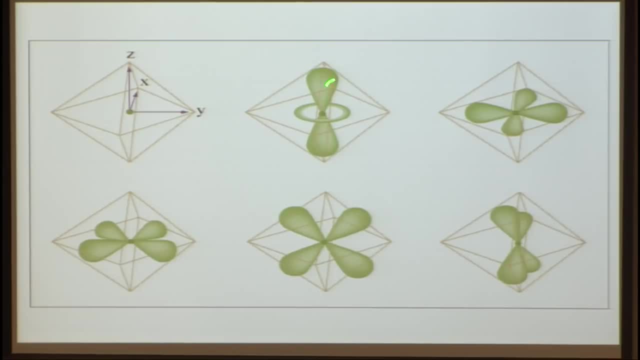 And now we have the orbitals inside that. So again, z is going up, y is in the plane of the screen and x is going back and also coming out toward us. So which is this d orbital? You can just look at it. 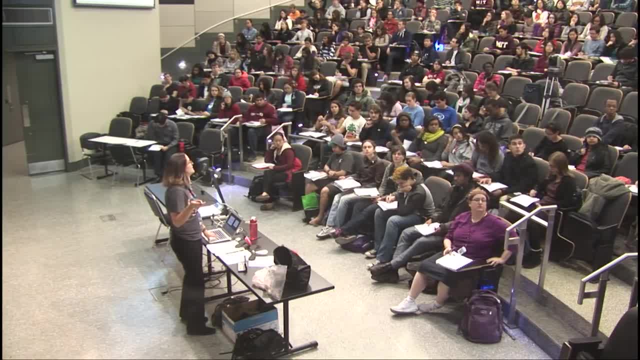 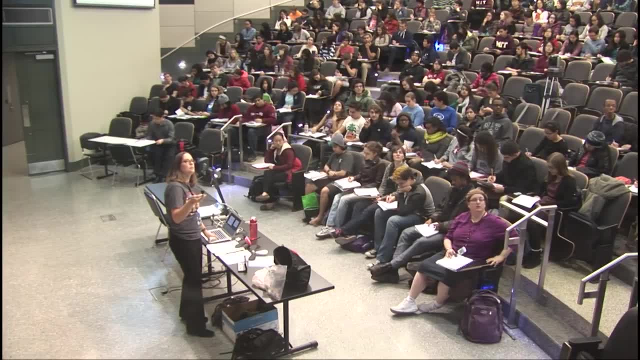 You can just yell it out: Yeah, that's easy to remember. That's the unique-looking one. What about this one? Think about this First. think about the plane. So it's the xy plane, and then is it on or off axis? 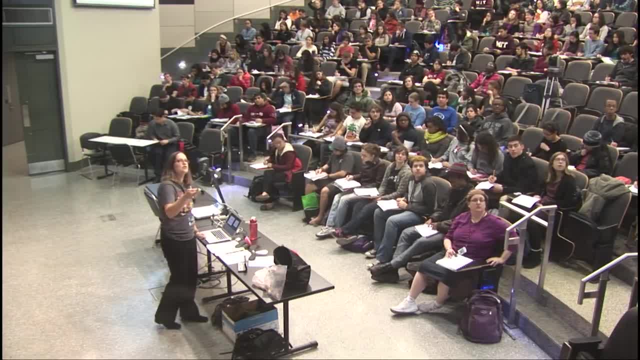 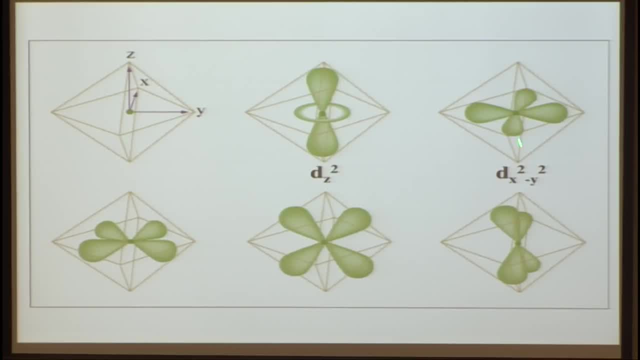 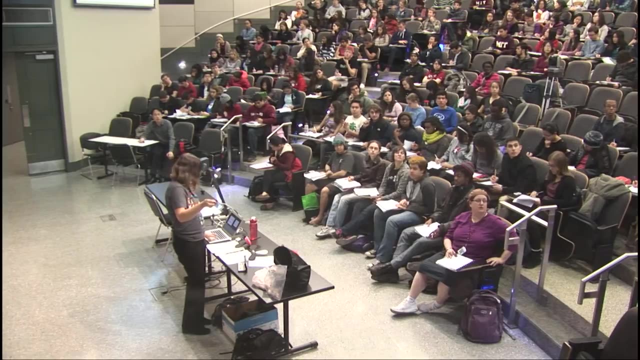 So which one is this? Yeah, so this one is on axis. You can see the maximum amplitude of the orbital pointing right along those axes. So it's right in the corners of that square there. What about this one down here? Yeah, so that would be dxy. 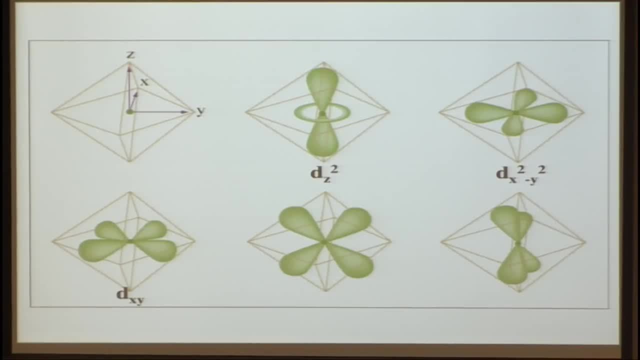 So it's in the xy plane, but it's 45 degrees off the axes, So it's in between the axes here. And what about that one, Right? so we have it's along both z and y here, And then this last one, which is drawn to kind of come out. 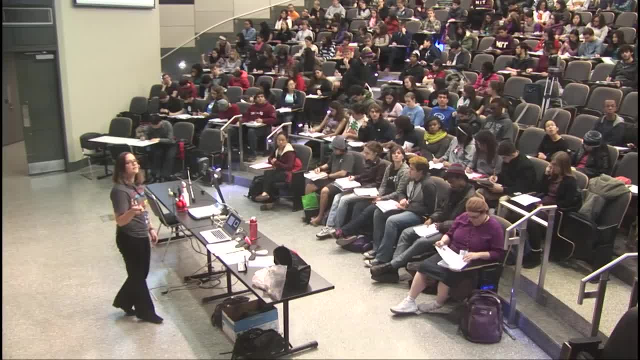 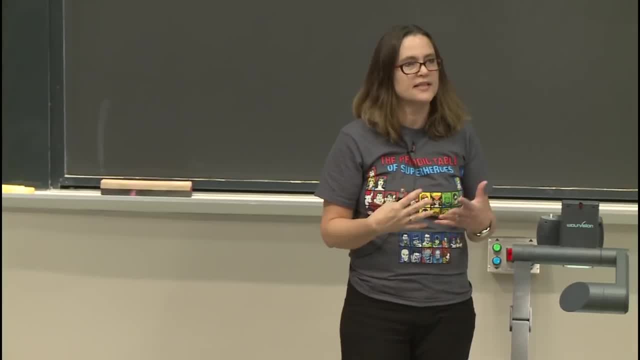 toward you. so that is along x as well. OK, So that's dxz and it's going up along z. So you can look at the coordinate frame, which we'll try to keep consistent, and figure out whether ask yourself: is it on axis or off axis? 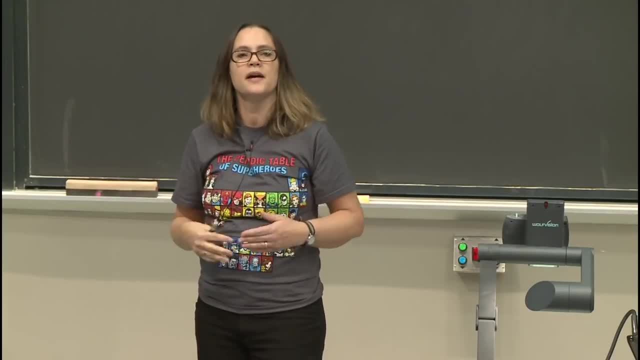 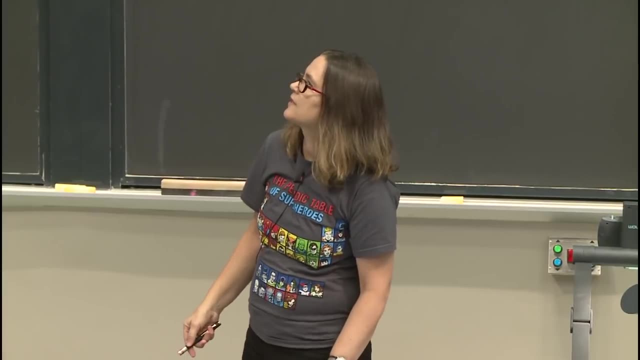 and which plane is it in, And that will allow you to name them and also to draw them. So just to kind of give you more of a three-dimensional sense, there's these little movies that I'll show you now And so you can get a better sense of that awesome donut. 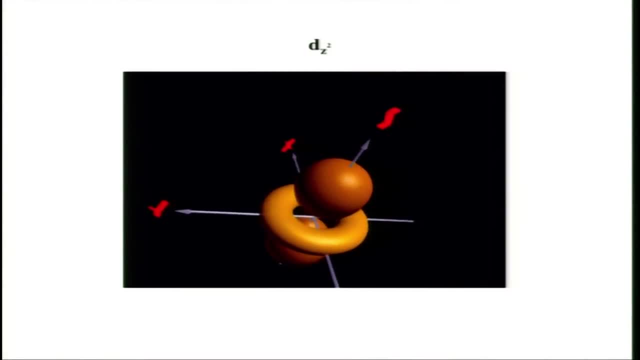 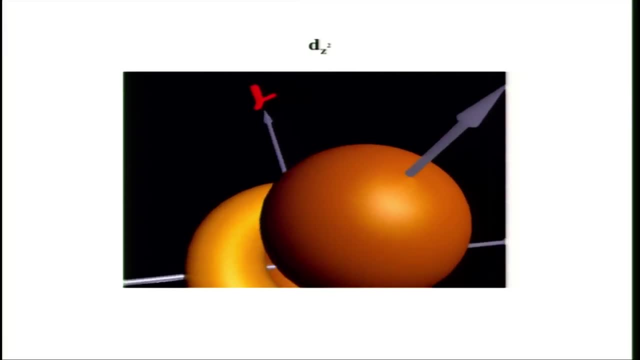 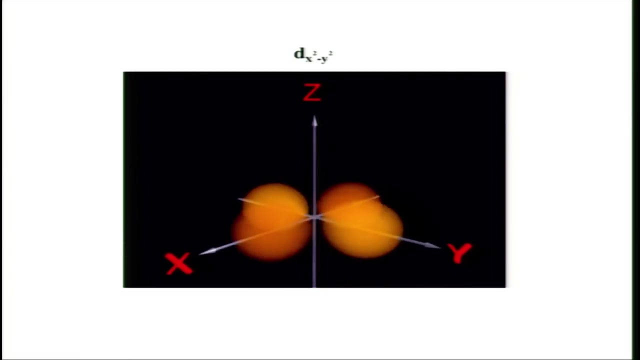 It's going to make you hungry. They even colored it. They colored it like a really nice original donut that you would get at Dunkin' Donuts. So the donut is in the xy plane and these other lobes are along z. 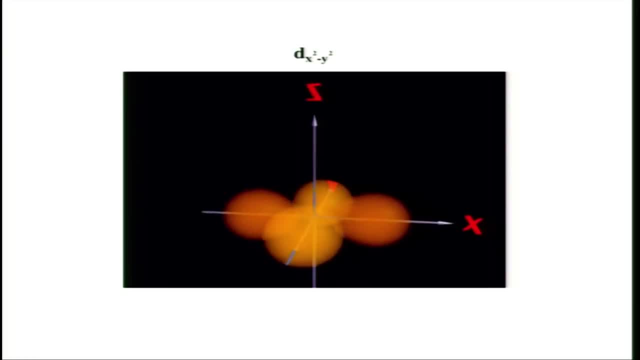 So now we have dx squared minus y squared and you can see that the maximum amplitudes again are along the axes Key. they're along the axes here. I don't know why it comes out toward you and it wrote I didn't yeah. 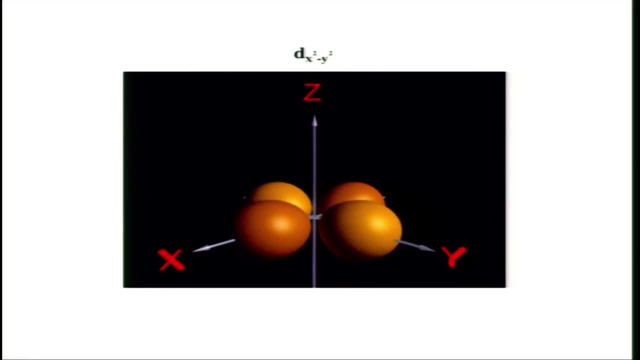 But it gives you a good three-dimensional sense of this. All right, so dxy, now again in the xy plane, But instead of being on axis, it's 45 degrees off axis. You can see, I think in this really nicely. 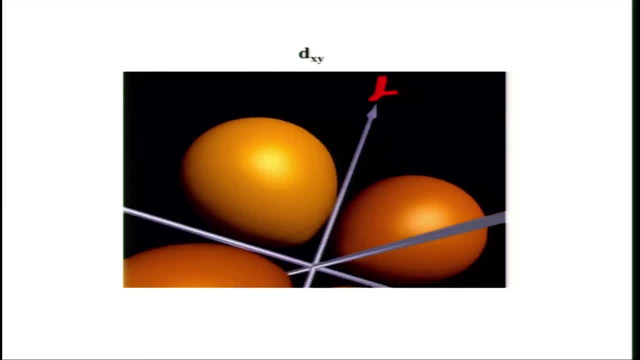 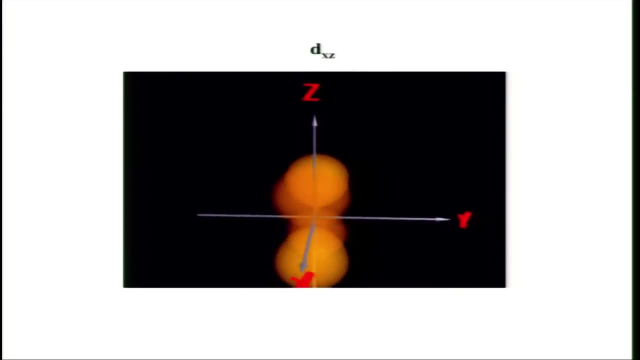 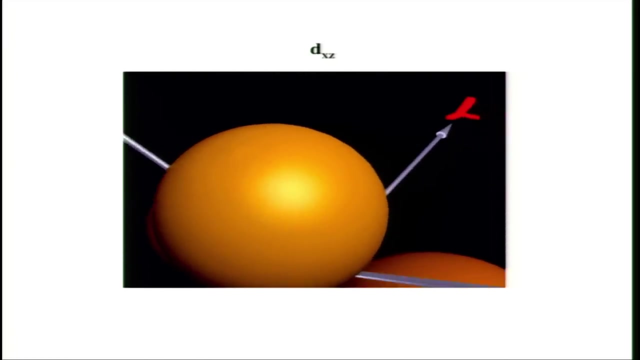 it's right between the axes, but it's not touching them. The axes sort of separate these orbitals. And then we have xy. So now we're going up along the z-axis and in the x-plane. And here it comes at you again: 45 degrees in between z and x.